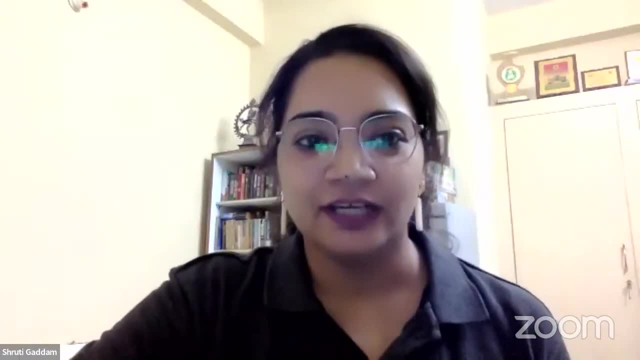 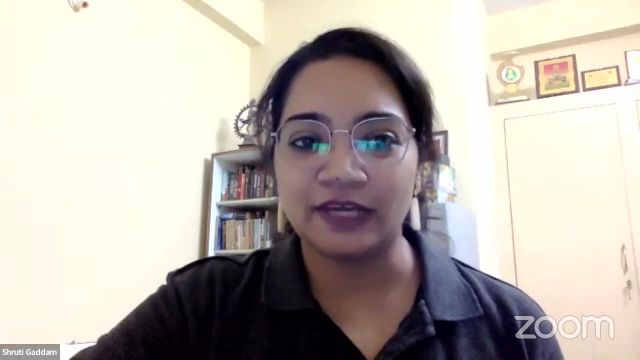 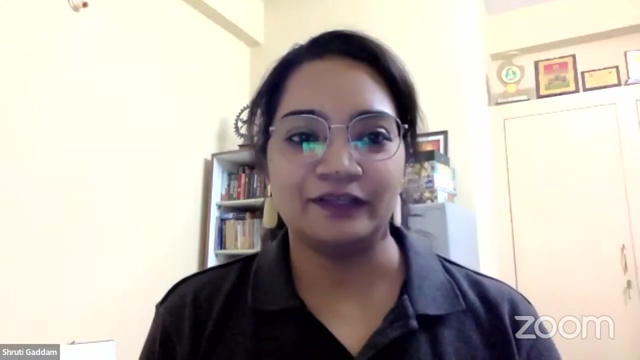 He's a specialist currently with NTI Mindtree and he comes with a lot of experience in the data sciences domain. Today's topic is very interesting: How do you extract information from NLP? So I will leave it at that. I will let Sarveshwaran you know. take us dive. 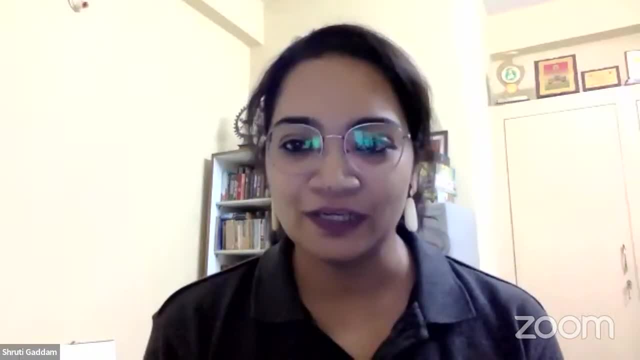 deeper into this topic and help us understand what it is all about, Looking forward to a very exciting session. Sarveshwaran, thank you so much for joining us. I hope you have a very exciting session. Sarveshwaran, over to you please. 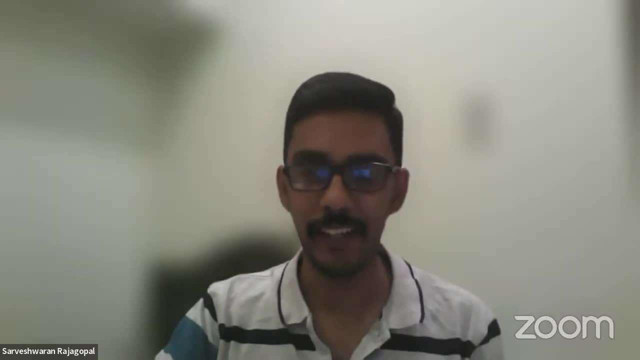 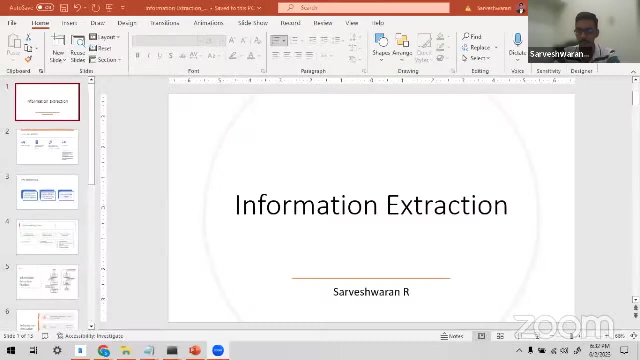 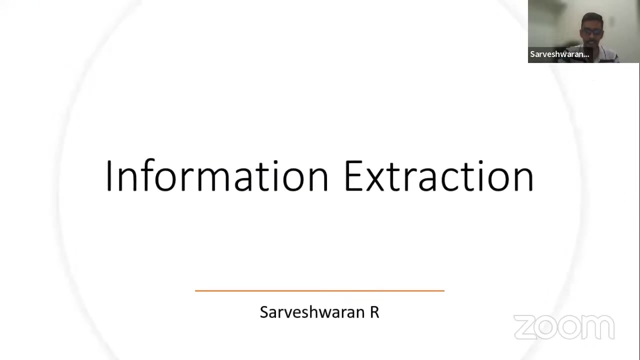 Sure Thanks. Thanks, Jyothi, And good evening folks. I welcome you all to the interesting session on the information extraction using NLP techniques. Okay, let me share my screen, All right? So okay, so what is information extraction? So any thoughts? So how do you? 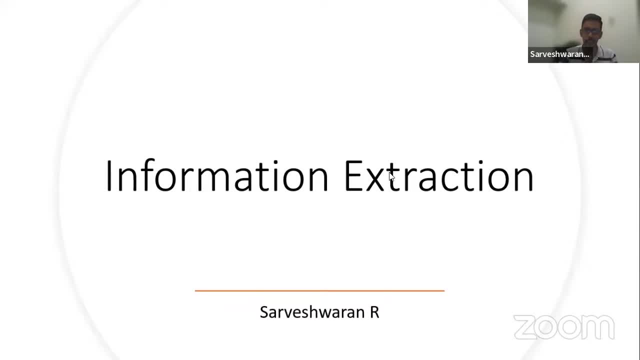 put in chat. Okay, So so here the information extraction is a white box. So after the rise of the GPT models and all these things, So the text is being shown more importance in the current world. So how a text processing is done, How can we make an informed decision with all? 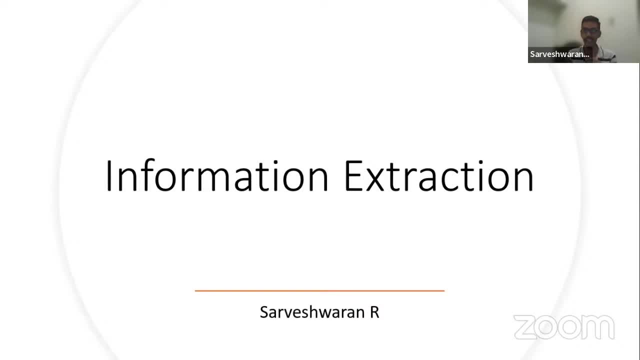 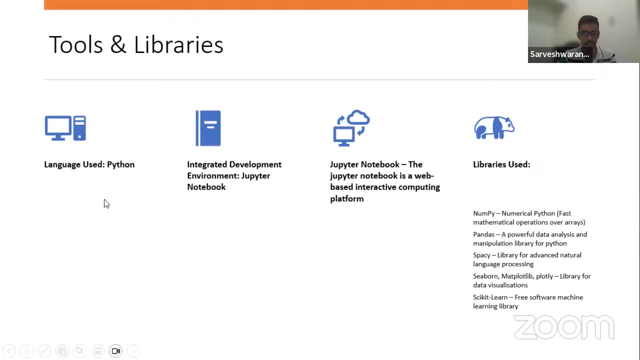 the documents? How can we extract the entities? There are various different applications to information extraction, So let's see what is an information extraction and let's go through it. So here, so the current the tools that we are going to use is the Python working notebook. 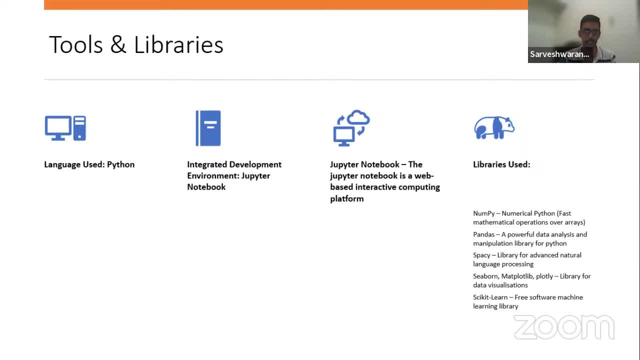 We can also understand what is a part of speech, what is an information extraction using spacing, and I'm using Jupyter Notebook for the today's session and I've also taken an example, the real-time example, the resume shortlisting using NLP. 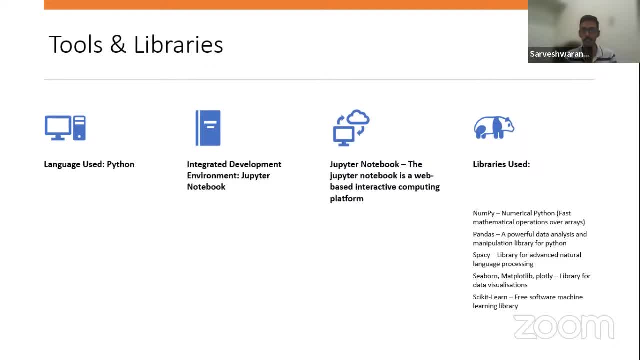 I've also showcased how and resume can be shortlisted using the NER techniques. So here I'm going to use NumPy, Pandas, Pacey and for clotting all the C Bon, ManclotLib and SkyKit Lab. 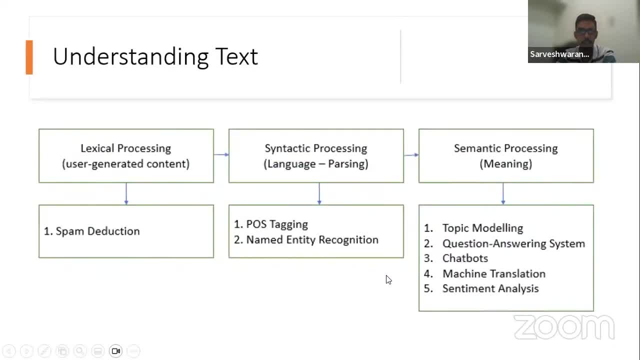 So before here. so let's understand text. So what is a text? So for us it's: the text is coming from a document. So what is a text for a mission? So what are they? So what are they? different use cases. that is revolving around the text, So the text can be the text processing. 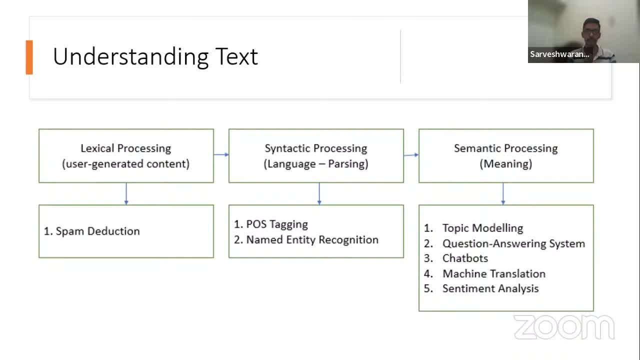 can be taken into three different processes: lexical processing, syntactic processing, semantic process. So what is a lexical process? So, firstly, we convert the text into words and, depending on all your application needs, So they are converted into either sentences: 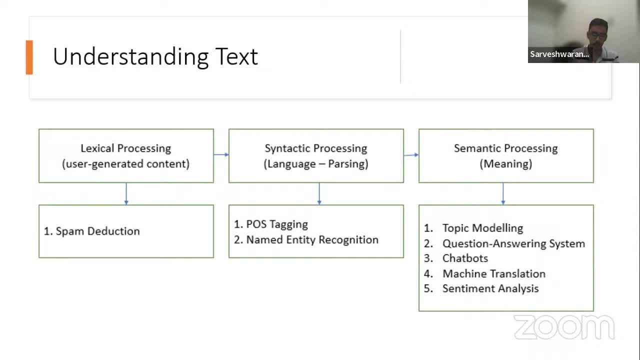 paragraphs as well. So not only converting to words, it can be converted into sentences and paragraphs. Say, for example, you receive an email. it has a word such as lottery prize or luck, So then the email is represented by these words. it is more likely that email 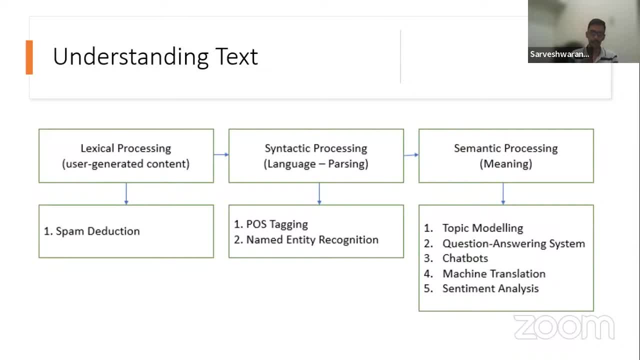 is going to be in spam email. So we have a lot of other words. we do not want the inbox to be spam. So the first use case, we are going to take a specific word and we are going to look up for that word. 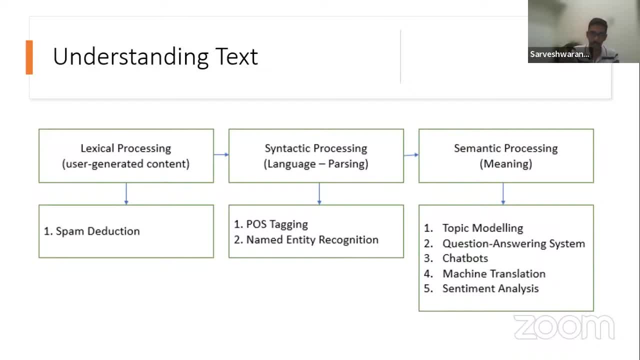 if there is that, if that email contains the word lottery, the prize or luck, something In general, the group of words that is contained in a sentence, and it gives an idea of what the difference is between the two. So the group of words that is contained in a sentence. 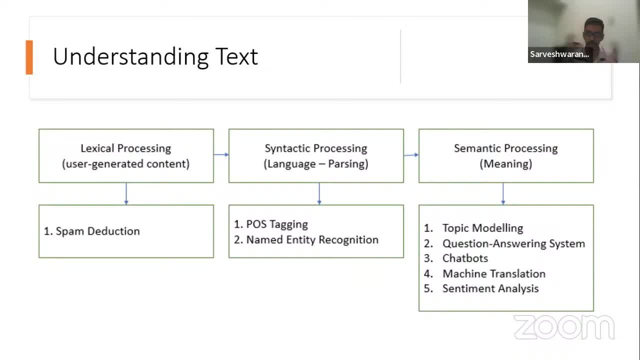 that email is or what that sentence is. We are breaking the email into smaller parts, into sentences or in paragraphs or in words. So here it goes. it does not look for the syntax, it just looks for the word. the word is present. that email is classified as spam. 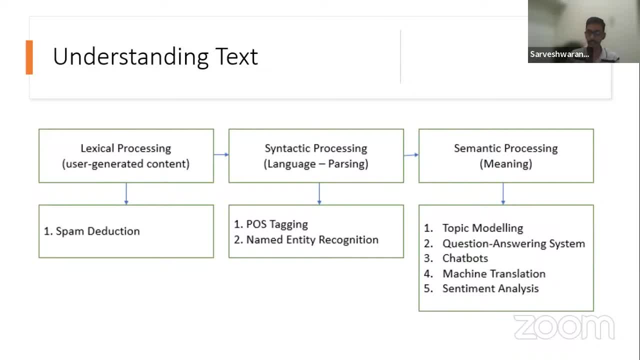 The classical use case, very classical use case. Now, what is the advancement to it? We do a synthetic processing From lexical analysis. we do a synthetic processing. So the lexical analysis or the lexical processing, what is, on synthetic processing, more advantage? 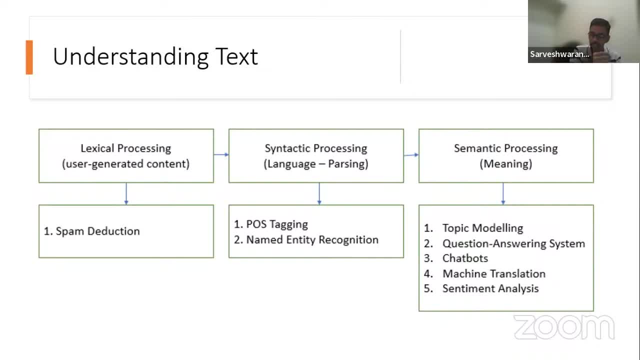 than lexical process. Here in synthetic processing we extract the meaning from the sentence by using the syntax of its word, syntax of that sentence. How do we extract the syntax? I extract the sentence using an part of speech tag- POS tag, very famous. What is in part? 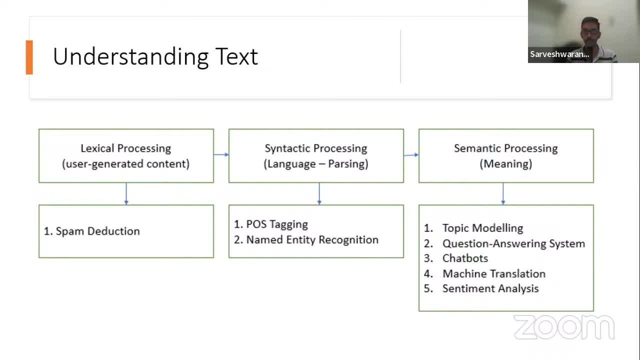 of speech, Noun, verb, adjective, sentence. So we extract the meaning from the sentence. One of them is adjective ster, relative adjective determiner, So adverb. There are so many different part of speech. Another one is the name entity recognition, very famous use case. 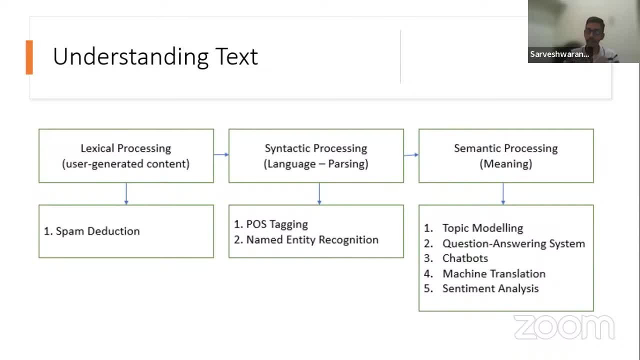 nowadays. So if I have number of documents in it, So there are number of. there are a lot of noise that is present in it, The unwanted words. I need to extract only the useful information from all the documents or anything. 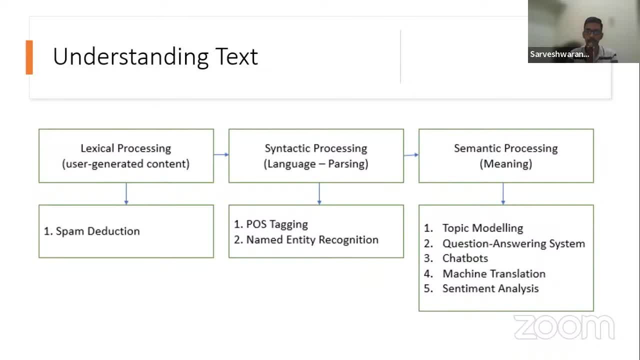 in a book or in a set of text. How do we do that? I extract using a name entity recognizer. By understanding the part of speech, the name entity recognition is done. I'll also showcase an example where we have in real time. 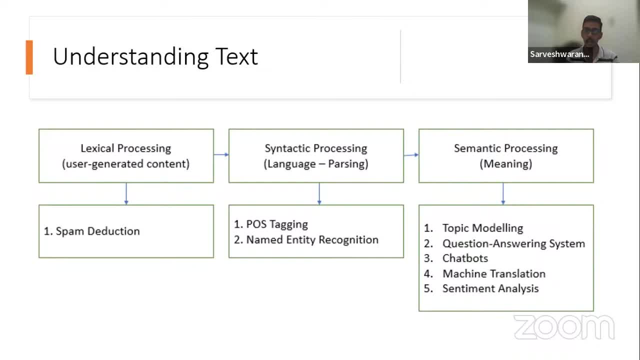 we have done a resume shortlisting using NLP right, How a named entity recognition has been used, and we have done a beautiful project around the syntactic processing right, The resume shortlisting using NLP, And the last step here is the semantic processing right. 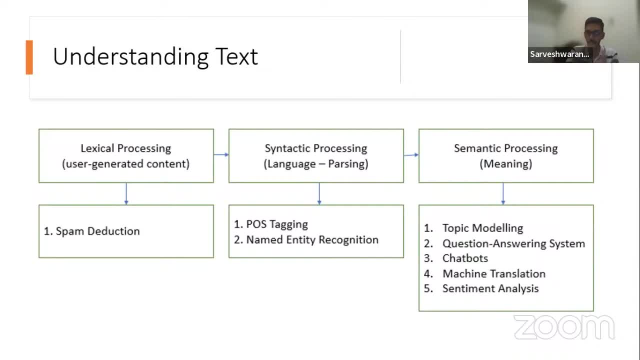 So here in the syntactic processing- sorry, the lexical processing, if I have an example- my cat ate its third meal And there is another sentence, my third cat ate its meal. Syntactically these are two different sentences. 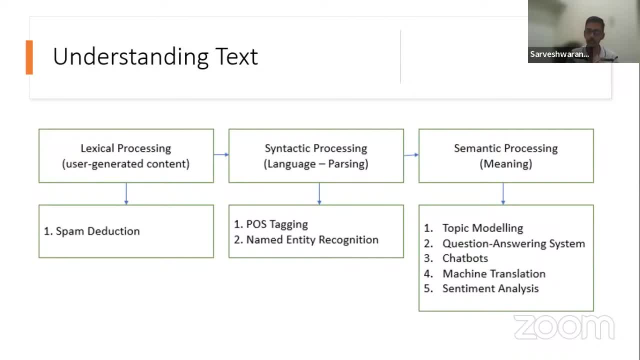 If I had to use a lexical, I would use a lexical processing. It doesn't know, the cat ate its third meal or my third cat ate its meal. They both are same for lexical processing When I'm going to use in syntactic processing. 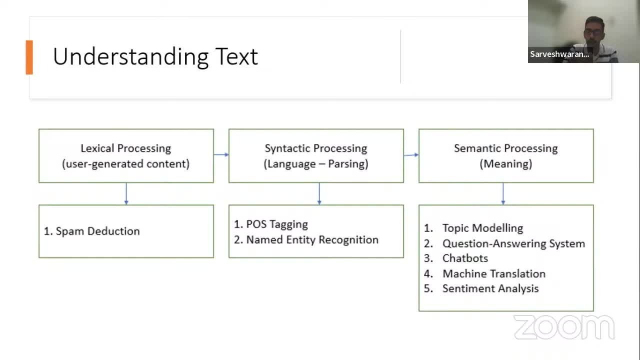 it knows what's in verb, it knows what's a noun, what is a noun phrase, So it can actually find the difference between the first sentence and the second sentence right. Ram thanked Shyam and the Shyam thanked Ram. 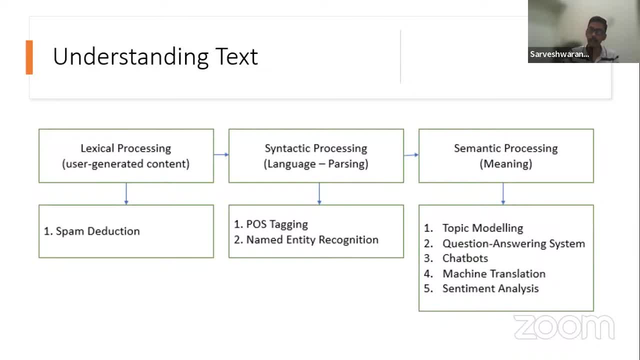 the classical example: Who thanked whom? Shyam thanked Ram and Ram thanked Shyam. These both are two different sentences. Lexical processing cannot distinguish between these two different sentences. If I'm going to use in syntactic processing, it knows the difference between who thanked who right. 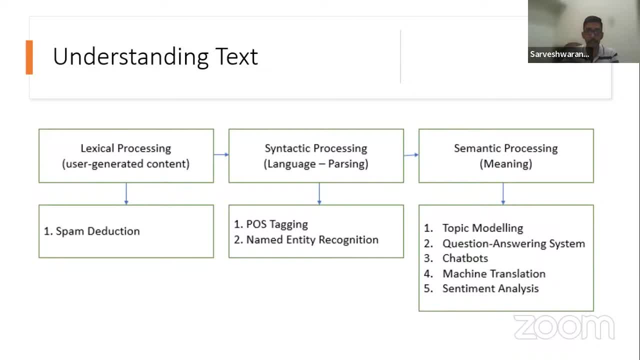 So it knows Shyam thanked Ram is different than Ram thanked Shyam. And the last is your semantic processing. It's more advanced. They're going to use it in a topic modeling the question answering system, the chat boards, the machine translation, the sentiment analysis. 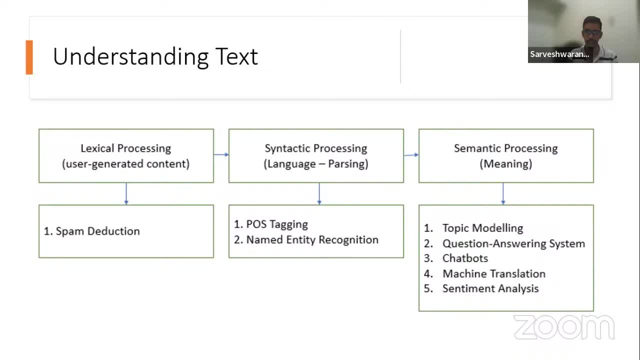 the applications keep on extending Semantic processing. Semantics is their most important trending topic now. What is a semantic right, Say, for example, someone asks who is the prime minister of India? right? So we are using an Alexa. We are using an Alexa. 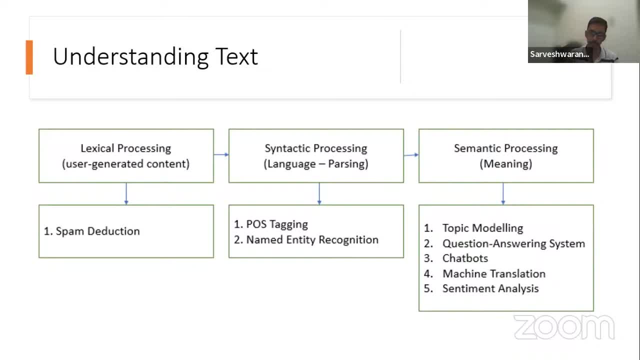 We are using in Siri right some voice assistant. You're asking who is prime minister of India right? It replies with Narendra Modi. So if you're going to twist the question- who is the PM of India Right? it should have the capacity or capability. 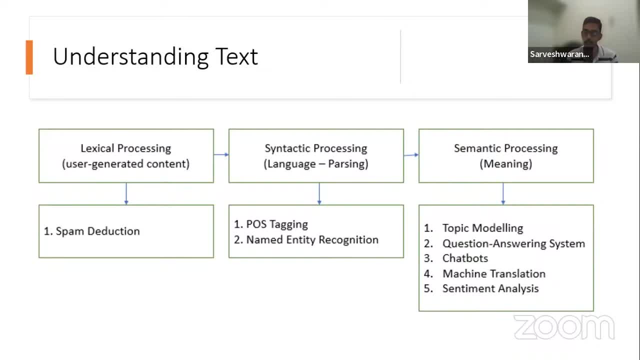 to understand that prime minister is equal to PM. How does it happen? We cannot create a lookup table for all the different centers or the acronyms, or the short forms. It should create a lookup table table on its own. How does it happen? It happens on the basis of your semantic processing. 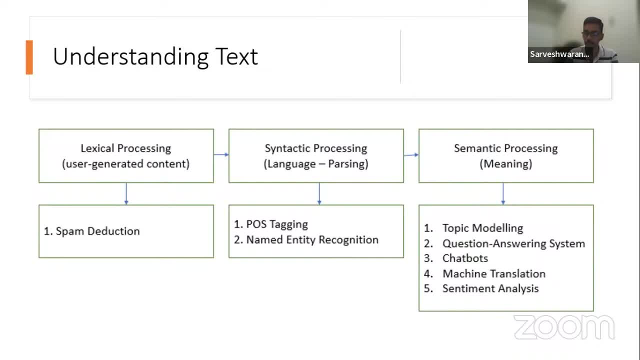 King and Queen, they all they are. there is again an example. So the Queen is simply the female version of the word King. If both these words are clubbed together, they are coming under an, the upper class, under the monarchy, or an kingdom. So the Queen is nothing. 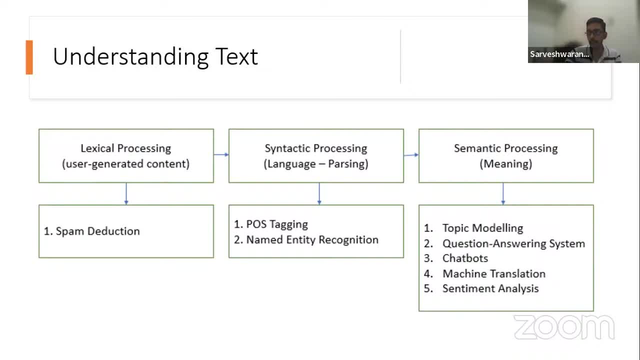 but a female version of the King. The female and the Queen or the King are not same, So it should understand the semantics present there. What is the meaning of that word is obtained using the semantic analysis. That is where your famous examples, like your mission. 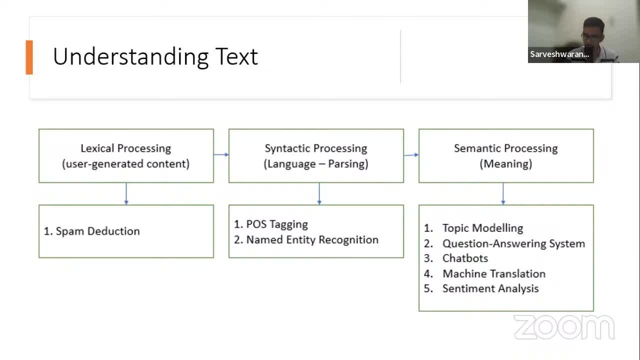 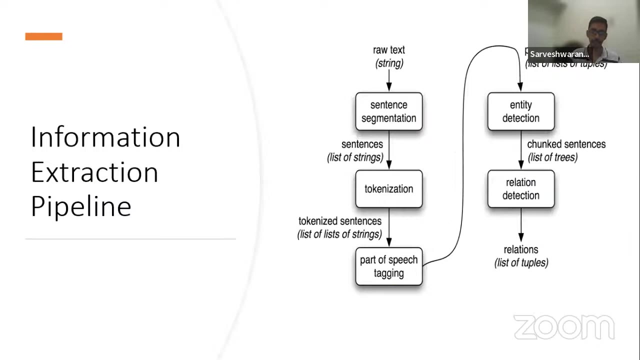 translations and the Charter of the World. So this, the scope of the lex, the semantics, is far advanced than your lexical processing and your synthetic processing. Let us go one step further. So what is an information extraction? So what is information extraction? And then we will get into the pipeline: What is an? 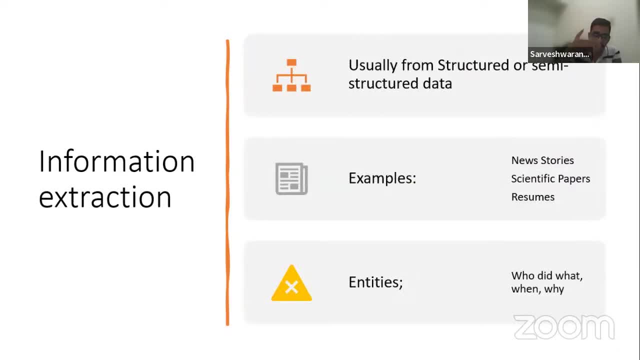 information extraction. So we extract the structured data from the unstructured data. To put it in very simple and in layman terms, we have an unstructured data or a semi-structured data, So we need to extract the useful or the important information, or the structured. 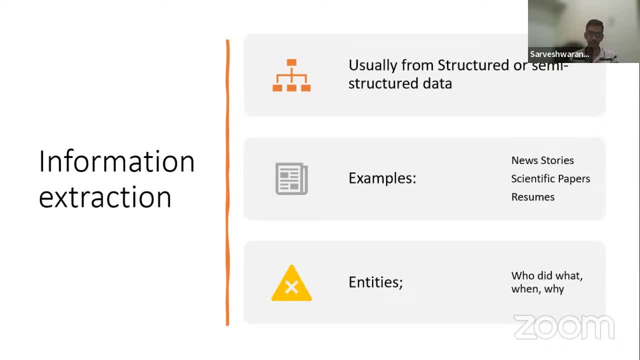 information from an unstructured textual data. The famous example is your Named Entity Recognition NER. Most of you should be aware. So, Named Entity Recognition- What is an entity? Who did that? When, Why? So there are a number of entities Say: 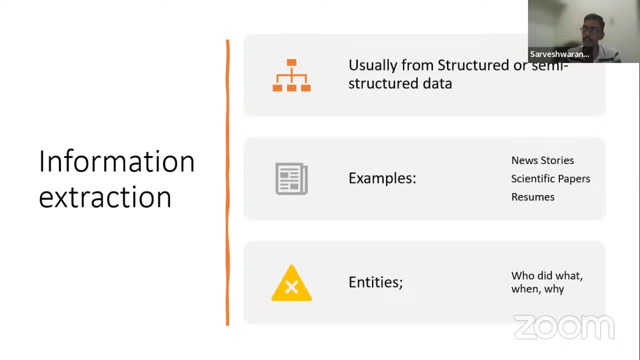 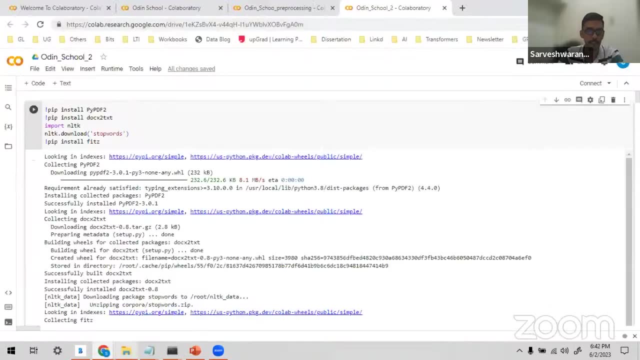 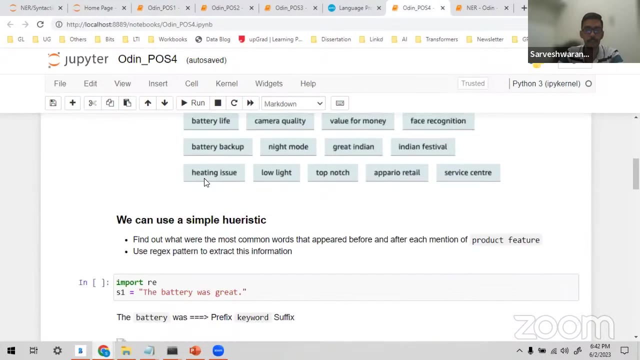 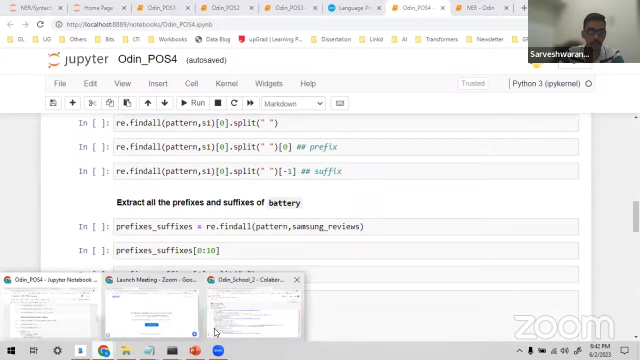 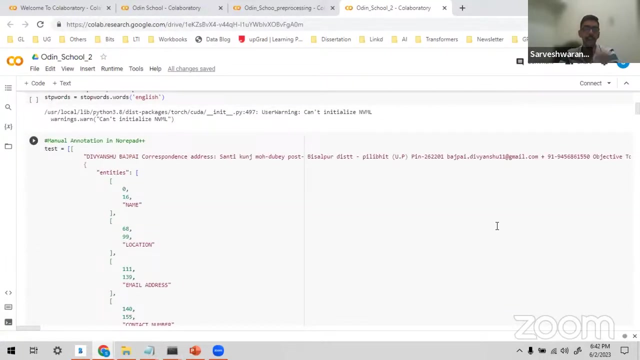 for example. let us take an example. I have a number of examples. Let us go here, Just go here. So what is an entity To make you understand? say, for example, I have. So this is an example from your resume shortlisting. So I have various different entities, such as name, location. 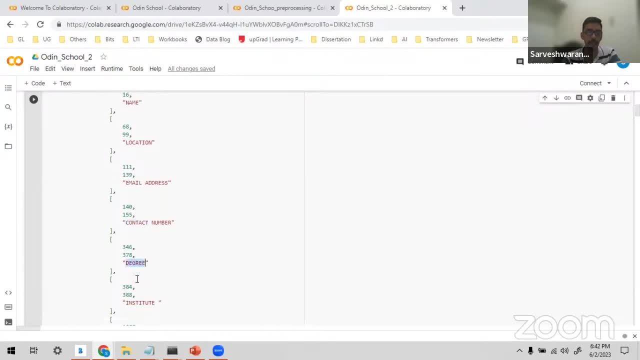 email address, your contact number, your degree, the institute skills. So, out of all the information that is present in that you are given, there are different entities For an, your resume, which interests me more. I, after all, need your name, location, email address. 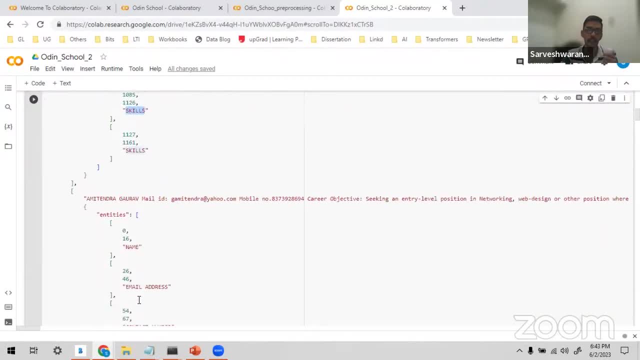 contact number? what is the institute, skills and years of experience? right? So I need from your one, two, three pages or n number of n pages of your resume. I need only these information to do an initial screening, right? I cannot go through all the hundreds of resumes. 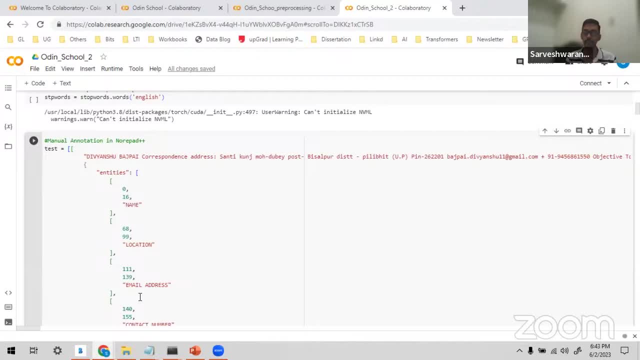 So this we have created? right So, to do an initial screening process, because we see nowadays a lot of technical managers are getting involved for data science, resume screening, right Yeah. So what happens is it goes beyond the scope of an HR, So the HR may not be able. 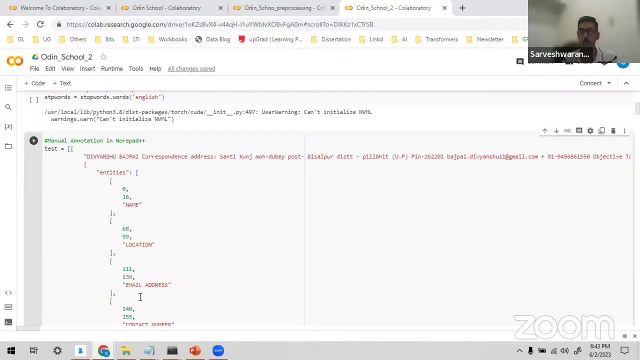 to look, take a closer look to all your skills right Now. the technical managers are getting involved, So the role of an HR manager is to take a closer look at your skills, right. So the role of an HR manager is to take a closer look at your skills right Now. the 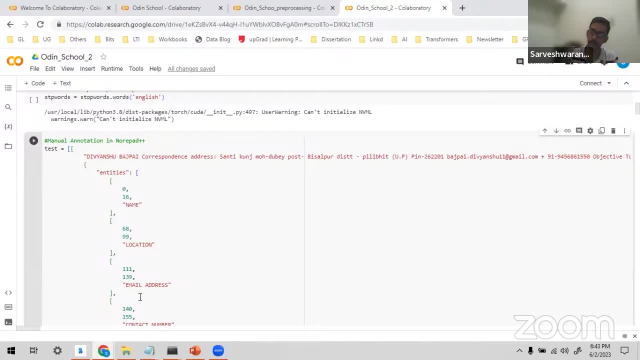 technical manager is not to shortlist resumes, to spend a lot of time in your resource management hours, right, So they are getting paid for a different reason right Now. their scope is changing. So how can we make a smarter use of this information, this NER, and we can. 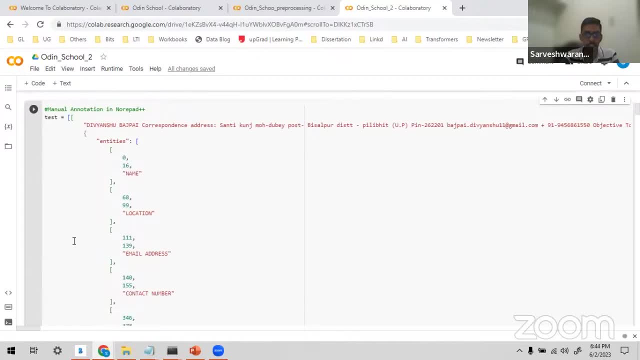 make an informed decision, right? So we can extract all these entities from the resume, right? Maybe I'll explain this in detail, Okay, so I'm just explaining what is an entity. Okay, so we extract all these entities, we convert into a JSON format. Once it is converted into a JSON format and I vectorize all your. 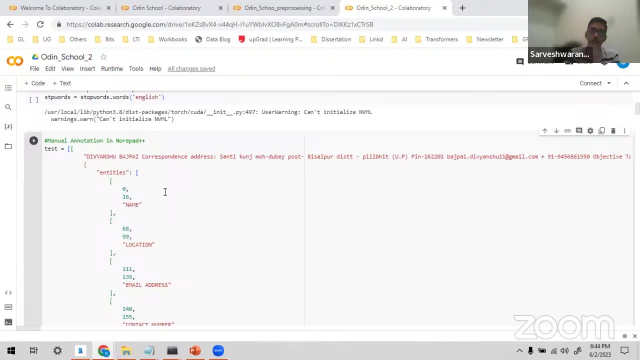 words, the text. to do any modeling, your text should be vectorized. You can use an PDF, idea, term, frequency, English, etc. So you can do any modeling. your text should be vectorized. So I'm just explaining this. So you can do any modeling your text should. be vectorized, So you can do any modeling. your text should be vectorized. And what is an entity? It's essentially a vectorizer. So the vectorizer is a dot, font frequency vectorizer, a count vectorizer. There are so many different vectorizers, So the very 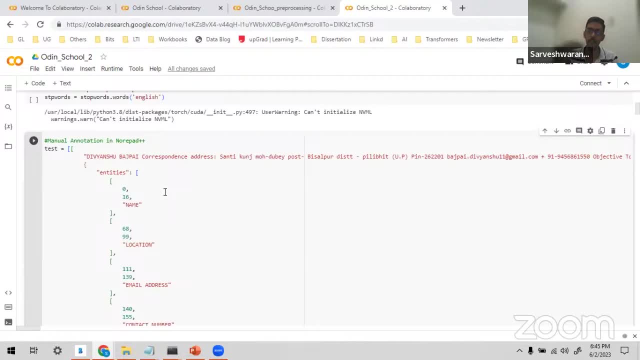 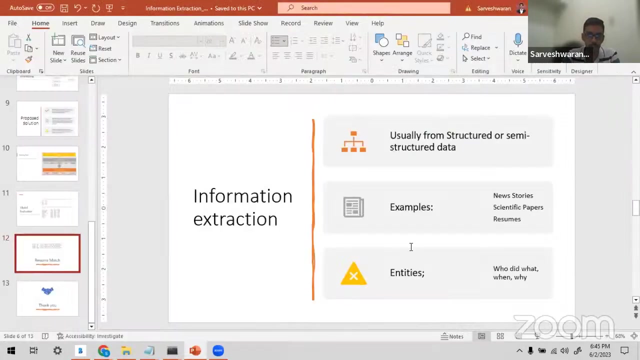 famous is tf-idf-vectorize: You convert into vectors And the other side, you also have your resume. Your resume is also vectorized and I do a cosine, similarity match, and I can get your rank order right. So and then, for every resume, what does the percentage? 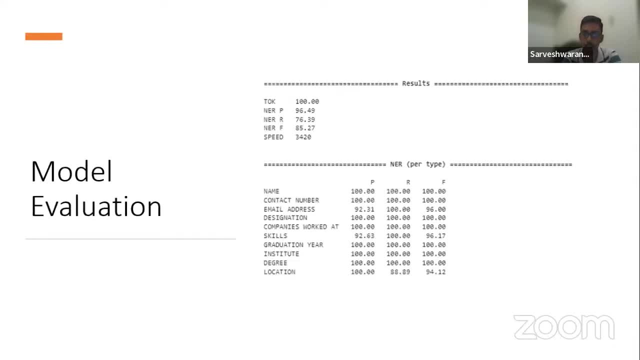 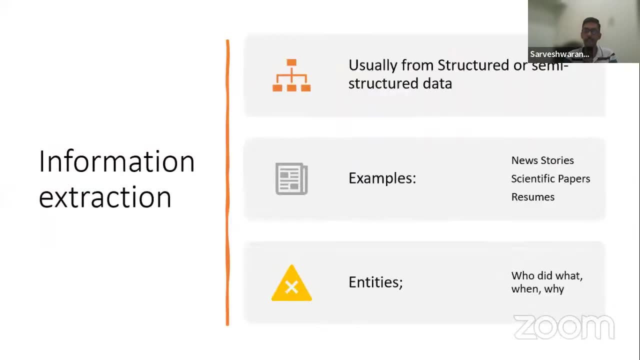 match to the job description. And this one example. maybe I'll show you how to do it. uh, go one step by step. so i'm just trying to give an example of what an information extraction is right. so, uh, the uh. so, after all the information extraction from all the semi-structured data, 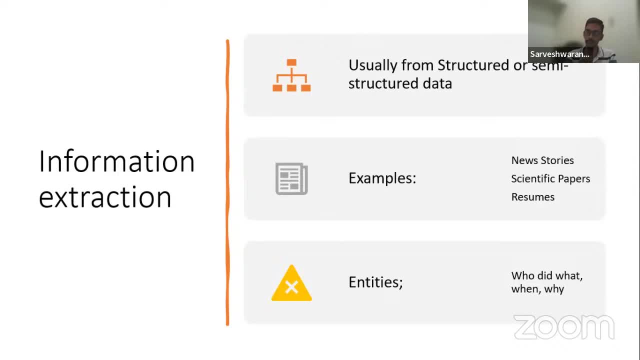 what is in semi-structured data, json, json format is in civil structure and uh, the various unstructured data. you convert the data to one structure and then you can do the information extraction. examples from your news stories, your scientific papers, your resumes, you extract only the useful information that is of your own. how do you do the information extraction? 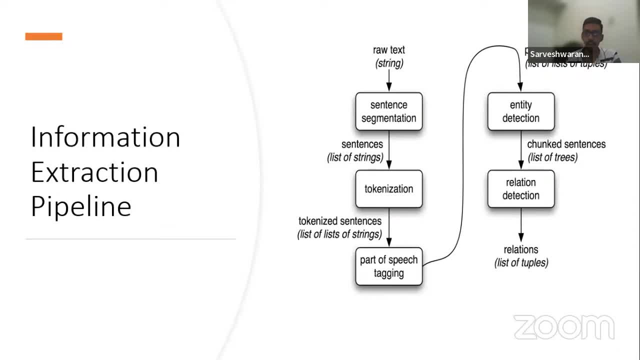 right, so i do the information extraction, uh, using this uh five step process, right, uh, it's easier said than done, but yeah, so we first uh start with the raw string, raw text, and we do the sentence segmentation once i do the sentence segmentation, right, uh, so the basic pre-processing goes like this: right, so 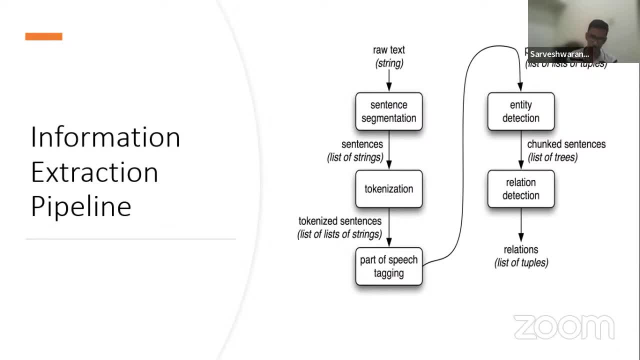 what is the word tokenization? we also do. the po is stagnant, so i break down all the sentences, the raw text, into sentences and then, once i have broken down the raw text into sentences, and i do the tokenization. so what is the word tokenization? i break each and every sentence. 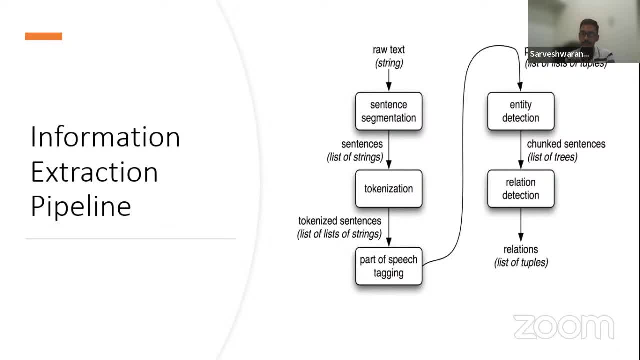 into different tokens, into a list of strings, and the third step is i'm going to use some part of speech tagging. i'll show you how the part of speech is done, and then i do an entity detection. what is entity detection? like i showed you, uh, some time back. 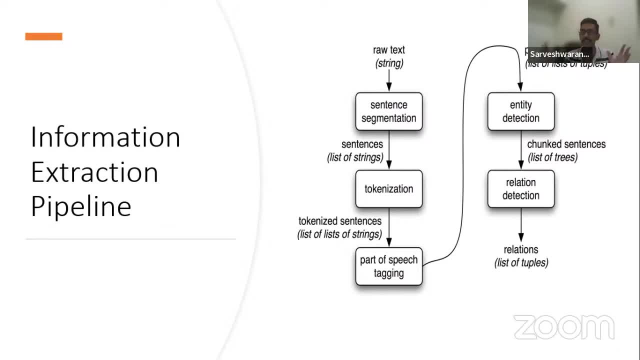 out of all the information i need. after all, the 10 different entities that are present in the system are: in the institute, the years of experience in the resume, short listing. i identify the entities from the resume or from your newspaper or from your research paper, with the help of your part of speedster poa stats. and then i have chunks and 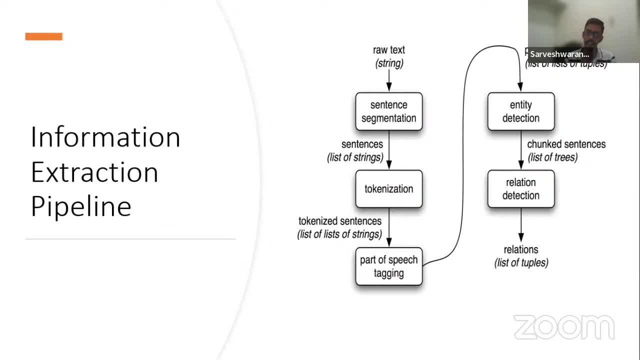 tensors and i have a relation, uh detection and then i find the relations. this is how the information extraction pipeline works. so any questions so far, Sneha, So how do you see the questions? You got it here, Sir. reassurance that there might be some questions coming in, because this is being live streamed on YouTube and LinkedIn. 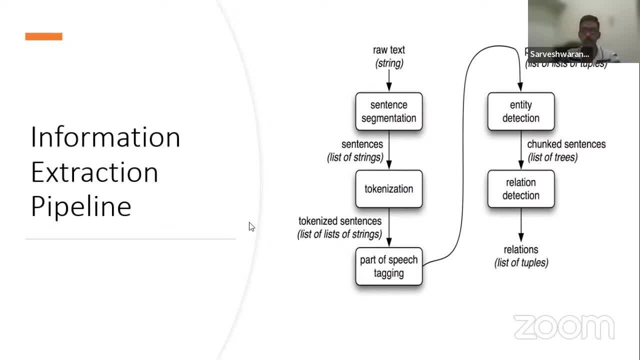 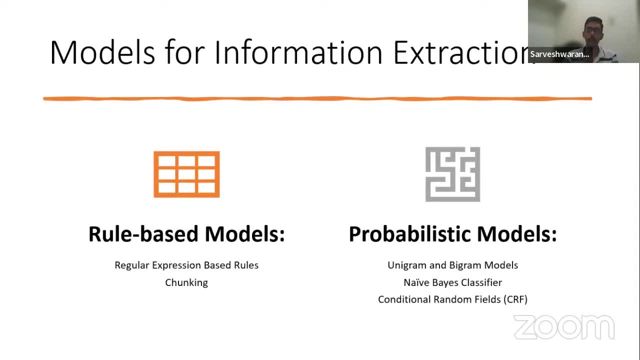 So any questions come up, they will inform you. Sure, Right, okay, Now the models for information extraction is either in rule based or in probabilistic based. So in rule based we use some regular expression based rules. So I hope you know what doesn't reject us. 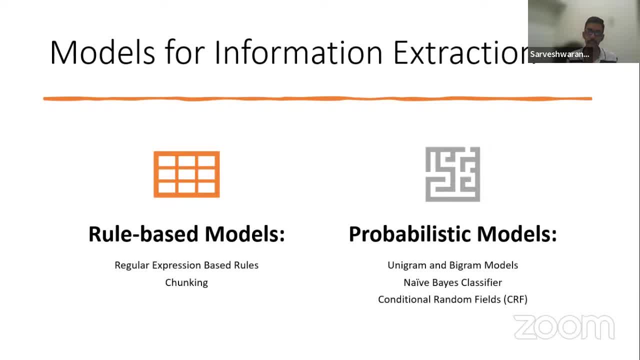 So rule based, So we have various different rules. So we have the quantifiers, your wildcards. So on basis of all these rules, we extract the entities And again in chunking on probabilistic models like in unigram, the bigram, the name base classifier, or in conditional random fields. 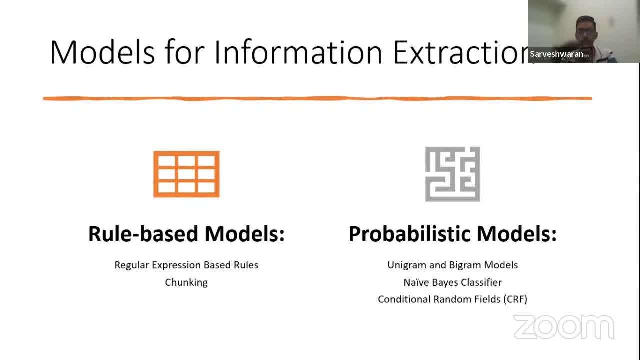 There's a wide topic So I've taken a few different examples. I wanted to showcase what's, in part of speech tagging is, And I also wanted to showcase how an entity recognition is done And a basic few examples. Okay, So I have a few examples around the NER. 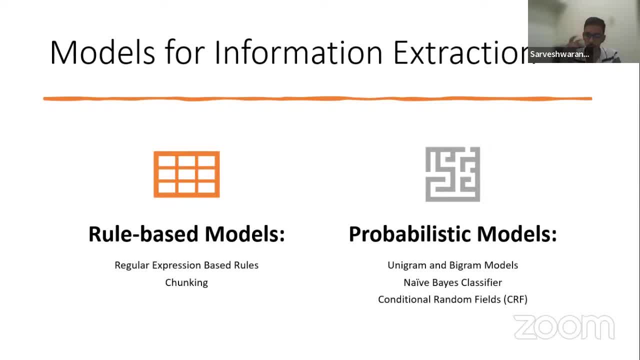 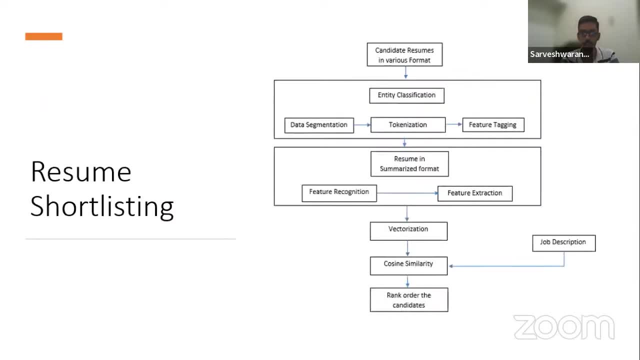 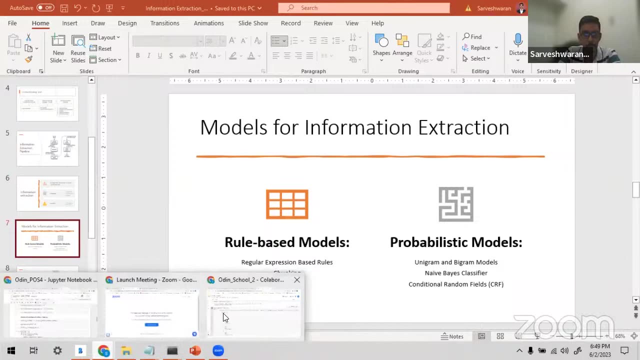 So this is the agenda that I have set. Okay, So if you have to go through all this- the conditional random fields, the chunking- it's much beyond the scope. It takes a lot more time, Okay, Okay, Now, before I go here, let me go through the notebook. 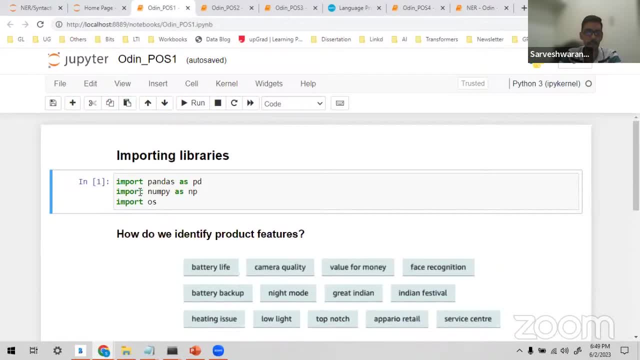 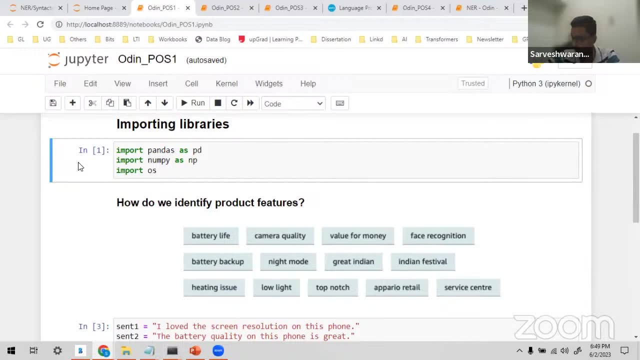 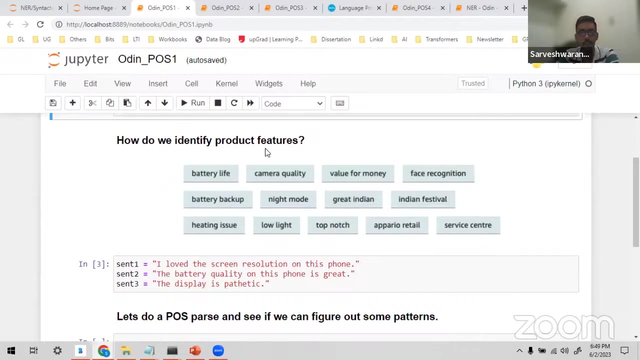 Okay, So I import the libraries: Import Pandas as PD here, Import Pandas as PD And NumPy as NP And import OS. So these are the three different libraries that I've used. Okay, So how do we identify the product features? 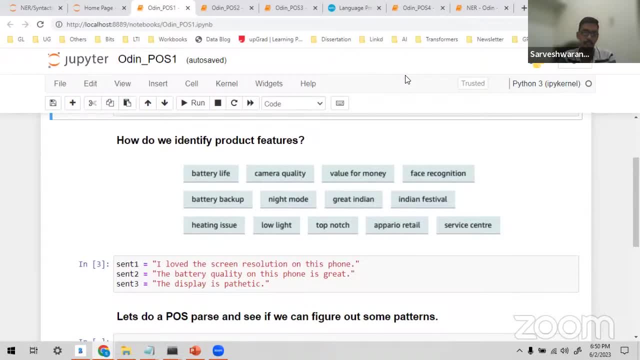 First of all, this is an example for an out of speech tag. How do I identify the package speech? So the battery life, the camera quality, the value for money, the face recognition, the battery backup. So there are so many different things. 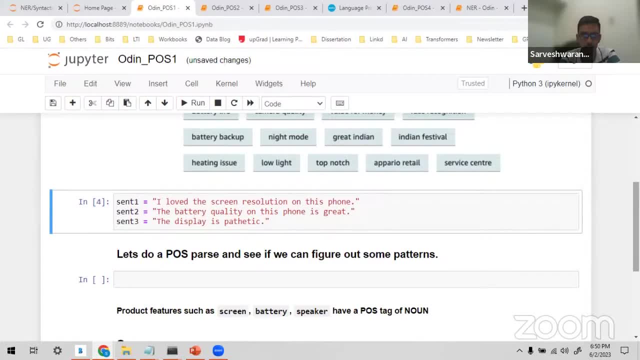 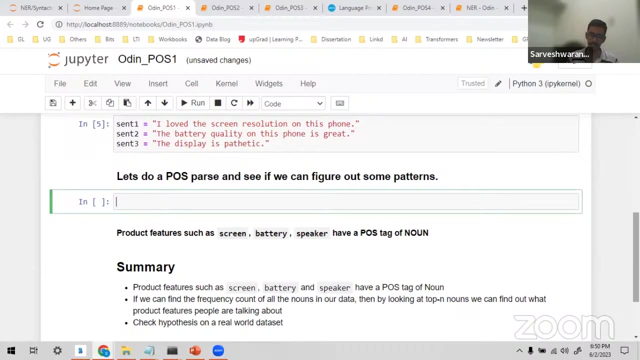 So in the first sentence, I love the screen resolution on this phone. The battery quality of the phone is great. The display is pathetic. Okay, So I have three different sentences, So let's do a part of speech pass and we see if we can infer any patterns out of it. 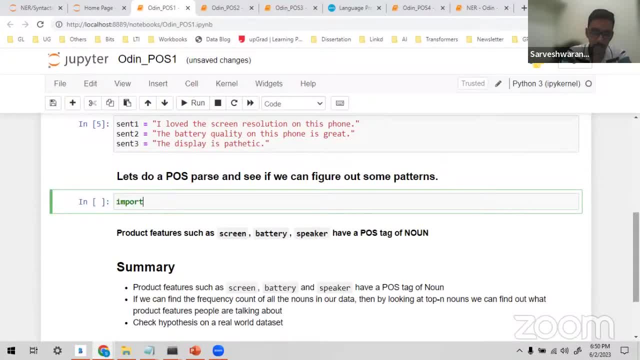 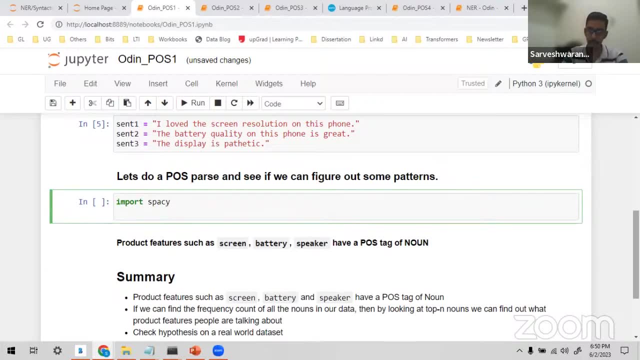 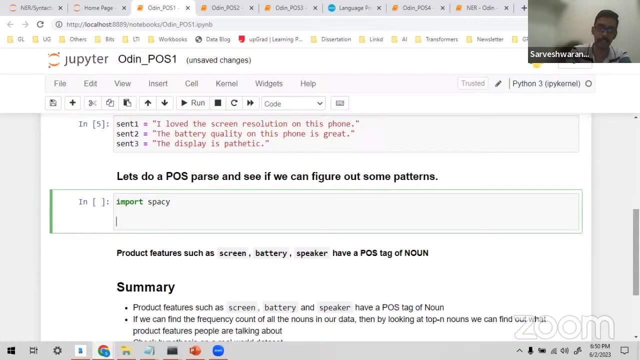 So here for this exercise, I'm going to take an example from, I'm going to make use of a library called Spacey, Very famous library, the Spacey. And so these are all models, the transformer based model. These are all pre-trained models. 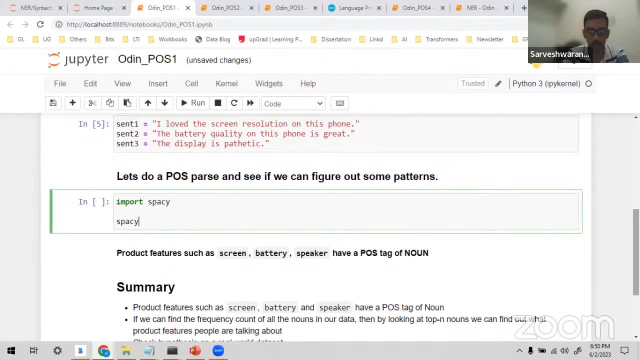 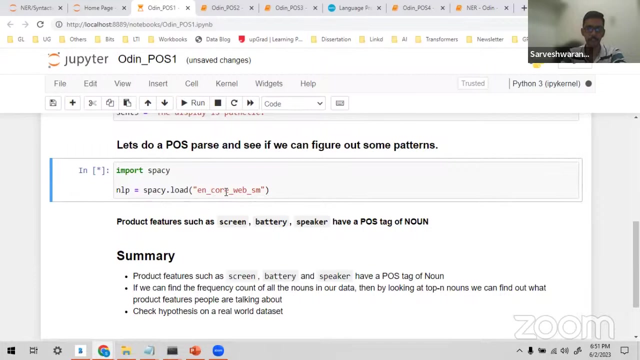 How do I load the pre-trained model? I use a Spaceyload n core web SCM Right. I use this n core web SM English And it is pre-trained Right. So it's a very big library that's pre-trained. 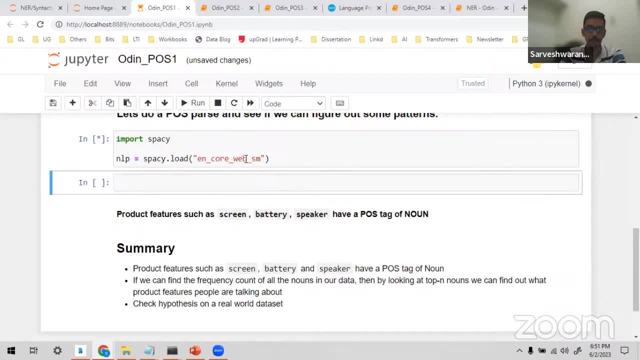 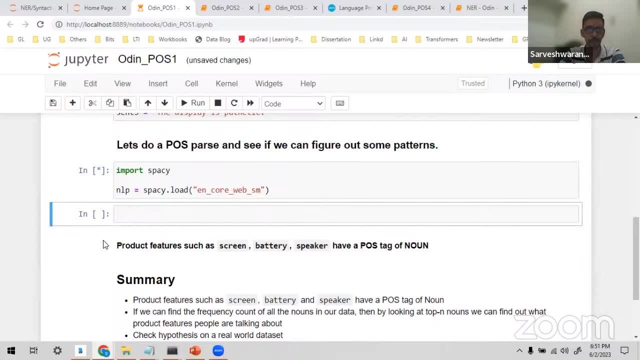 And I'm saving it inside an object: NLP. As you can see, the star indicates that the cell is still running Right, So it's just loading this big model. Okay, Now you can see that it is, That it has loaded. 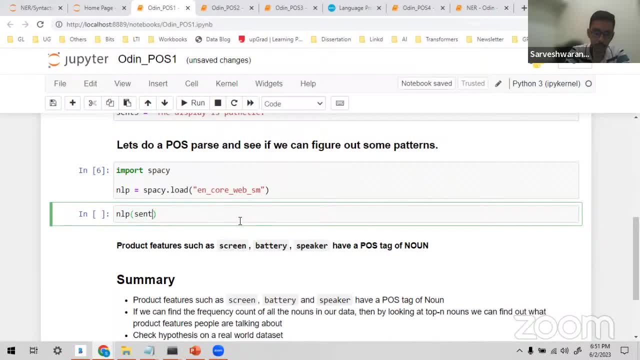 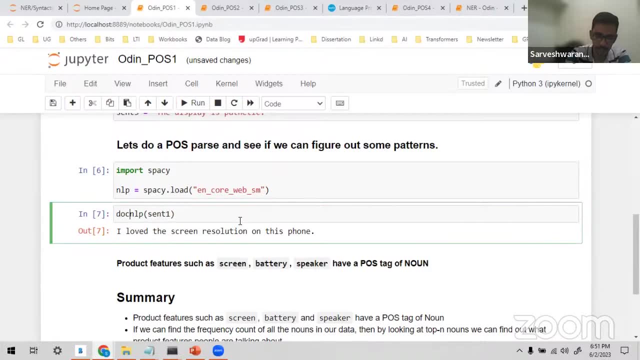 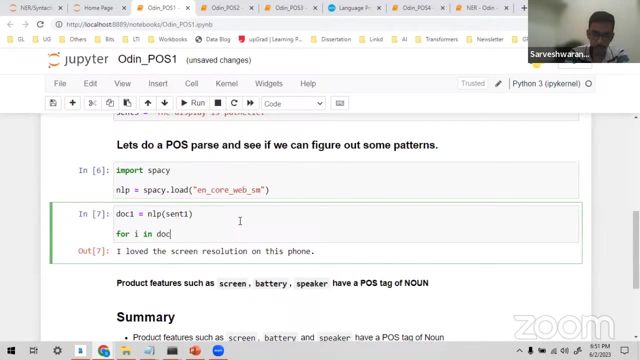 Now let me take NLP of SYNC 1.. Right, So how do I extract the entities For the document 1 here For IN doc 1.. Now I want to print the I dot. What is the text And what is the part of speech? 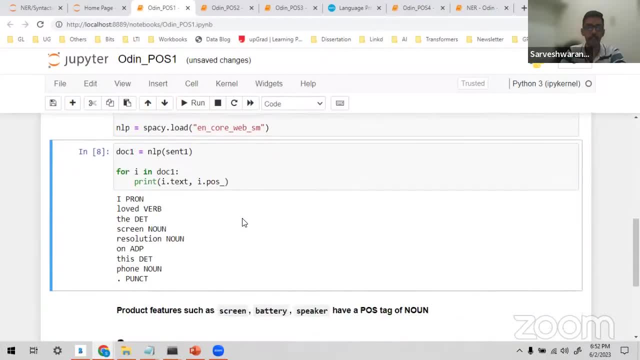 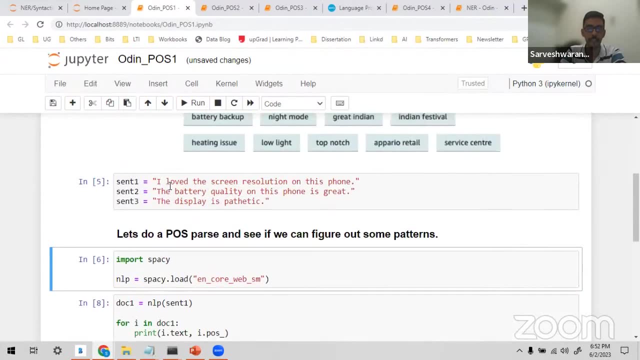 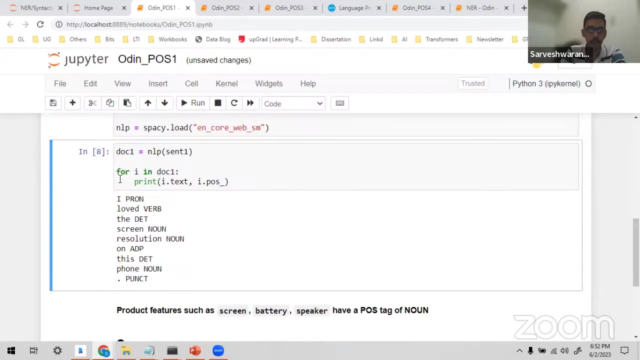 I dot. Okay, Now you can see here I've used this pre-trained model And for this sentence I load the screen resolution of this phone. I'm extracting, I mean I'm tagging, I'm doing part of speech tag. 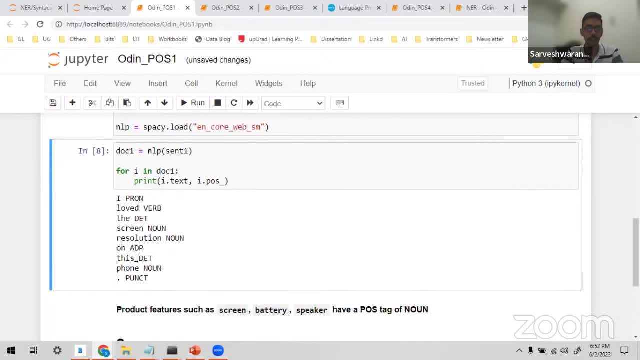 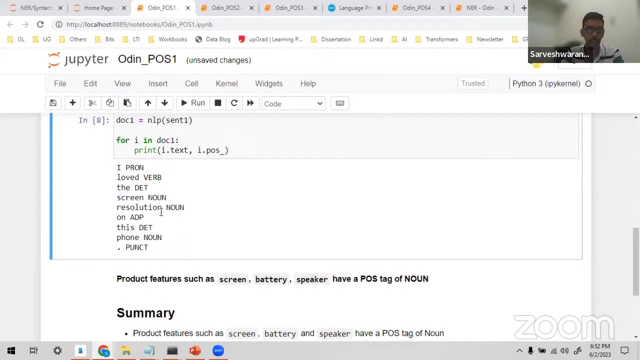 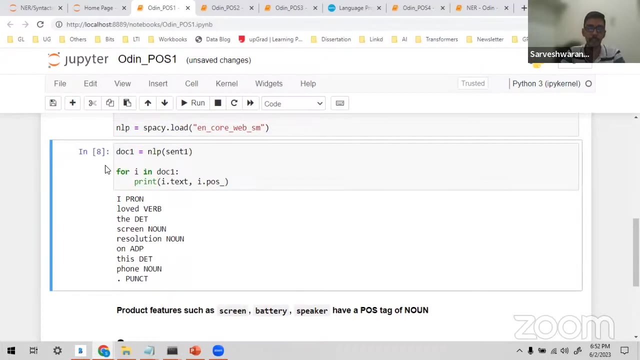 I'm doing part of speech tag. for each and every word I proper noun load, verb the determiner, screen, noun resolution, noun Right. So I'm, I'm extracting, I'm tagging. So there's not an extraction. 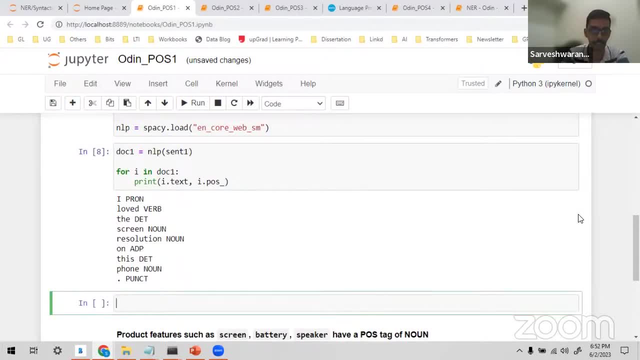 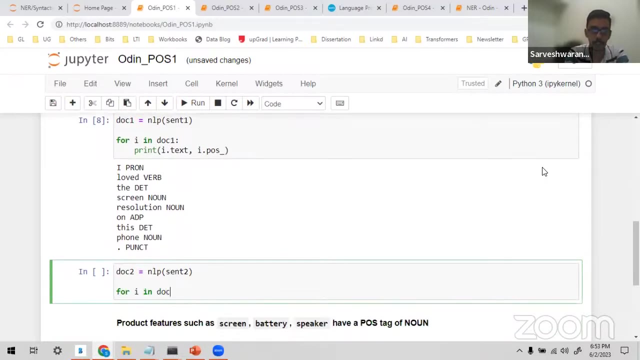 I'm just tagging, I'm doing part of speech tagging. So the document 2 is equal to NLP of SYNC 2.. Okay, Similarly what I'm going to do For IN the document 2.. Now I print: I dot text comma, I dot POS. 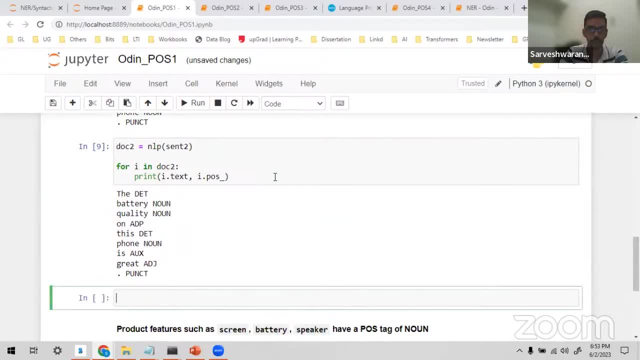 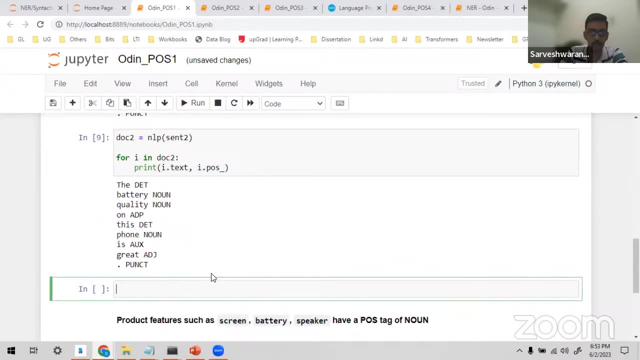 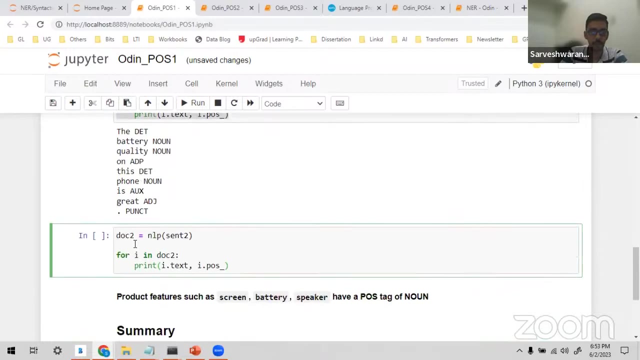 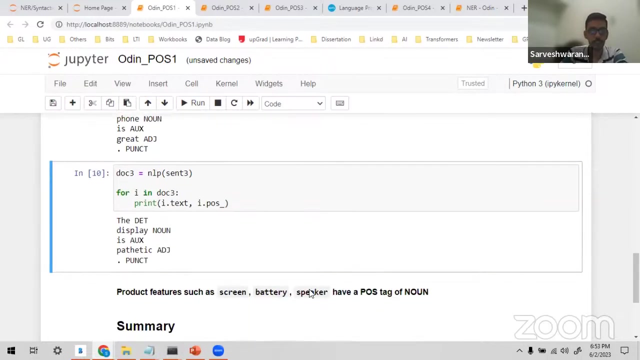 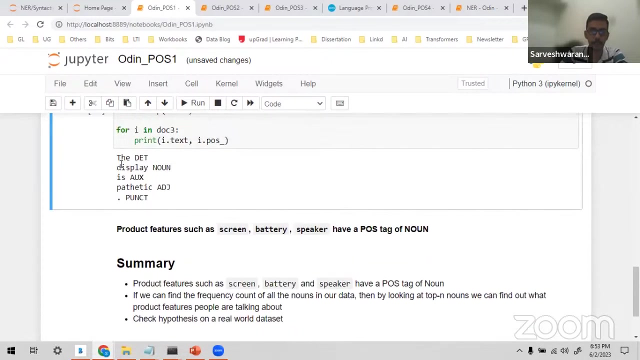 Right, So I'm just understanding. Similarly I'll do for the third sentences. So here we can understand Which are the important features. which has an part of speech tag as a noun? Okay, So the display, the screen. So here the product features, such as some screen battery, the display, 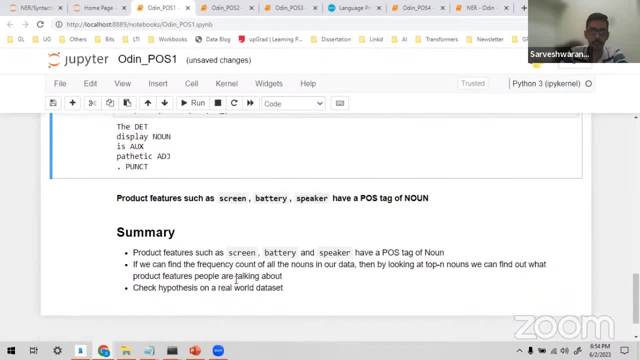 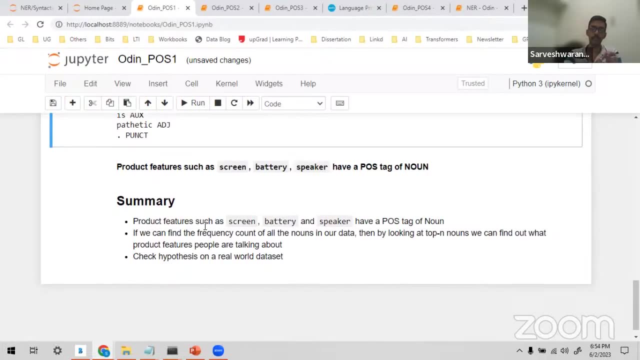 So these are all tagged as noun, Right So. So, further extension to this, what we can do, I have known the important product features. So the important product features, Right So we can, So we know right. So the important entities, the the important entities are always tagged as noun and proper. 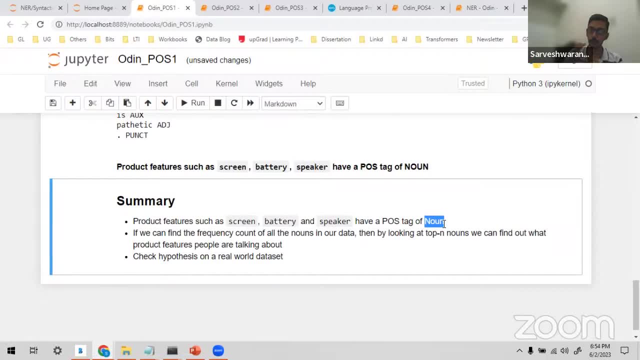 noun Right. If you want to extract the useful information, we can simply extract the noun from that sentences or the document that we have As an as an initial stage Right. So important product features such as some screen display battery speaker. 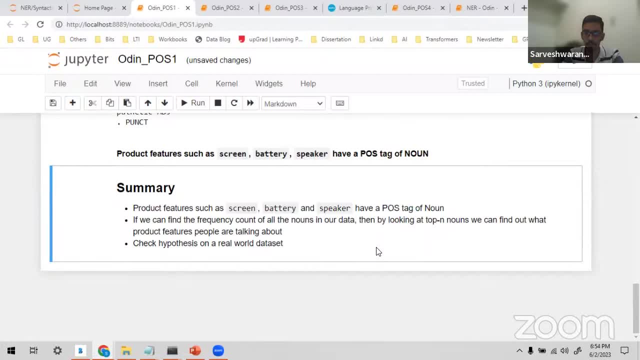 These all have an part of speech tag as a noun Right. The next step would be we can find the frequency count of all the nouns in our data. Then, by looking at the top N nouns, we can find what does this product features that. 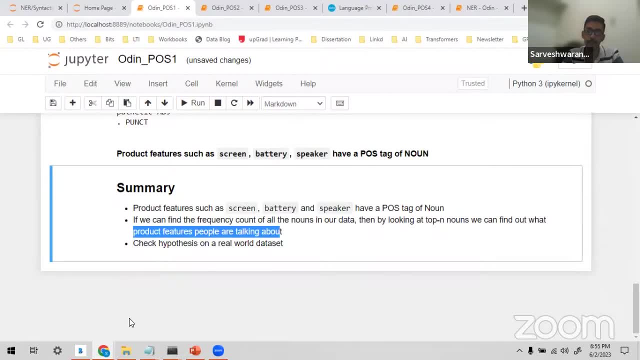 the people are talking about And, extension to this, I can check in hypothesis on the real world data. So what is that? So if I'm going to extract all the tweets about an Apple, Apple product or any movie review that we want to do in a tweet right from the Twitter feedback, I extract all the. 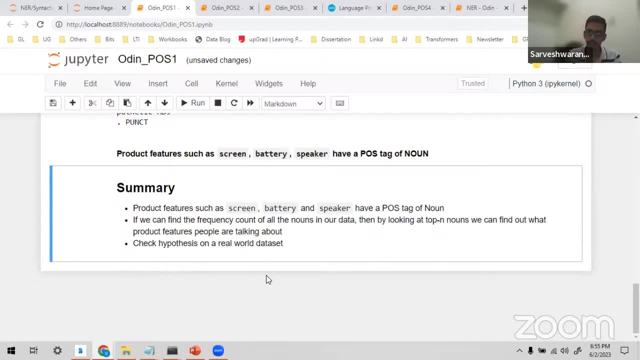 Twitter tweets. Okay, There is a connection from which we can download all the tweets With given an hashtag: hashtag Apple hashtag, the Android- whatever the hashtag you give, you will be able to download all the tweets. So once you have downloaded the tweets, you can do one part of speech tag of that noun. 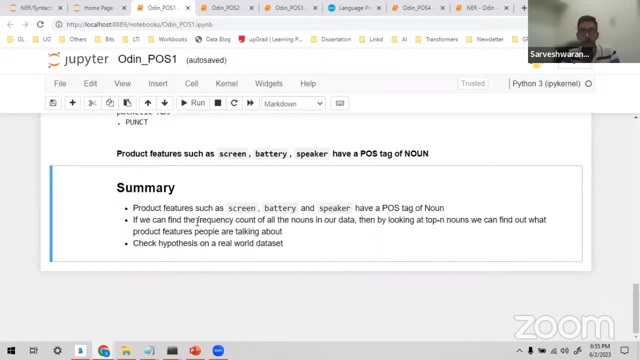 And you can understand what is that people are speaking more about. And you can start doing a lot of exploration by doing some hypothesis testing and the sentiment analysis, By doing the first step, by taking the first step of doing the part of speech tag. 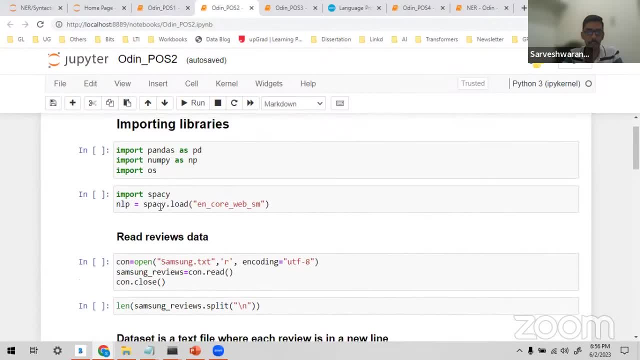 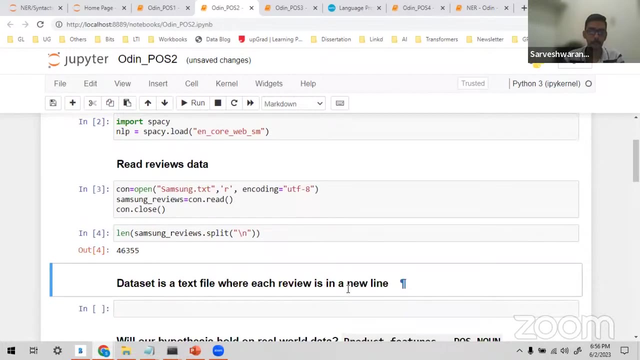 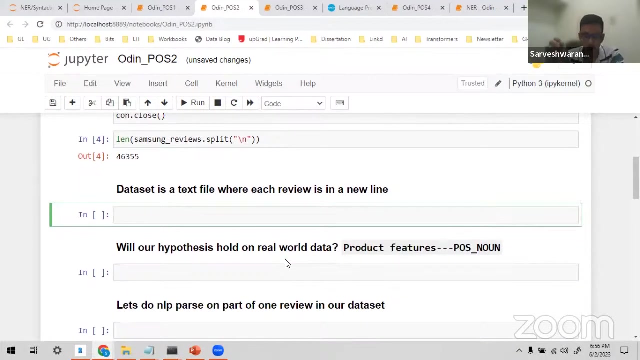 Okay, Another example also I've taken, So here reviews data from the Samsung Right. So similarly, I'm making use of in core web here, Okay, So, and so there are so many different reviews here Now, Yeah, so the Samsung reviews. 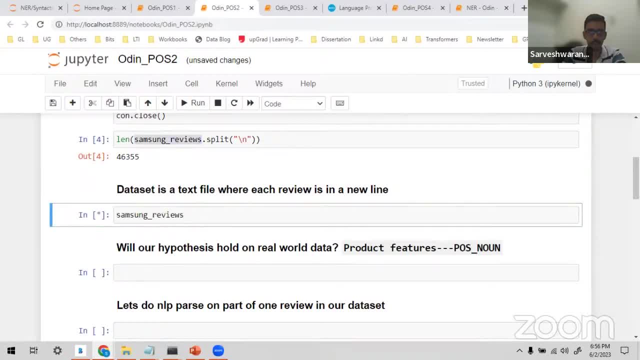 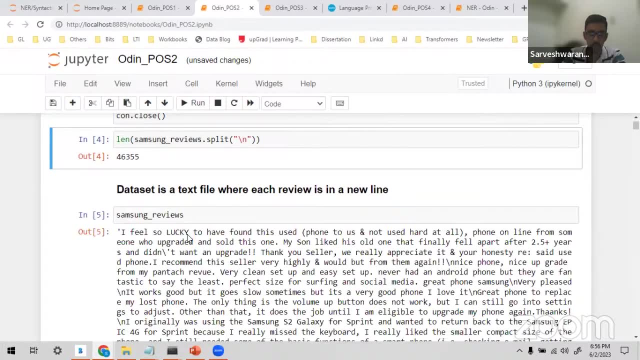 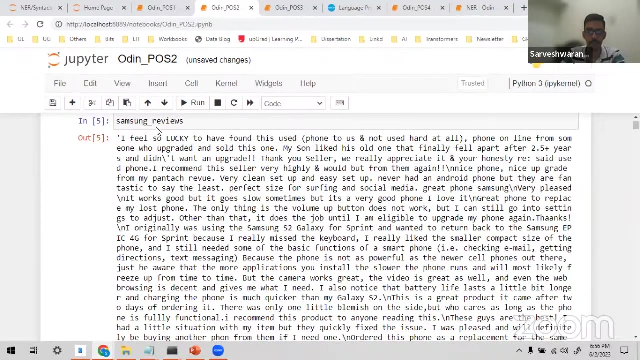 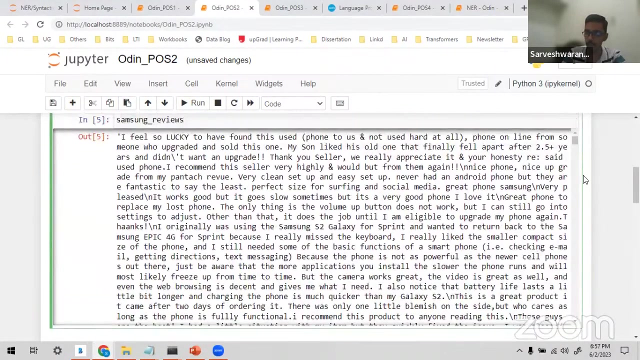 Yes, Just look at the reviews. So every word is in line. Now let us just do that split. So this is where sometimes it is difficult. Okay, So here, sometimes your local system is stuck, even for a small data. So there's an example. 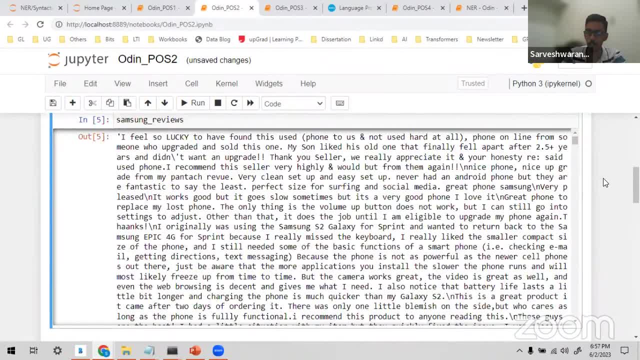 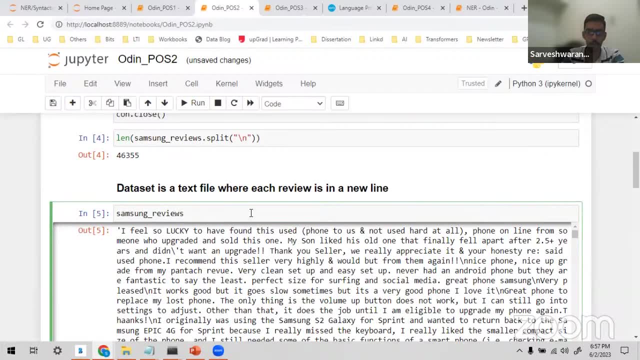 So it's in such a small data Your local computer is not able to support. Right, You can make use of Google collab, The pro version of Google collab, And you can make use of the GPU processes in the Google collab. 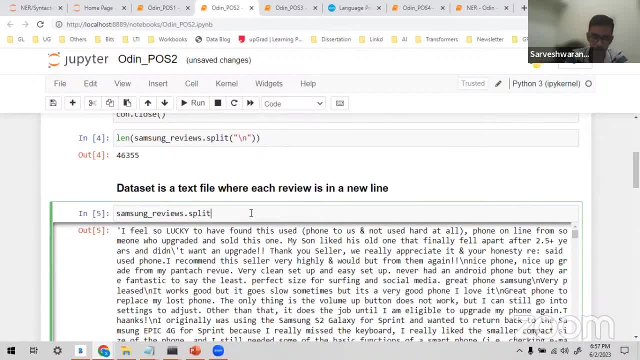 Right, So you can take Samsung reviews And the split, Split it how? Split it into each sentence: 0,, 2,, 4, right, So I'm giving an escape sequence. N is a new line. Right, So the escape sequence new line. 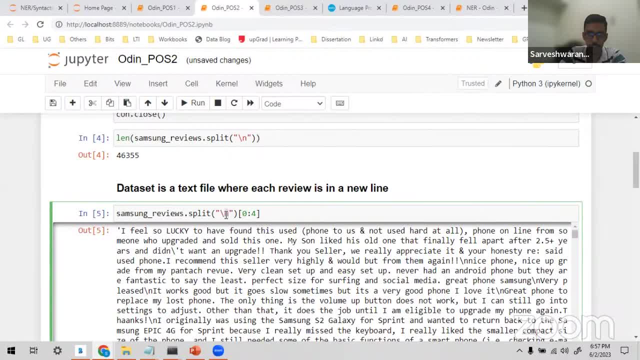 So I'm splitting with respect to a new line. Show me the first four, the reviews. Right, I'm just showing. So the indexing starts from zero And once the indexing Starts from zero, you can make use of. You can make use of. 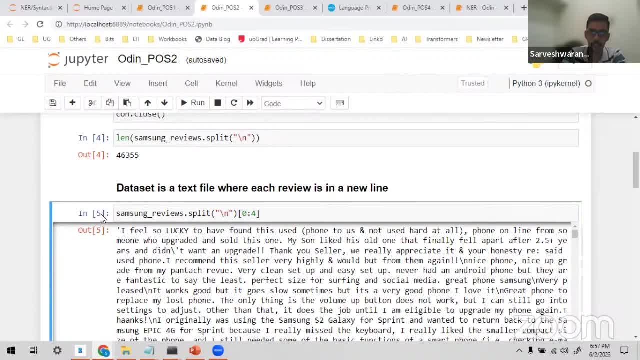 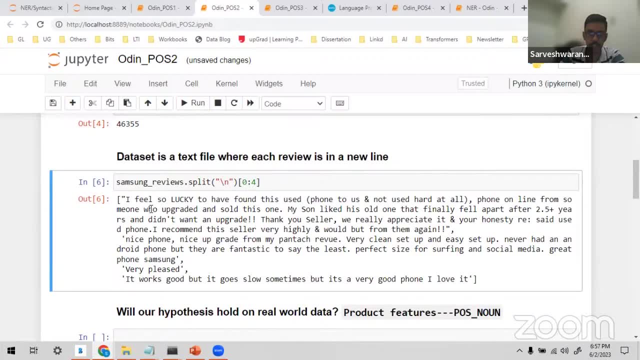 It like a Like a single line, A single line, So it can be A line. It can be Two lines, A line, A line, And then it can. indexing starts from zero. So I feel so lucky to have found this used phone online from. 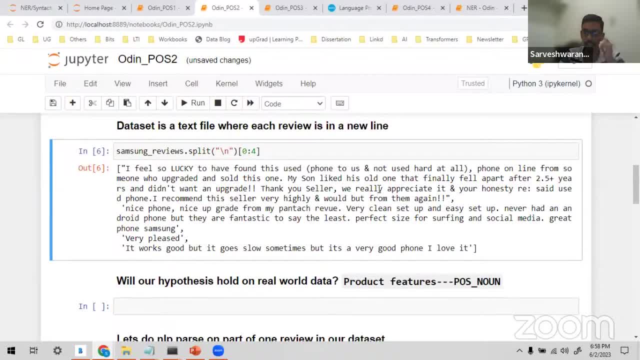 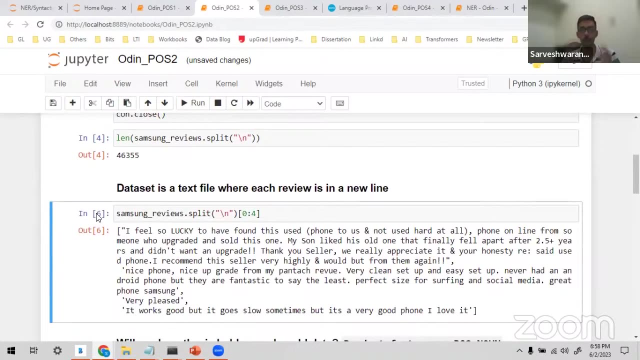 someone who upgraded and sold this phone right. So my son liked this one, So there is a review, So very pleased. It works good, but it goes slow sometimes, but it's a very good phone. I love it. So once you have such a kind of text or feedback, you can do a lot. 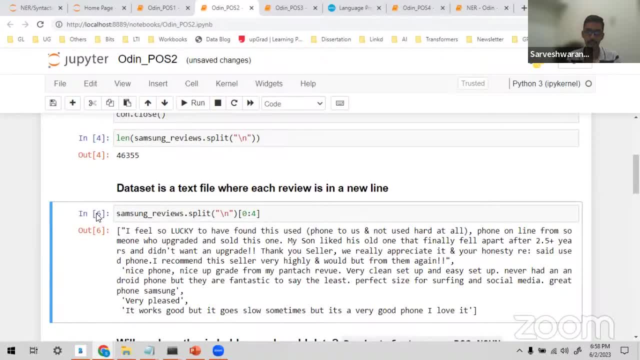 of things. You can do a sentiment analysis, You can categorize, You can do a topic modeling. Again, you can think about this: if you're working in an operations, There are so many tickets that's raised right. So what are the current days people are doing? They're. 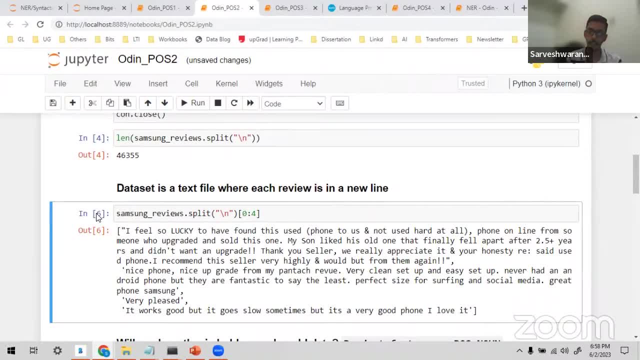 tagging: What is the priority of the ticket? P1, P2, P3. Tagging of these three different tickets- Priority one, priority two, Priority two, priority three- So you can automatically classify. Automatic ticket classification is an example. It's an extension to all this information extraction. Your POA stack right. 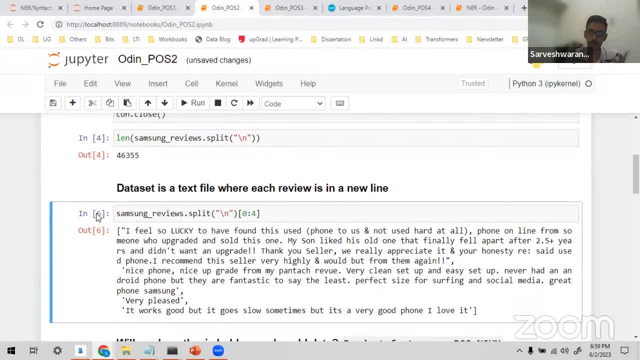 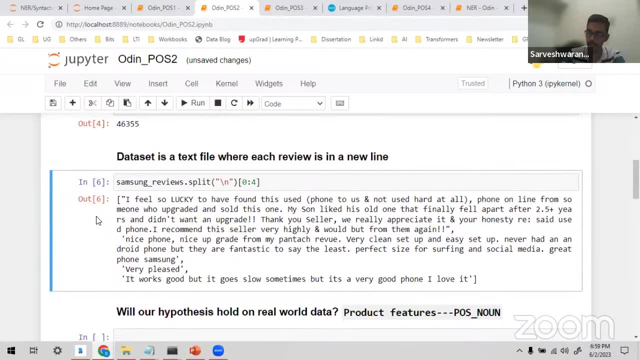 So you can suggest this, the use cases, to your organization also. So automatic ticket classification And you can do a sentiment analysis and you can route. if you are doing a topic modeling, you can route the tickets to your organization, So you can do a sentiment. 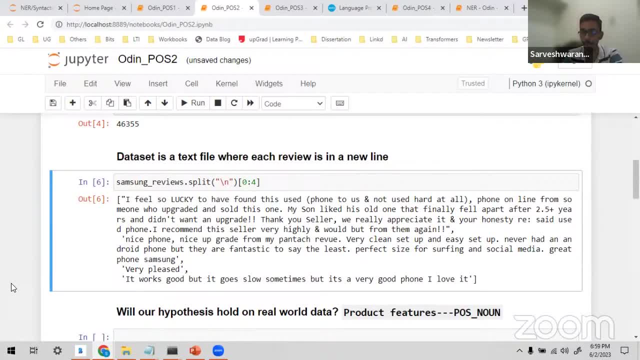 analysis and you can route. if you are doing a topic modeling, you can route the tickets to your organization. So you can do a sentiment analysis and you can route your organization. Right, If there is a PO ticket, there are 10 different PO tickets, right? who is specialized? 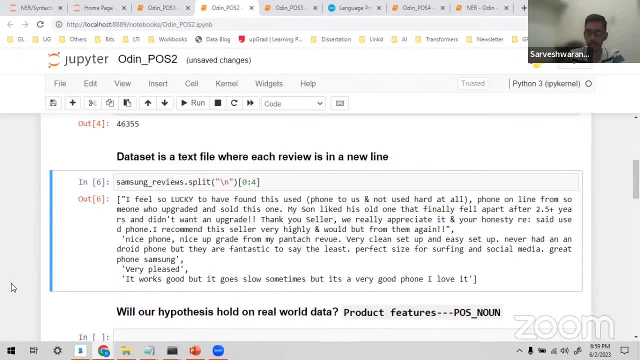 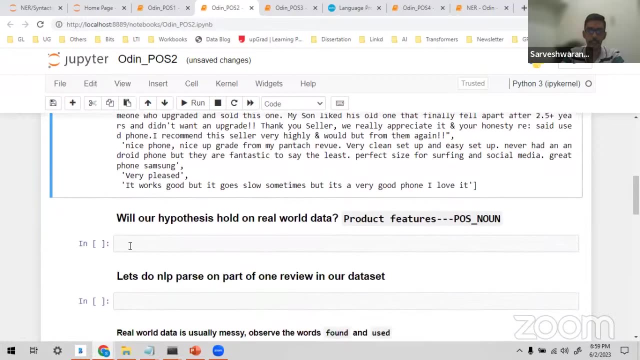 in login issues. So, for example, there's a login issue Right. Who is specialized to a login issue? We can automatically route that ticket, the PO ticket, to the assigned person Right. So there are a lot of applications using this element Right. So will our hypothesis. 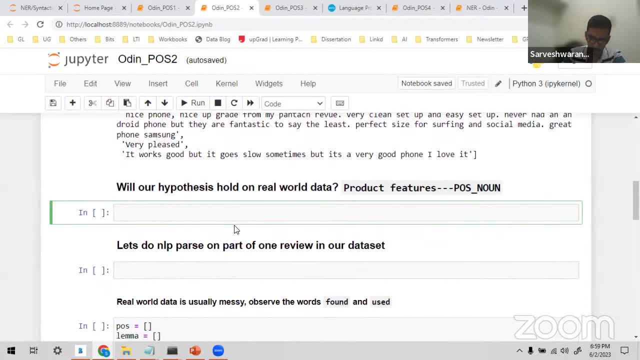 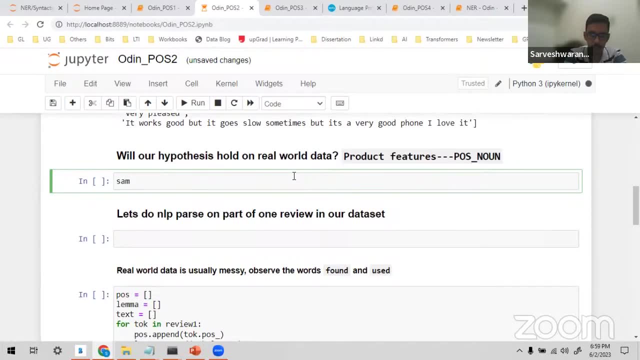 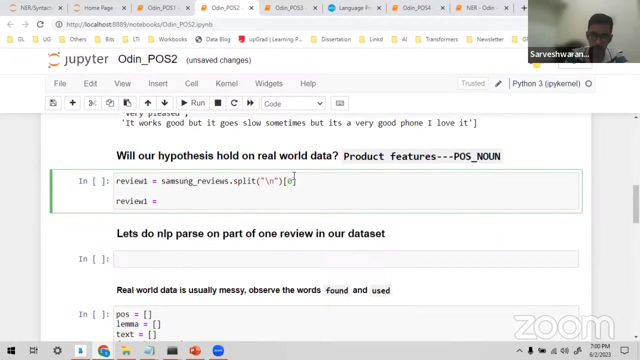 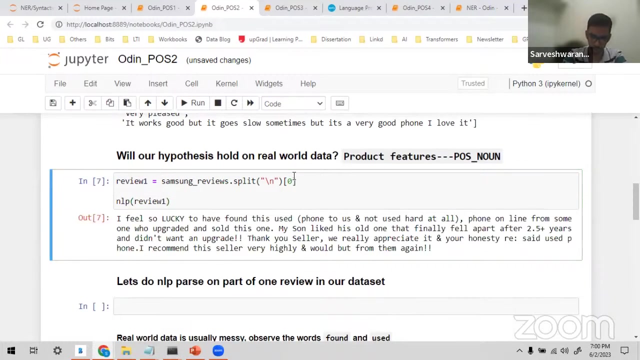 hold on real world data, right. So let's take P2.. P3. Right, Right? So let us take the Samsung reviews and split and take the first one out of it. the review. one is equal to review, one is equal to NLP, or hold on NLP of a user, okay. 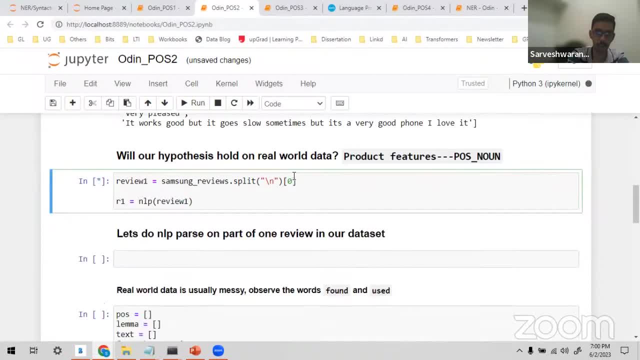 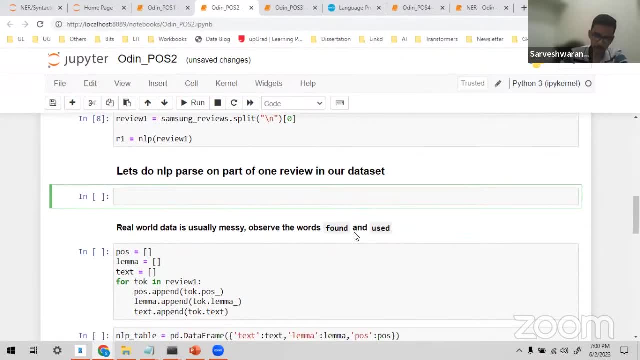 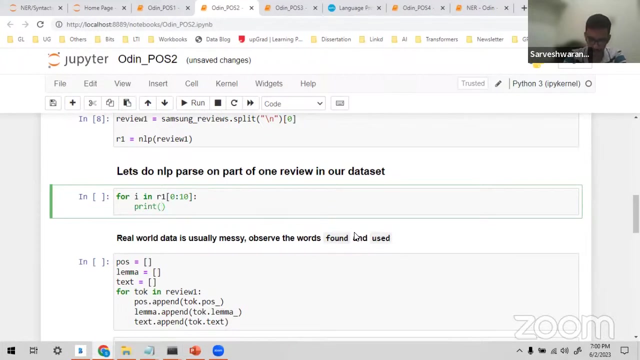 So let me tag it as R1.. Now let us do NLP parse on path of one review, one dataset, right. similarly for INR1, right, so there are so many. let us take 0 to N, okay, so, and then print itext: okay, and. 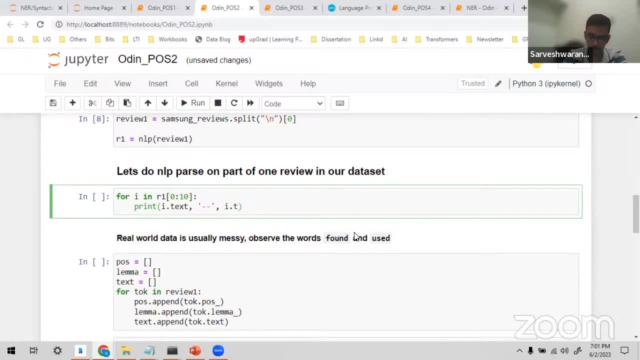 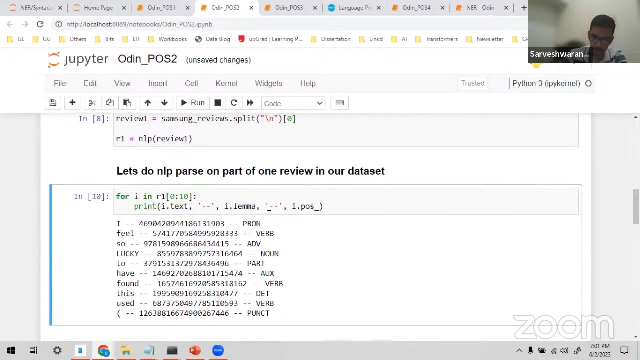 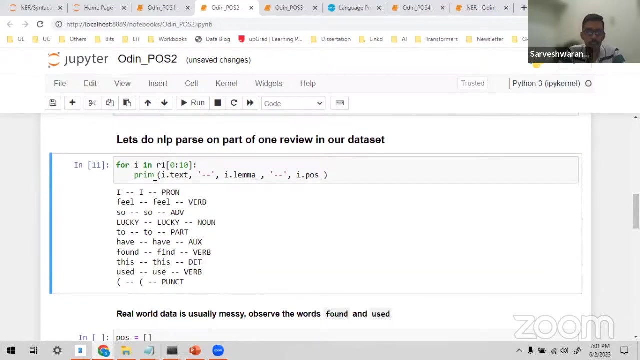 then we put itext: So itos, now let us also add inema. Okay, Now, what have I done? I am taking each and every word and I am extracting a lemma upon sentence. What is a lemma? Any idea what is lemma? Or what is a root word? I convert. 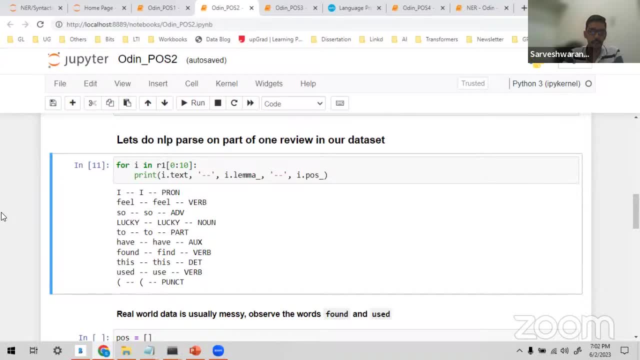 every word to a root word. I do not want to have the verb have, having See, found, find, It is converted to its root word. So this is done using two different words: stemming and lemmatization. 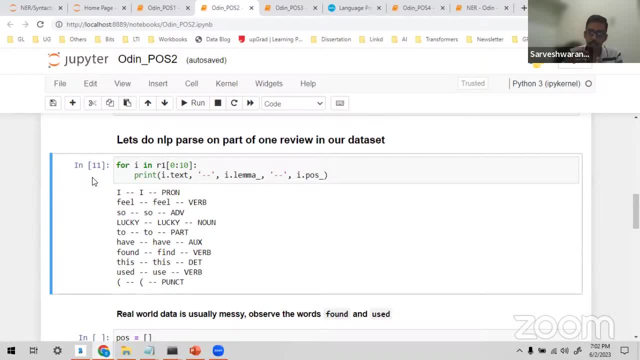 So the stemming converts every word to a root word. on the rule-based format, Lemma accounts the part of speech tag and it converts itself to its lemma. So there you called us in stem words, here you called us in lemma. of that word, the root word, I hope I have. 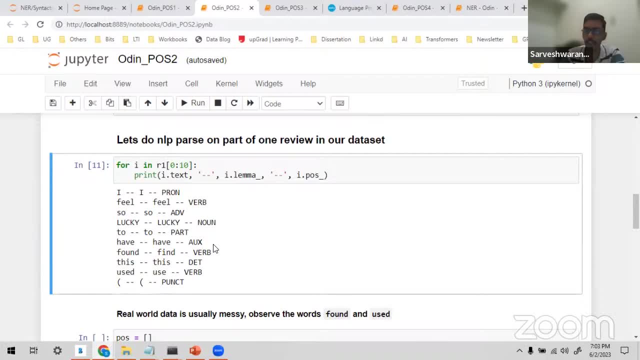 stayed for this long. I am just making it clear. So there are two ways of converting to word and root words. One is the stemming method and another is lemmatization. So the stemming just converts gradually with the rule-based and converts to its root word. 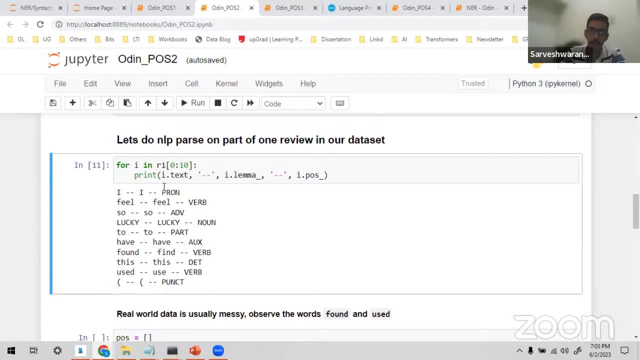 And lemmatization is another technique. It makes use of the part of speech tag and on basis of that part of speech tag it converts to the word and that is lemonization. But based off the part tag and based off this, which roupage? and let me analyze this- It 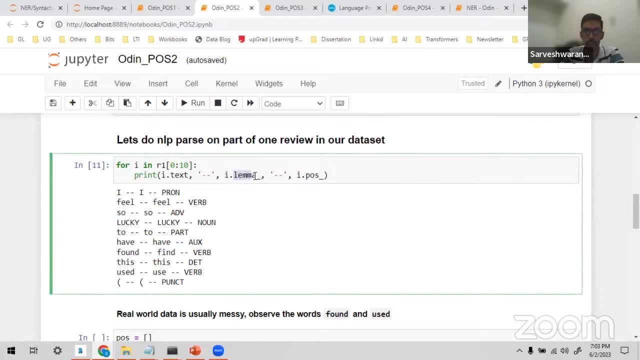 is almost the use of lemmatization, which is just common with a help muốn make a different change. The simplification is früher and the protect number The use of speechdam. You just converts the extended word to lemma of its worth. So here, one thing that we have done. 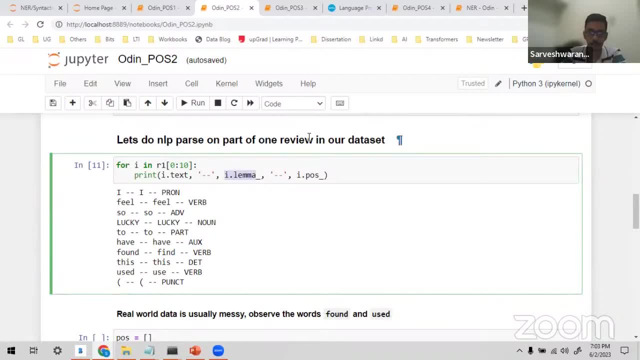 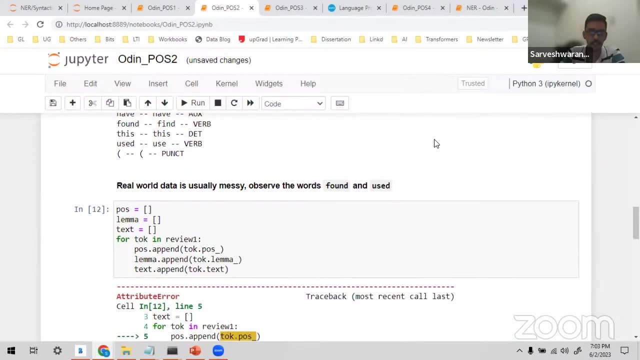 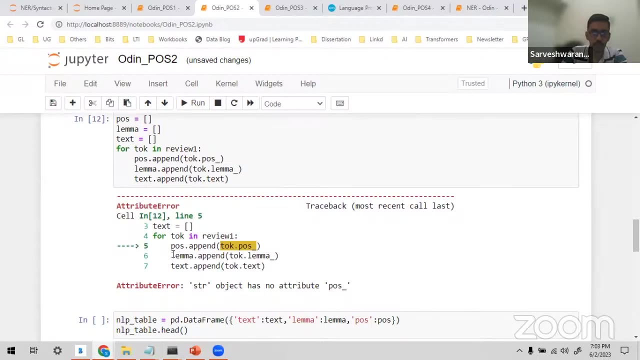 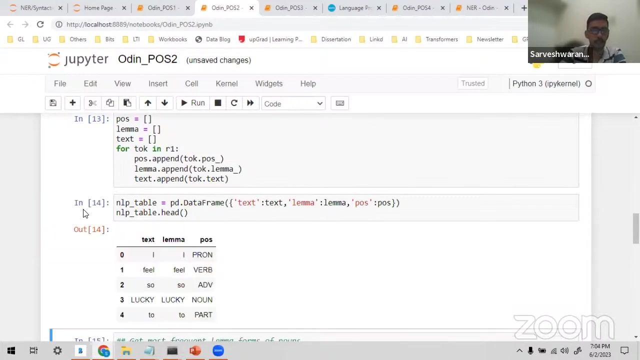 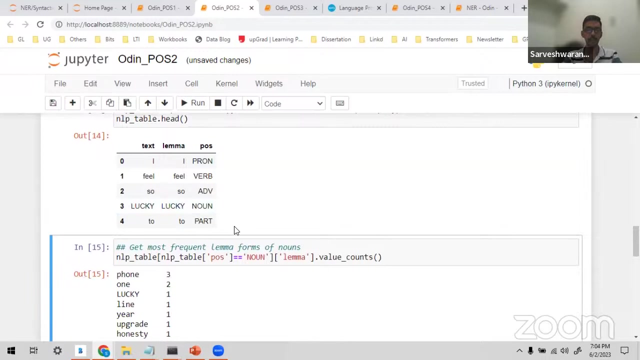 more is conversion to a lemma. Now let us see So for R1, I am just converting it to a data frame, proper data frame. So the moment I make it to a data frame, so I can do a lot of things. So here it is. 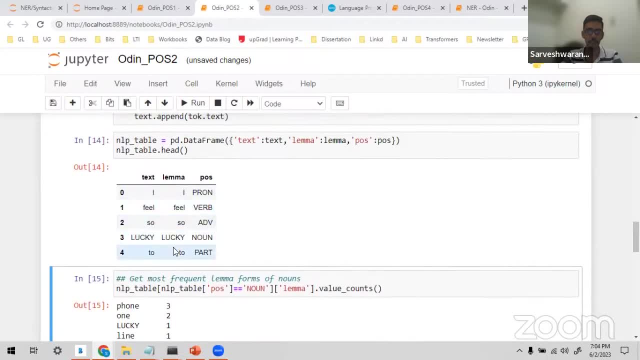 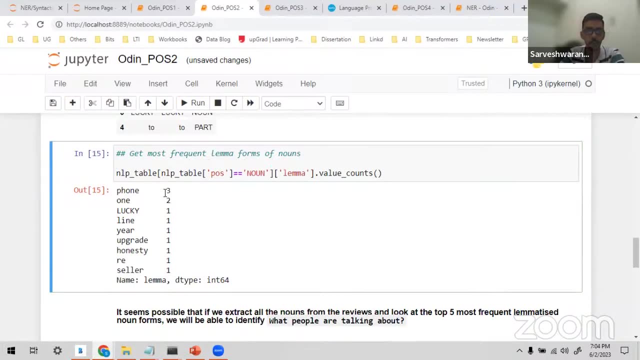 all, it is not an inflected word, these are all the straight form of the word. So here and then I am converting most frequent lemma forms of the nouns: the phone, the one lucky line. So these are all the part of speech which is tagged as a noun and I am just taking 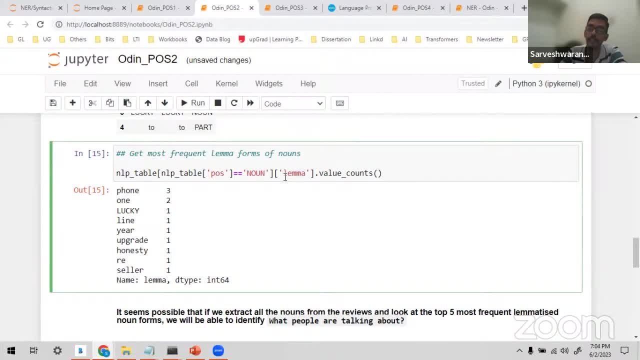 the lemma of that word, in sense Removing the inflection form of the word. what is an inflection form of the word? I have a word called as playing. I convert the playing to play, I knock off that ing and I make it to play. going to go, driving to drive. So I do not want to have a word to. 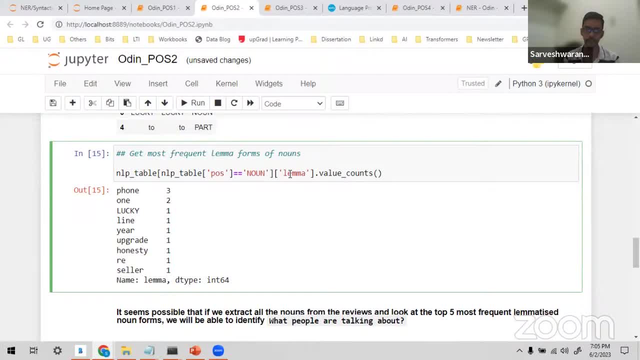 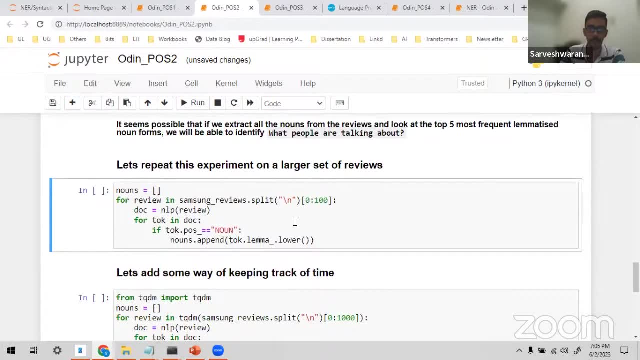 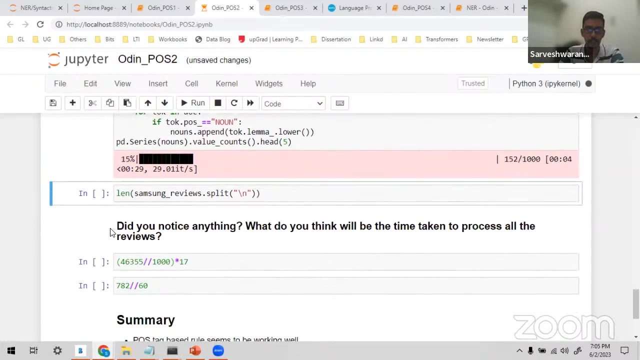 be inflected in form: Right. grammatical sums: right. so i make use of the part of speech tag and i convert to the m of it, right, and then i repeat the same experiment in larger data set. okay, so let's see how it goes. so it takes. 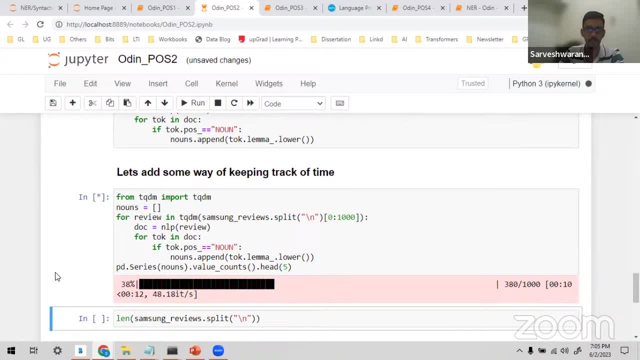 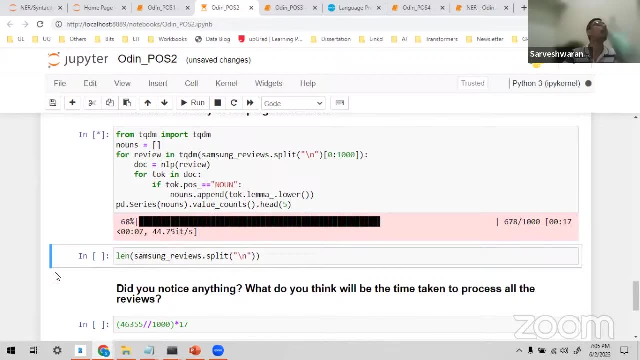 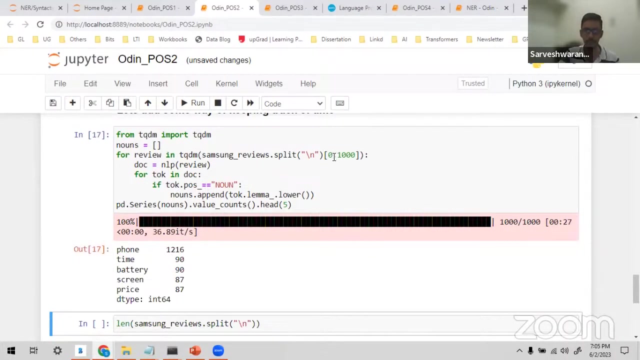 some time let's follow so when you're working with image and text, so it's better to have an higher configuration systems, right? so with i have taken very simple uh for two thousand records. it is taking such a long time, right? so i have uh, sometimes i have. 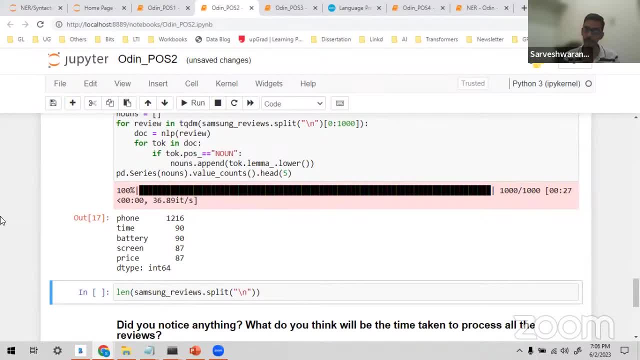 lost patients. so sometimes the models used to run for hours together. right, it will take, uh, five hours, six hours, right? so, and then, if, if we have to do one small fine tuning and then we have to go back right and then do a small fine tuning and then again wait for five, six hours, right, so that's. 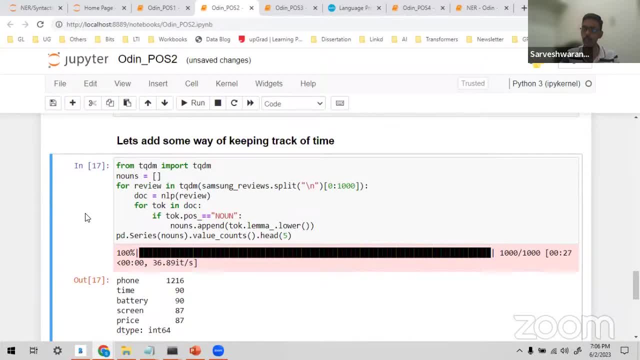 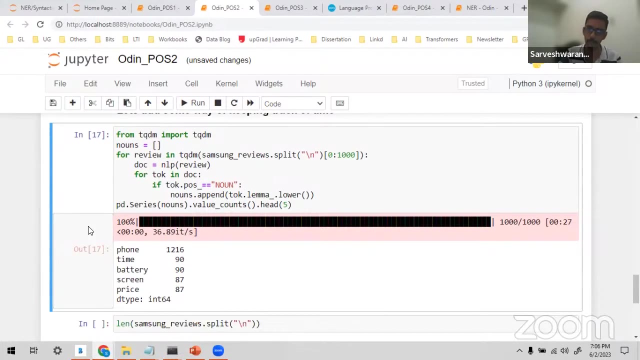 where you can make use of the higher configuration systems. you don't have to necessarily invest in a new hardware. make use of the cloud platforms. there are many uh cloud platforms nowadays, right, so you can make use of your very famous google collab group. very simple, very cheap and 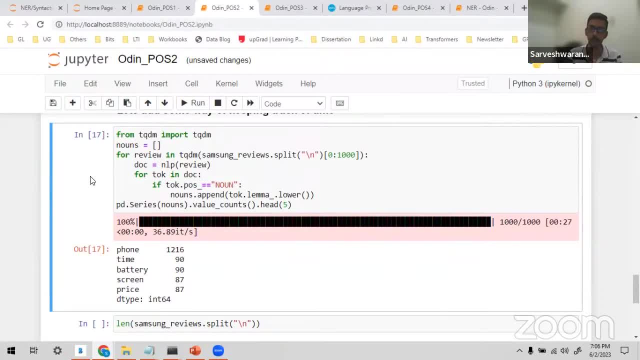 there are some disadvantages, you know we can keep arguing in it, but if you are in beginner, if you are learning right, so you can make. you can start making use of your google collab, okay, so, and then you can see. so the part of speech tag is now right. so which are the words for the? 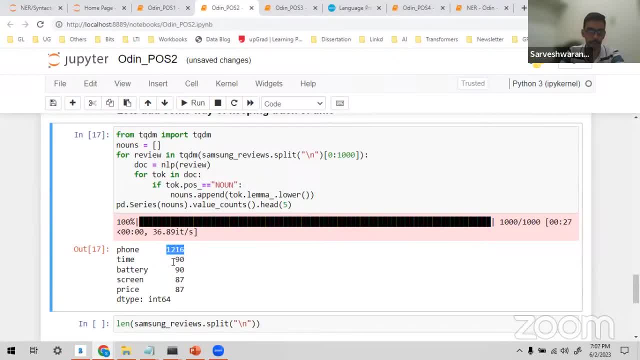 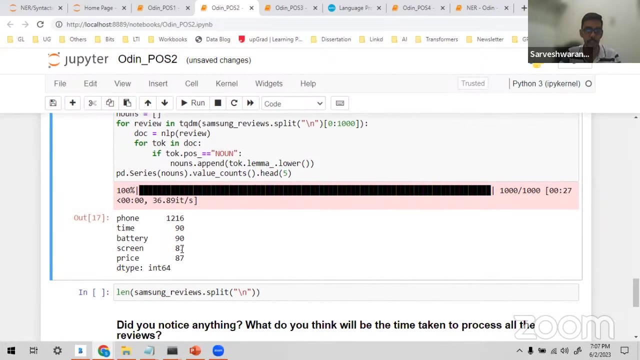 thousand uh sentences. the phone is the highest used time, battery, screen and price. this is what people are speaking, more in your feedback, right? so the moment i understand this, what is that my people are speaking about? i can make some informed decisions. the extension to it, like i said in sentiment. 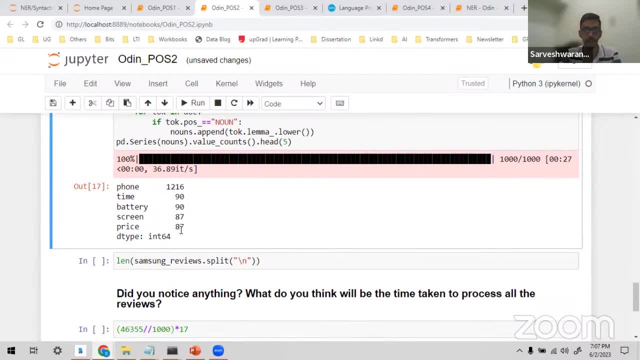 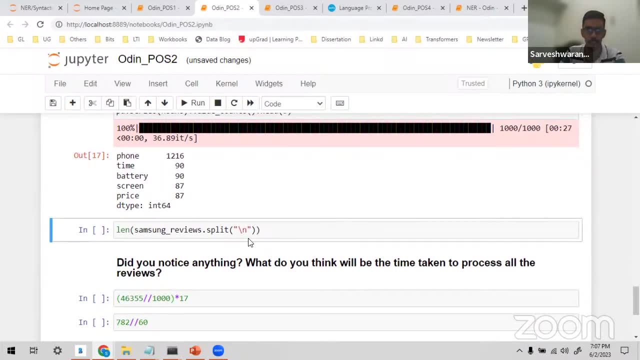 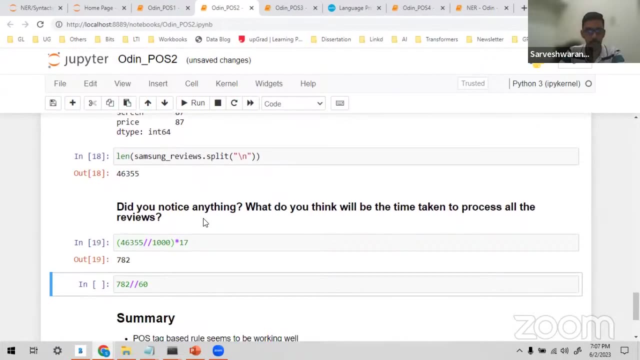 and the sentiment analysis, right. automatic ticket routing: there are a lot of applications so i can convert to in workload. it isn't small experimental show, a small demo that i can show it, and right. so? so what will be, uh, the time to process all these reviews, right, so that's what. so it has. 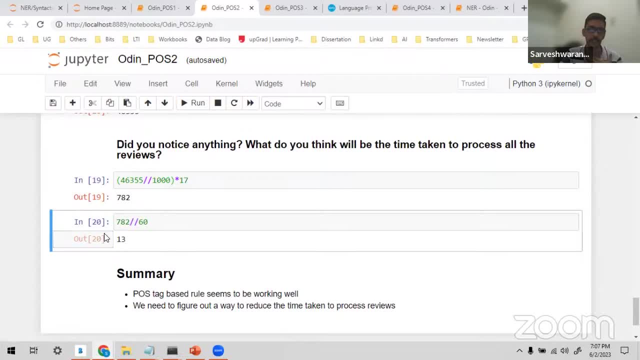 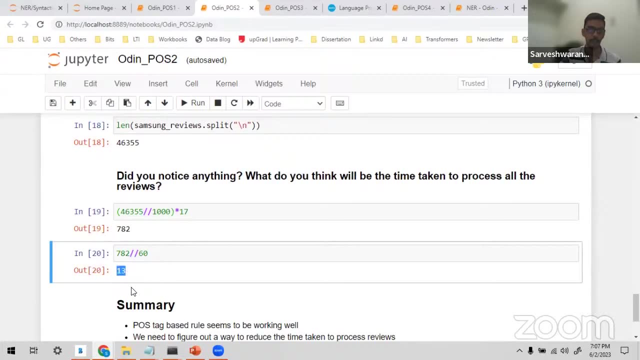 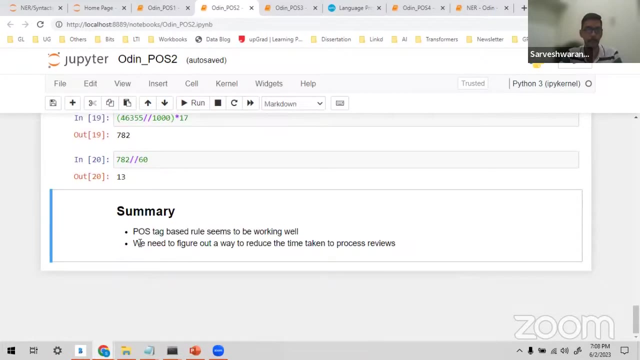 taken so long. right, it will take a bit more, right uh, to process all these reviews. it is taking a lot more time, you can see um it to uh to do um this, uh, the review processing. it takes much more than more, much more time, right? so the summary part. 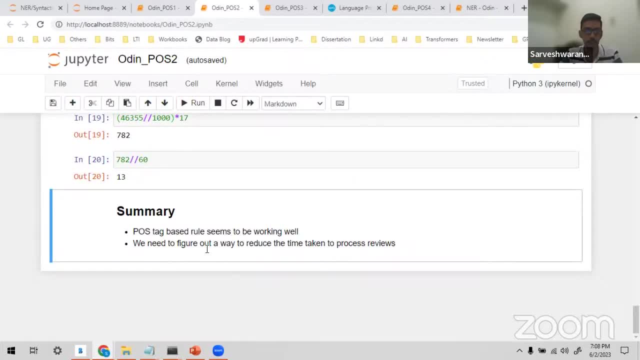 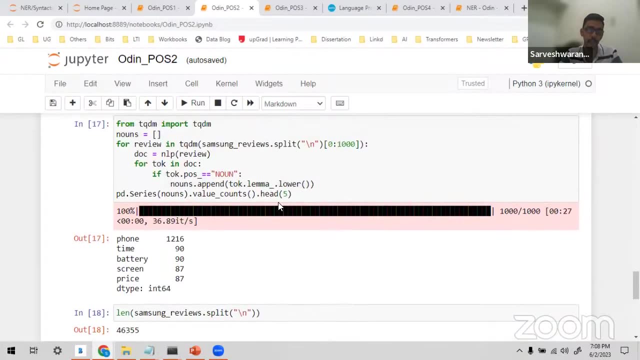 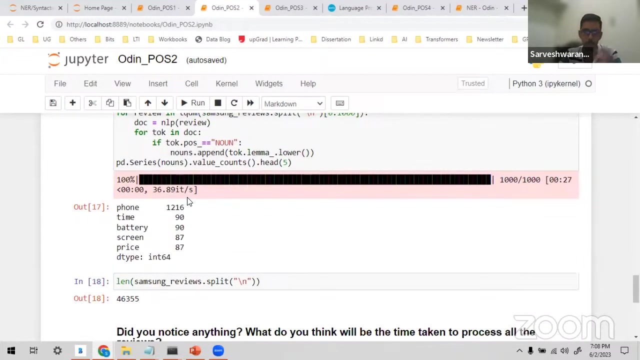 of speech. tag based rule. uh seems to work well, but we need to figure out a way to reduce the time taking process. so this is one time consuming way of doing it a bit uh, and back to all the old school ways of doing it. now we have very bit more advanced ways of doing it. let's see. 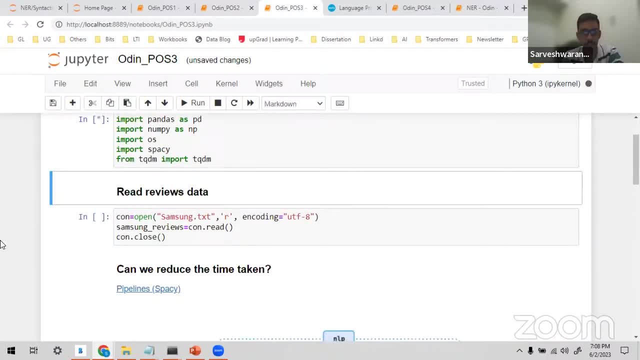 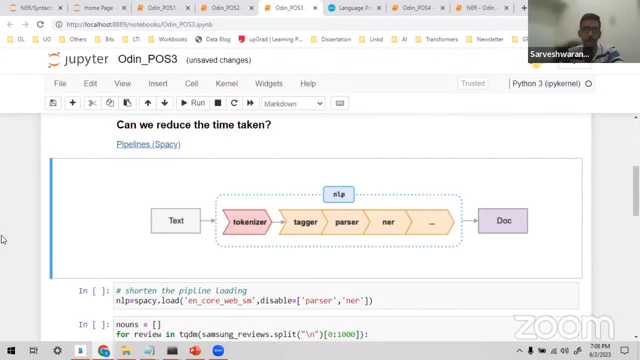 so another example i have taken. so i have taken a samsung data, the same thing. how can we reduce it? very famous example- uh, very famous library, is your spacing. i've used this same spacey library to do the entity recognition or the entity extraction from all the different receipts. 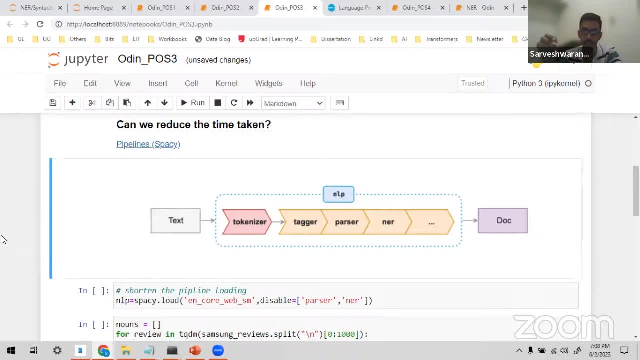 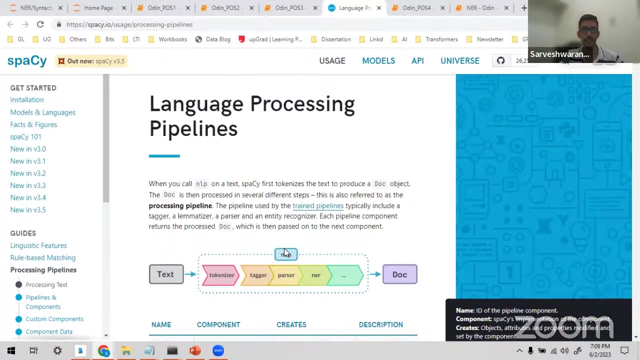 i give the text, i tokenize it, tagged parser, named entity recognition, right, all this and it's converted and this is the pipeline here you can see. i just all these are taken from here, right from the spacey you can see the text, the tokenizer and the. the specie 3.0 was. 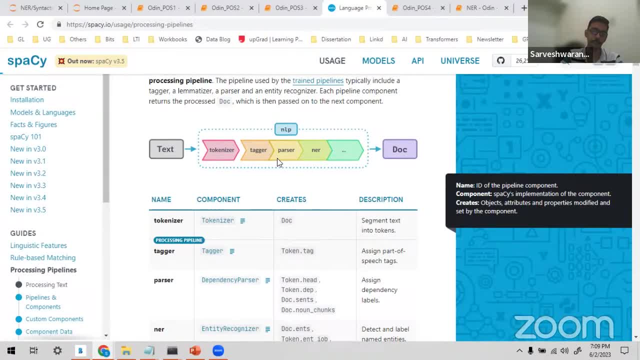 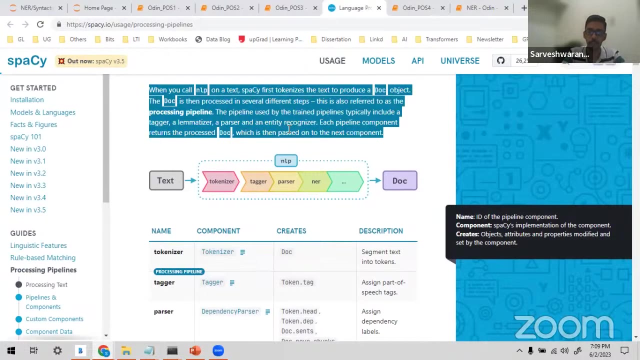 very famous. now you can see there is a new version of spacing right. just just just understood understanding this PC And by making use of this pre trained model, you can. you can fulfill most of the low hanging fruits in the market. You can have so many different applications. 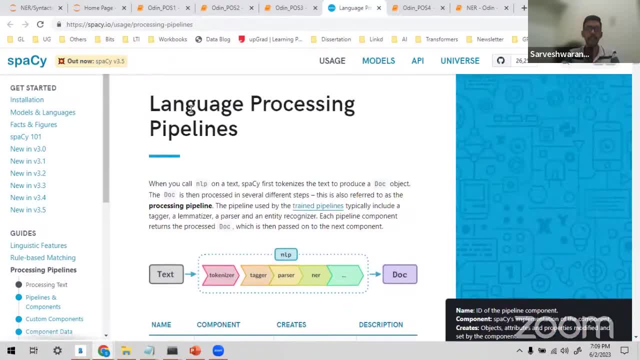 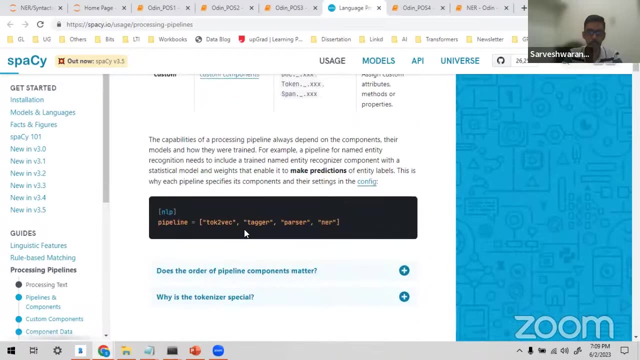 using the same space. Just go through this PC. Very fantastic library. I'm not promoting it, but I realized it by using it myself, Right? So you can see. so what? all it's very simple, right? so you can go here and you can select what is the pipeline that you want to talk. 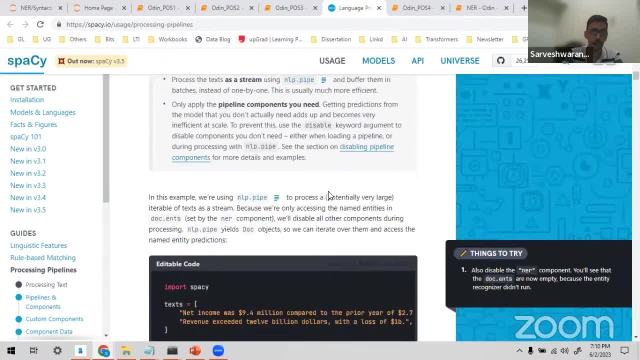 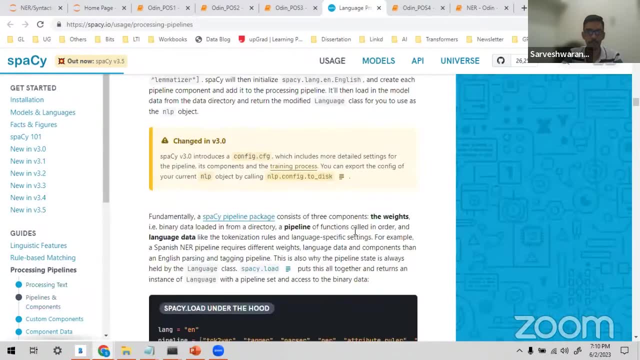 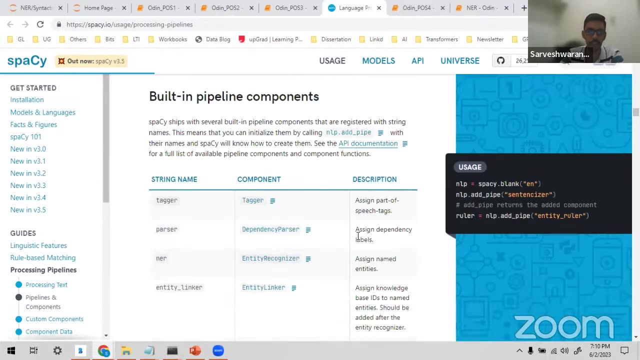 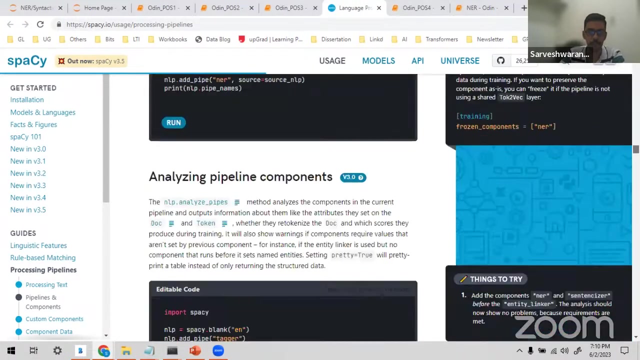 into a tagger password, So you can go here and you can download. So okay, so you can configure here and you can download the file. you can download the config file right away. I'll show you at last. I have the downloaded config file. I'm not getting it right now. 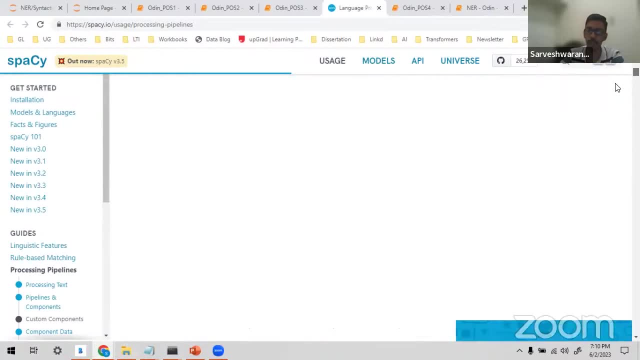 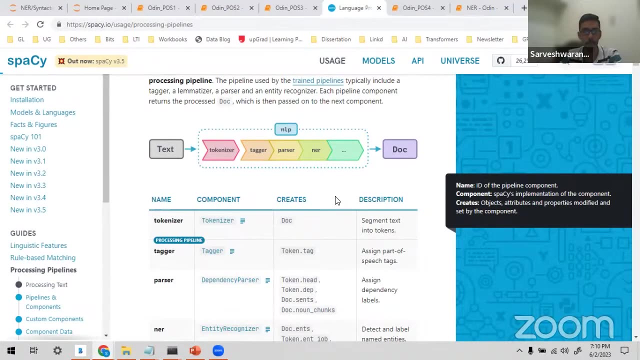 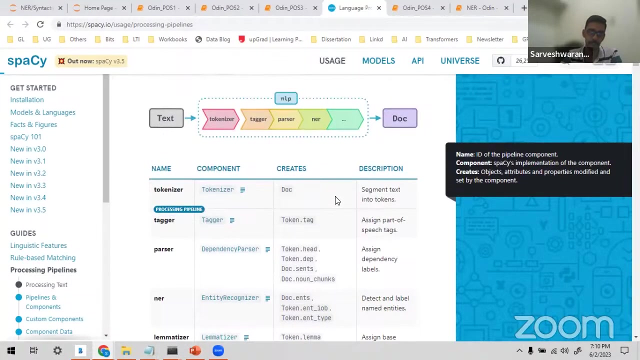 But I have the downloaded config file. I'll show you how the config file will be. like you are do the hyper parameter tuning, how you pass the values to the model. So all these things can be done in the config file and you can load the config file directly, Right, 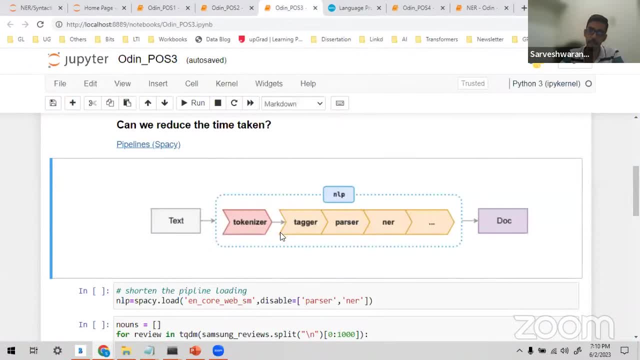 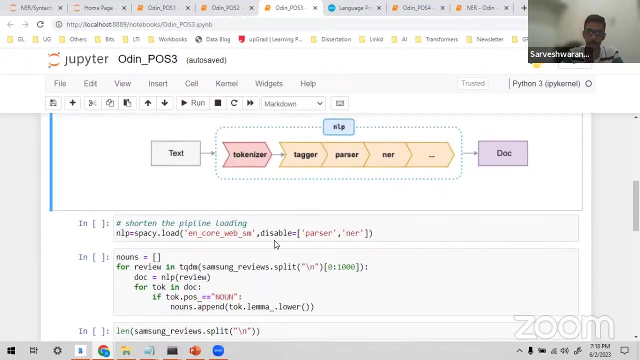 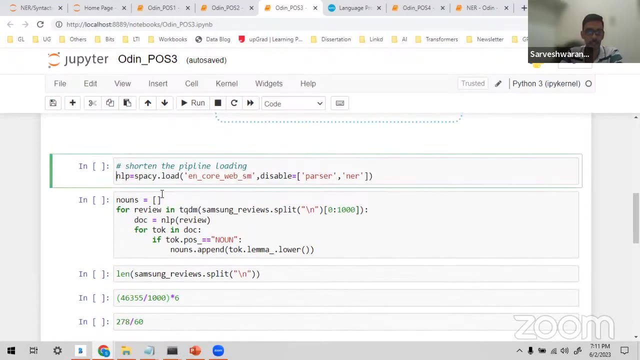 And you can also do in custom based in here. If you do not want to make use of the pre trained model And you want to custom train the model, you can take the pre trained model, encode that SM right so and you can do and custom in the air here. Okay, so that is one thing that you can explore. So I load. 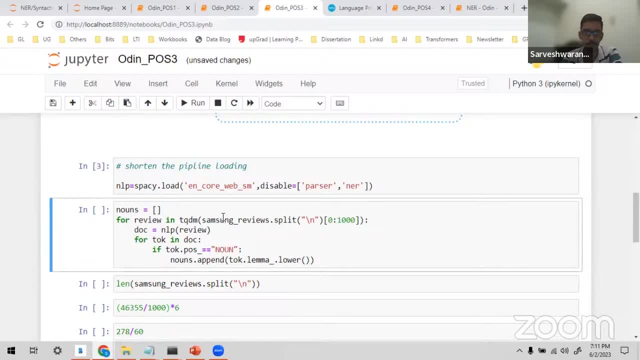 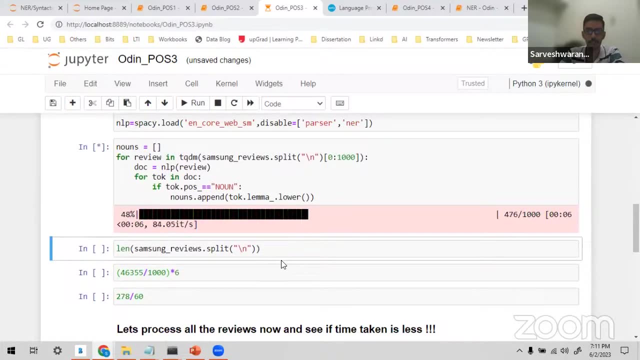 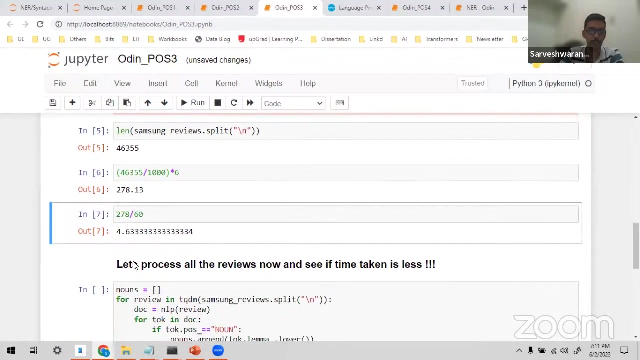 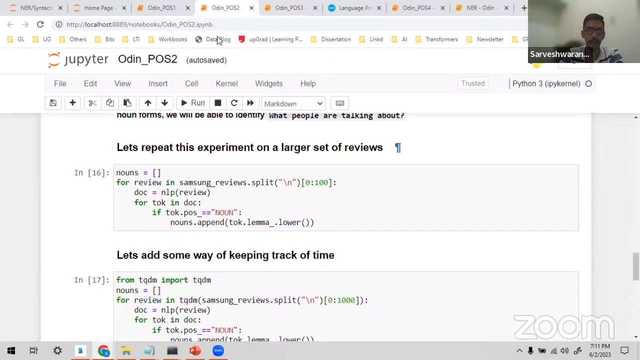 this model in code with SM right and you can see it's bit more faster and see the time consumption- 27. Okay, so we're using in So so the time consumption you can see. so it's far more less time consuming than your traditional way of doing it and you're going to use some. 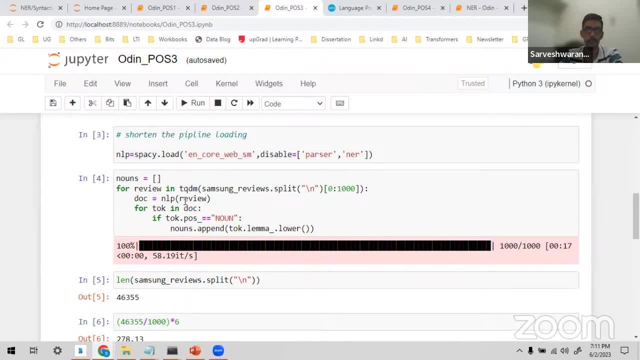 spacey like this. It's short on the pipeline loading. Okay, so you don't have to use a lot of time. So you don't have to use a lot of time. Okay, so you don't have to use a lot of time. 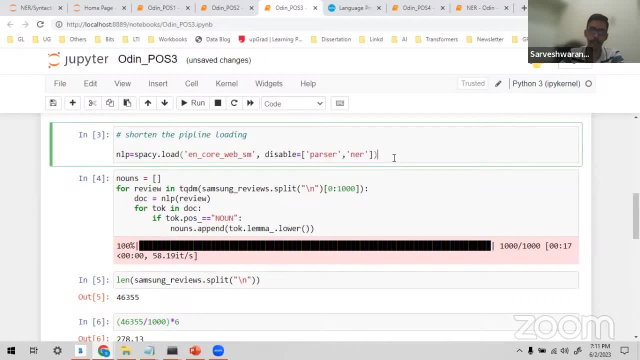 Okay, so you don't have to use a lot of time. Okay, so you don't have to use a lot of time. You're going to be able to use the parser or an NIR. you just disable this to read. just by disabling this two, you can save a lot of time. 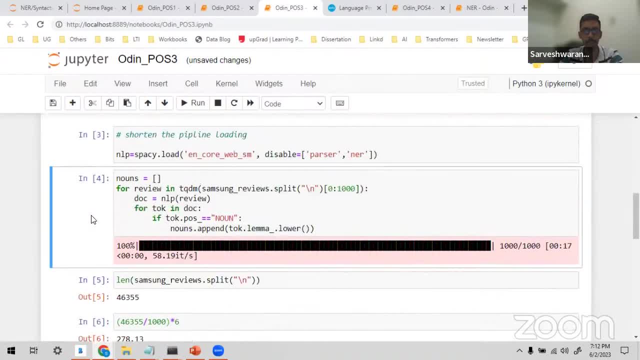 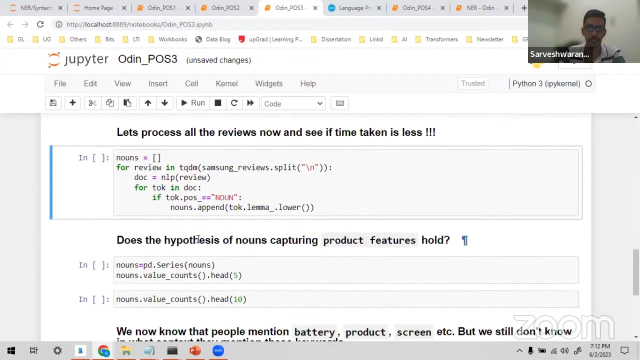 By using an encoder. so this one simple thing. all this comes from experience, right? so I'm just giving it right away, right, if you just disabling this a couple of parameters here, so you can save a lot of time. So let's process all these reviews And, yeah, it takes much. 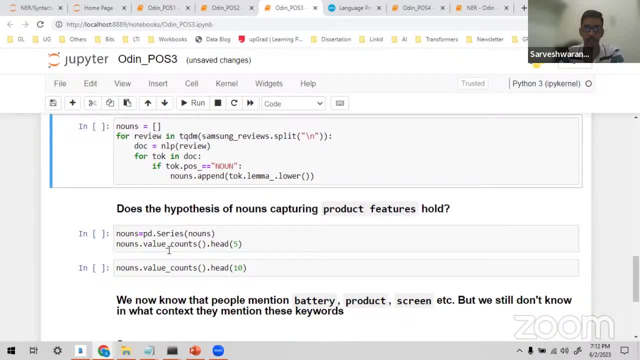 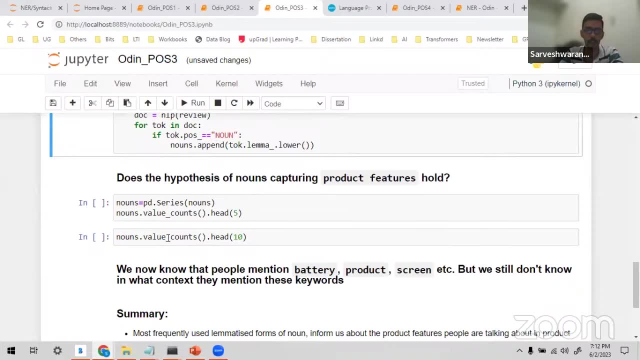 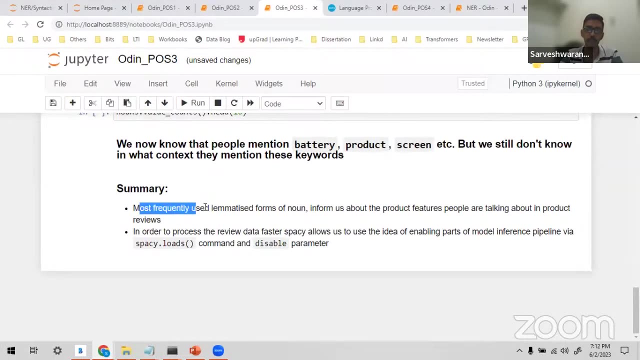 more time, do it, but uh, but definitely by uh disabling these two, uh, you can save a lot of time here, right? so, and i can also do an analysis. what is battery product screen? how many? how much number of times it has used most frequently used lemmatized words of noun. inform us about. 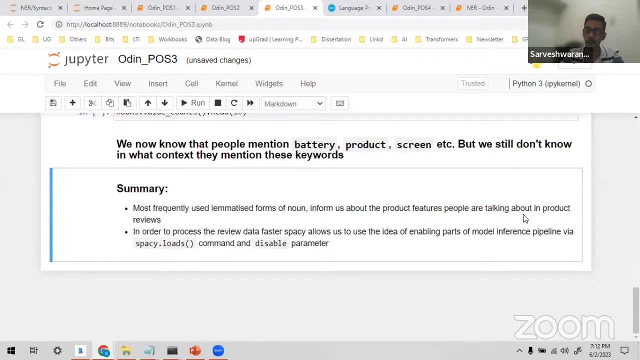 the product features- uh, people are talking about in the product, right? so there is different way when you write in feedback. it's not proper grammar, right? we write whatever we want to write, exactly right. so i want to do the pre-processing so that i make all the feedbacks in a uniform way, right? 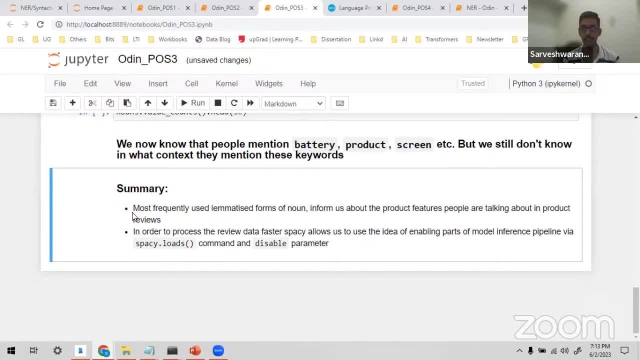 i write it in my own way, my own slang, right. the people in us write in their own slang, the people in uk, they write in their own slang right. so these products are, uh, having an international market right. so i need to convert them to the root form. normalize, right. you do the, the normalization in the numbers. 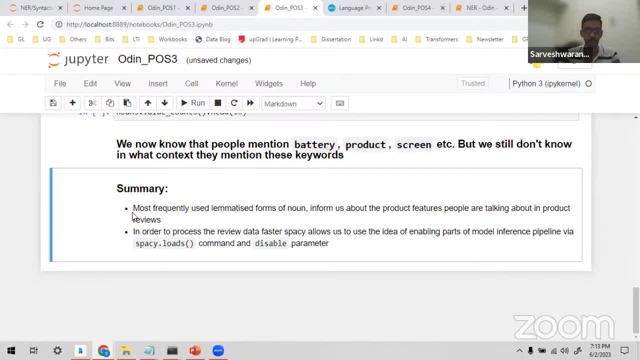 similarly, you do the normalization for the text right. so, in order to process the reviews uh data faster, allows us the uh idea of enabling the model inferencing pipeline using the spacey loads command and and disable some parameters like issue. i'll also show you a very interesting 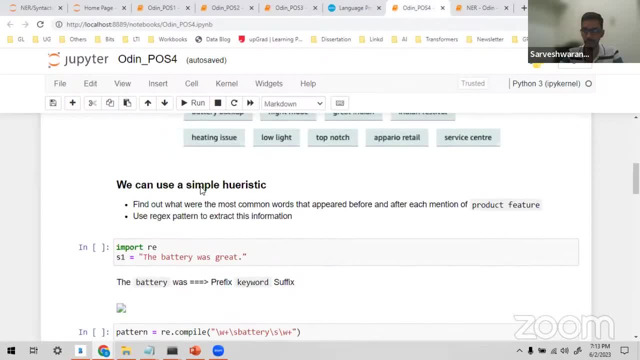 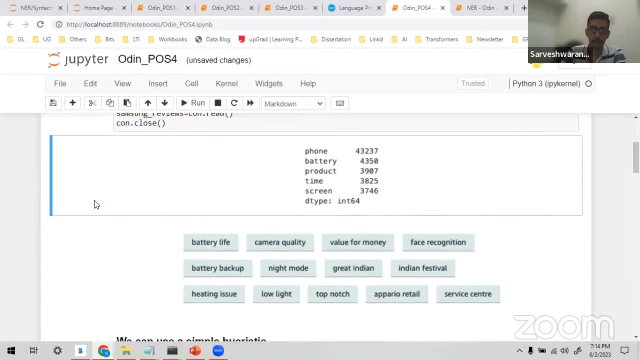 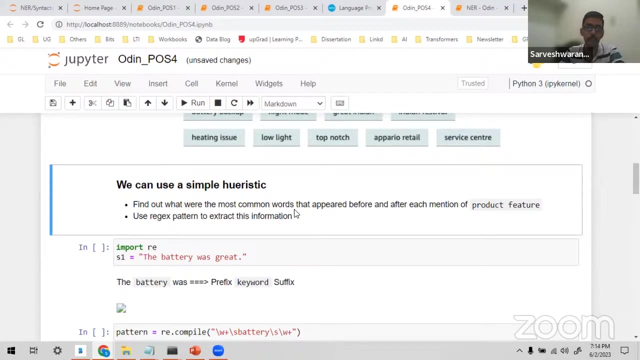 example in shortly. they have very less time, but anyway i'll show you. you read the data again. another example here. okay, what is that people are speaking more? so we can use in simple heuristic: find out where the most common words that appear before and after each mention of the product. 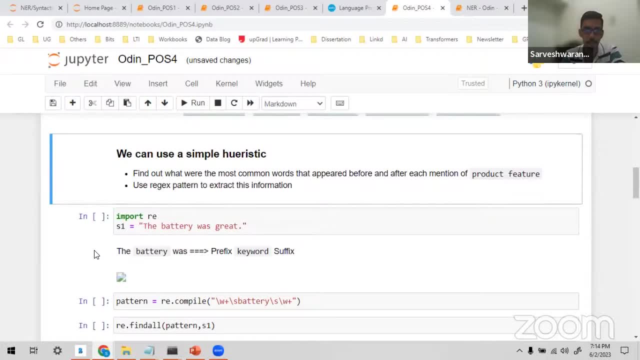 feature. so we use a rejects pattern to extract the information, right? so how do you use that rejects pattern, right so? uh, yeah, maybe i can go explaining. so the rejects pattern. you have five important functions: match, find, uh, the match, the search. we find all. we find. iter, your substitute. so these are the five different famous functions that we use. i'm 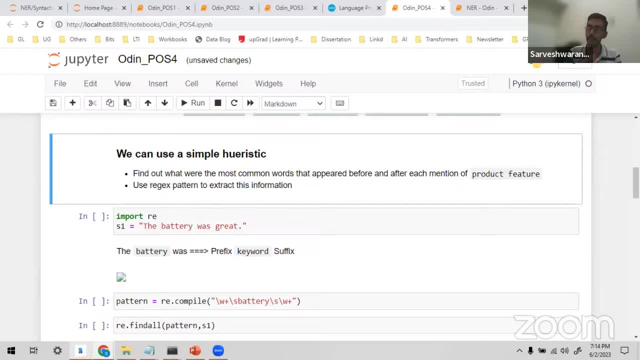 using famous uh, the, the five quantifiers, the question mark, the star, the plus and the mn operators. So these are the different quantifiers that we use. So, basis of all this regex patterns will be able to extract in, so extract the information from the text. 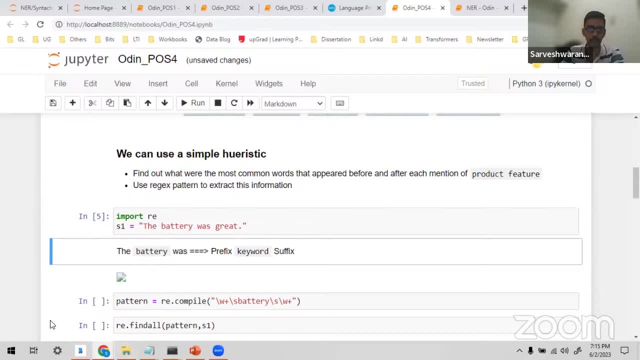 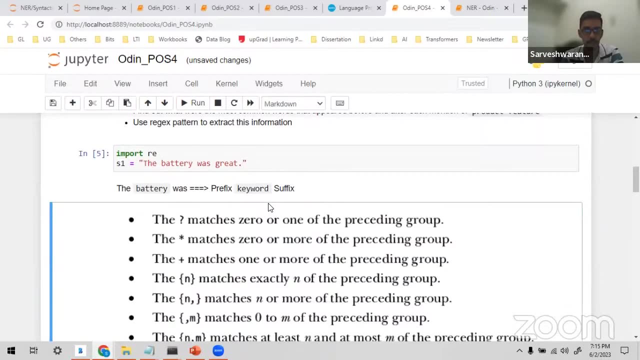 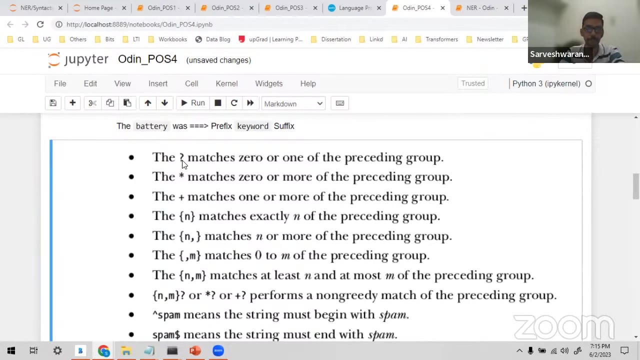 Battery was great, Right, So the battery was great. The prefix keyword suffix, Right, So yeah, so this are the different quantifiers. So what is a quantifier? Question mark: the entity the last keyword matches that the preceding character matches. 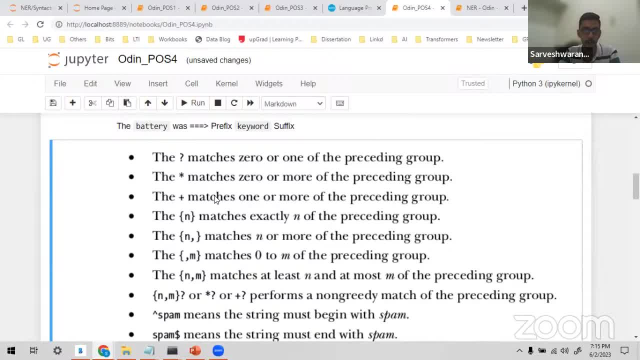 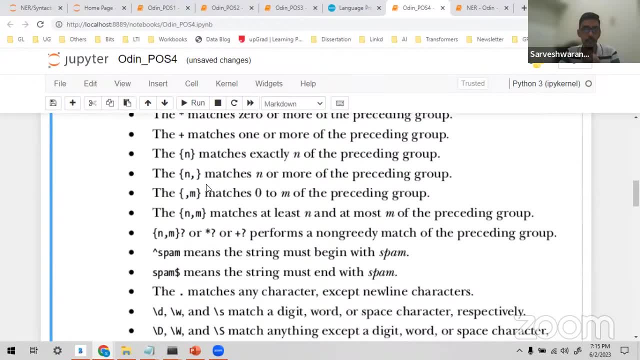 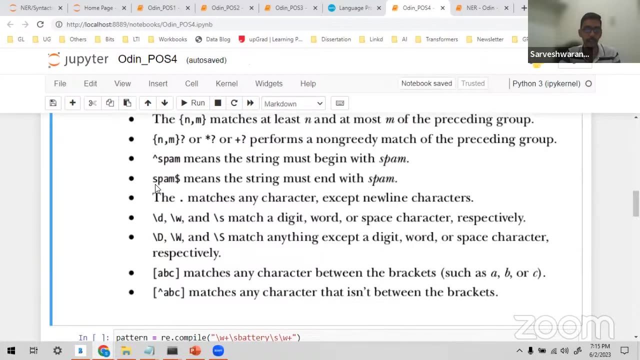 zero or one of the preceding group, the star matches zero or more of the preceding group, plus matches zero or more of the preceding group. Right, So again, MN quantifiers. So these are the different quantifier, that is, for example, and write so again, the wildcards, the anchors, bit advanced, and 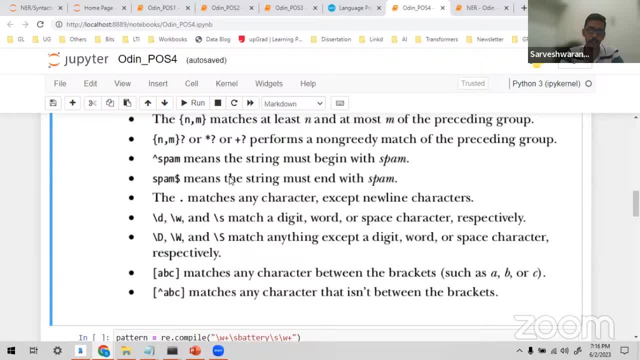 the rejects if I'm using an exponential mark here. So the string must begin with use and dollars in a class is spring. the string must invent and write. So these are the different quantifiers. So again in the quantifier dot sagen fmg lemma quantif��요. So these are the 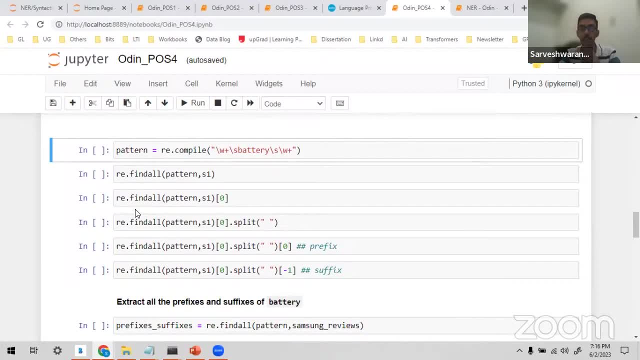 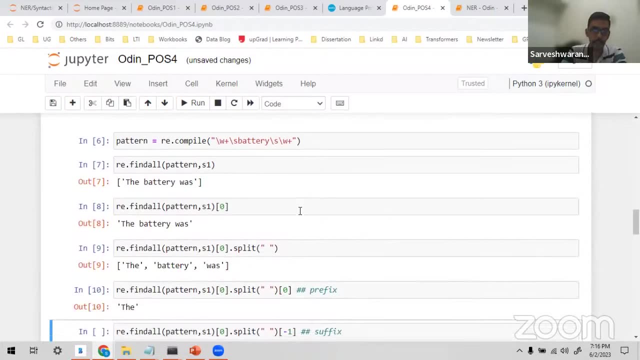 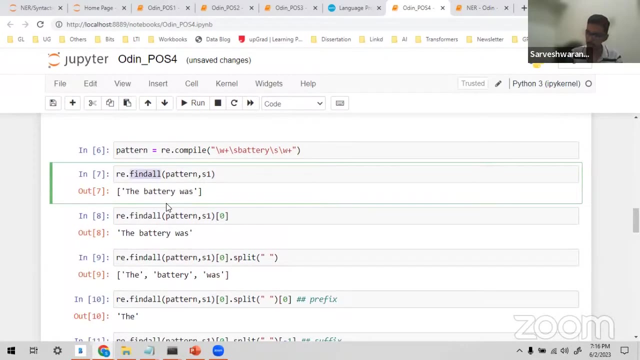 quantifiers on the while cards on the anchors here. okay, so see again here i can use. so here i'm using in regex based way of doing it. now see here i'm using in find all function. so out of five different functions i mentioned, match, search, find all, find data and substitute. 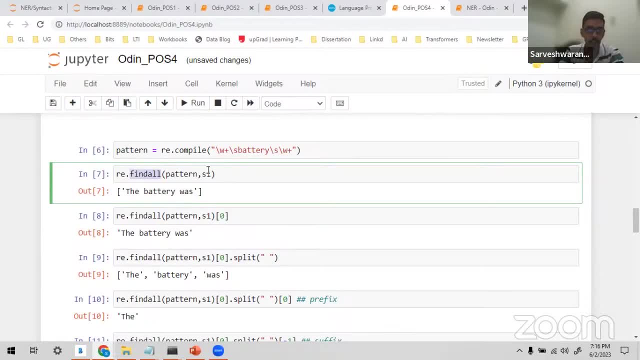 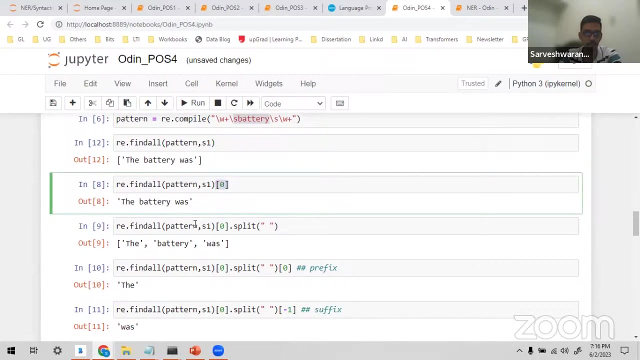 in that i'm using in find all function. so what is that function doing? it has some pattern. i have a pattern right. so on basis of that pattern i'm identifying what are the important words with respect to battery. is there the battery was. so in the first review i'm taking 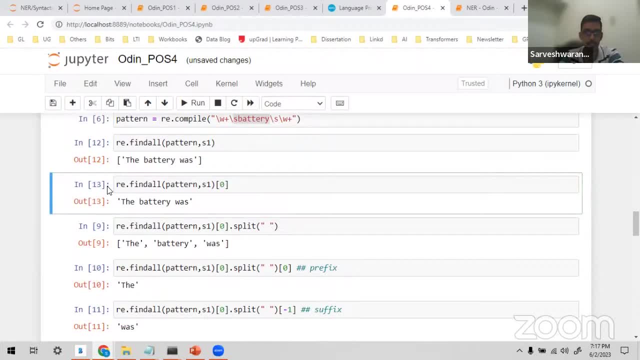 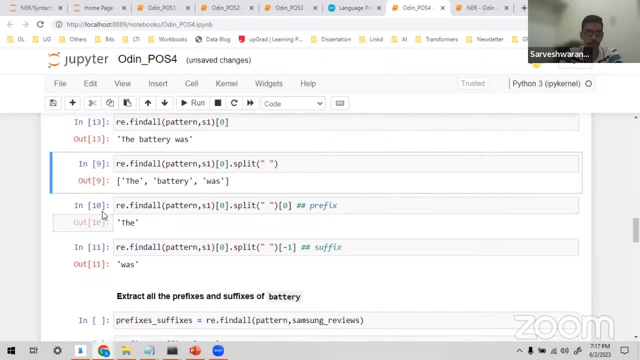 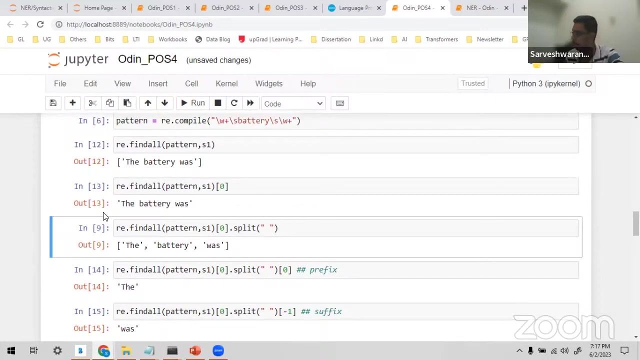 the pattern the battery was and i'm checking for, uh, the number of times it is present. okay, and i'm just taking the prefix of the word battery and i'm taking in suffix of the word. but right, so you can see how i can play around with the text. so i can do a lot of things. 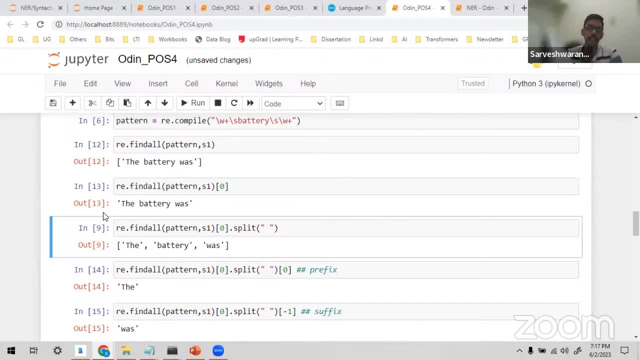 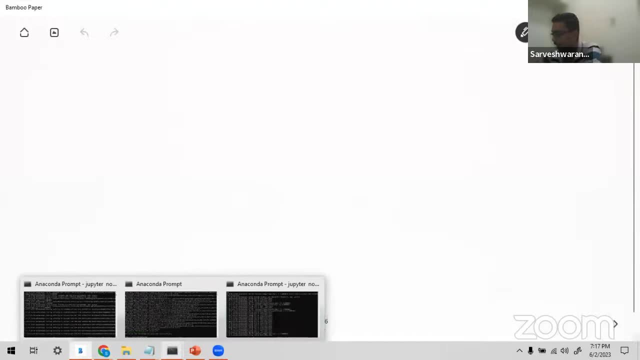 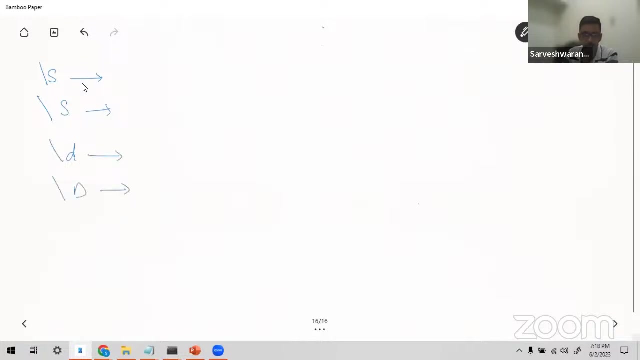 with this text, right so? so these, all these things are called some meta sequences, right? so the meta sequences goes like this, right, say, say, for example: so, so, so, so, yeah, so, uh, so again you have a lot of meta sequences, yes, and and capital s, again here, small s, capital s, slash d, slash capital d. 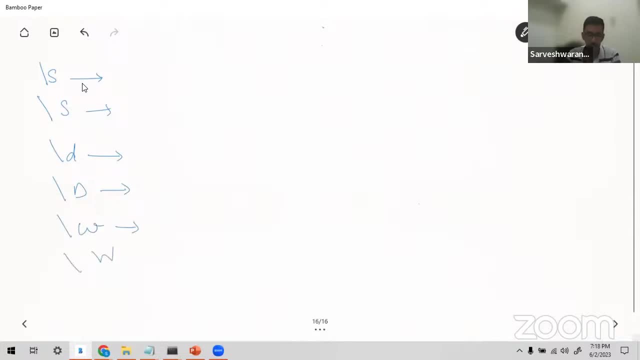 slash w slash, capital w right, so, so, yeah, so here's a little journalists, right? first thing is that, if you, 你们要想看今天的这个圈中, if there is any white space present, right, if there is any white space present, white space. 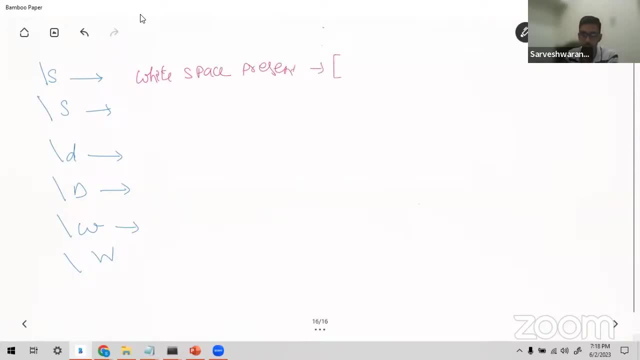 that is present, or in other words, right. so if you are going to use in backslash the escape sequences, you will use an escape sequence t, escape sequence n, escape sequence r, f and v, right. so once you start learning this regex, so we have in short form for all these uh regex. we see that our target range is like z right and z is like z right and z is also z right and z is also z right, because we don't know whether this is working or not. we don't know because we don't know whether this is working or not, and so the way that we've created these- 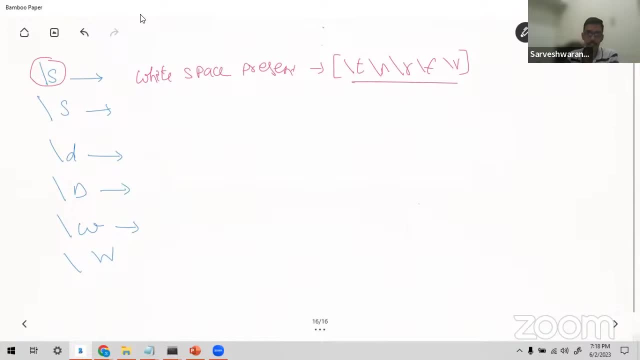 search modules. which are these search modules we are going to use these search modules to, in short form, for all these rejects. we convert these to a meta sequence. If there is a wide space present, I use an slash S. I use capital slash and the escape sequence and an S the 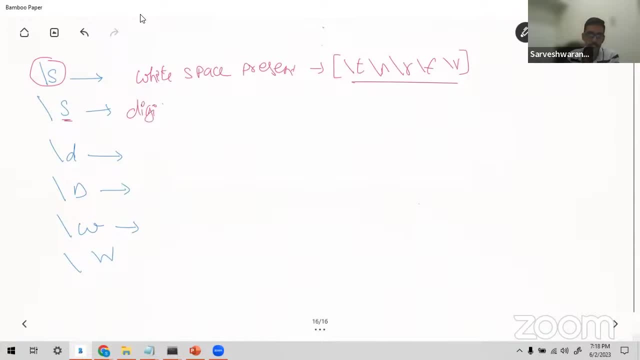 capital. S is to search when there is an. if there is any digit present, I want to extract the digit that is present If there is any alphanumeric, alphanumeric sequences, if there is an inverse set of alphanumeric. So these are some shortcuts. you call it as a meta. 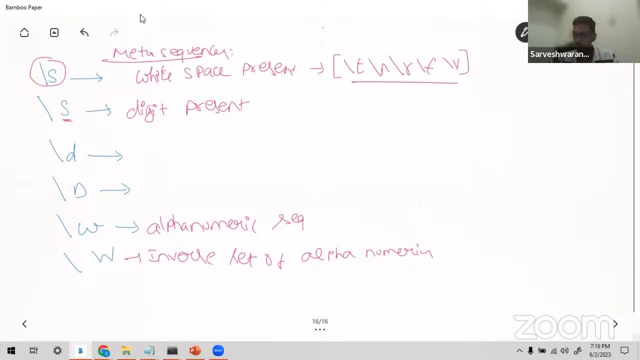 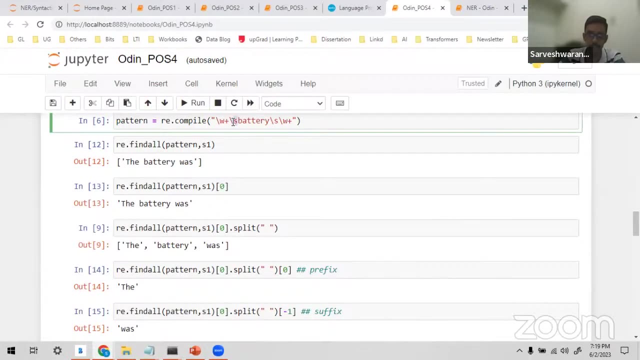 sequences. So these are some shortcuts. you call it as a meta sequences, So this gets too technical. So at an high level I am just using an slash, S and and small w the alphanumeric sequence and if there is a wide space present, like I mentioned. 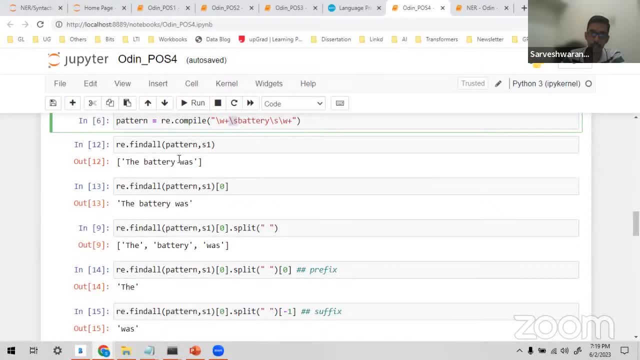 w the alphanumeric sequence and white space present, so it identifies the prefix and suffix of the word when there is a wide space present and an alphanumeric character. the alphanumeric sequence: right, Wow, Okay, Okay, Okay, Okay. So any text that you give, I can extract the useful information using the regex rules. 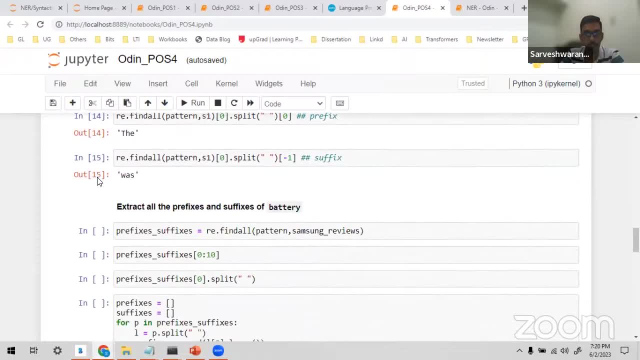 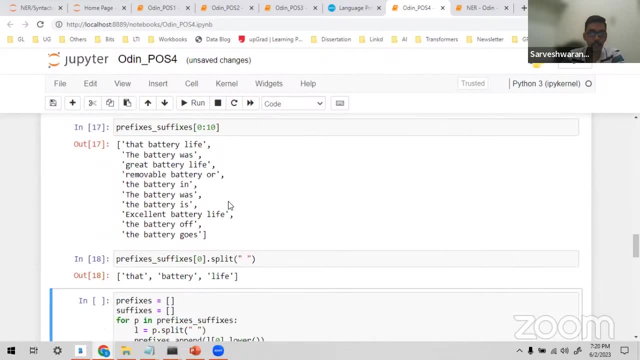 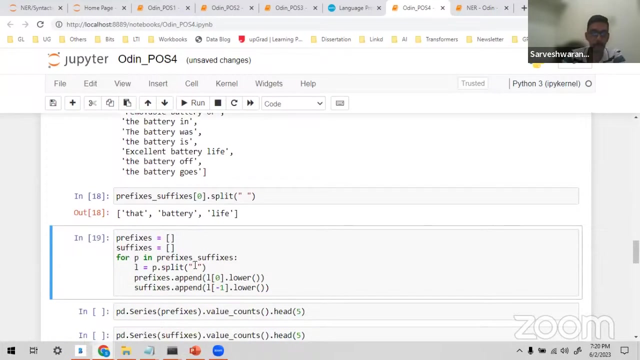 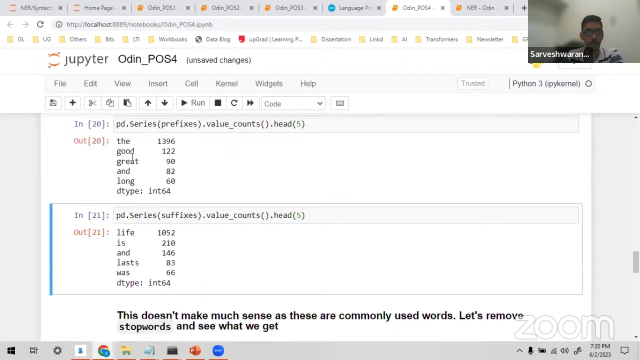 These are all rule-based Extract, all the prefixes and suffixes of battery. So these are the different places where battery is used. that battery life, the battery was great battery life, removable battery power. So I extract the prefix and suffix. so for every word where the battery is used, I extract. 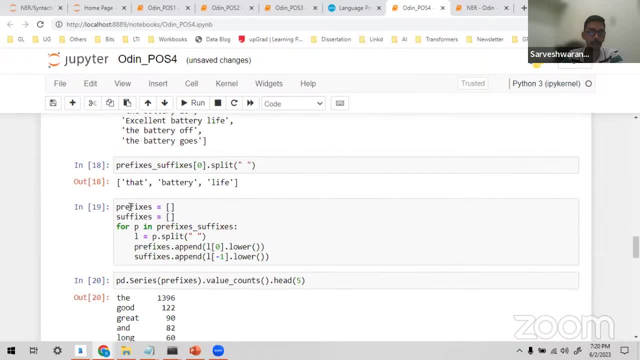 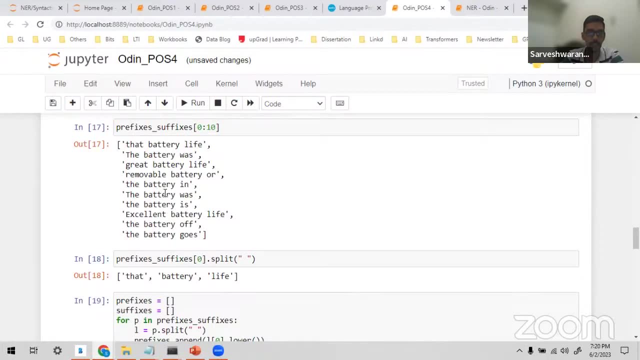 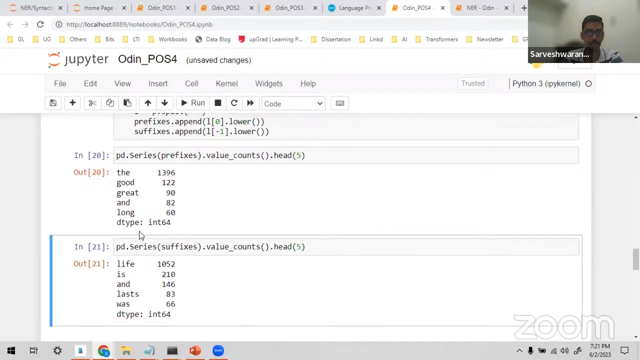 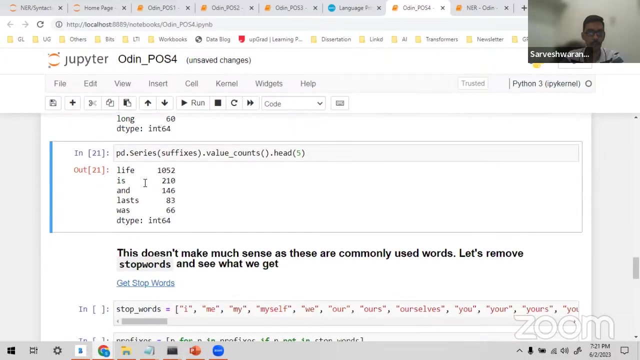 the prefixes the good great long. you can see the long battery somewhere. it was present, where it is, I have just taken few of it here. it is that battery life, removable battery life. you can see life. and yeah, so all the prefixes and suffixes are stored. 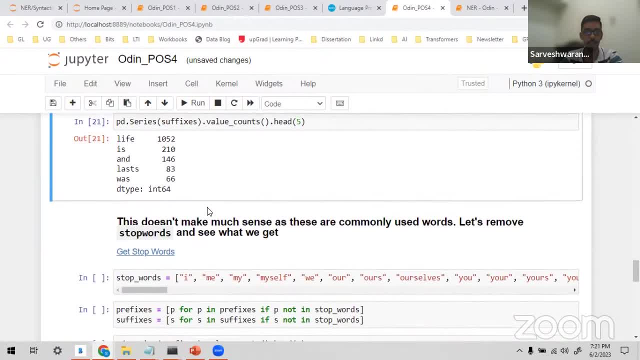 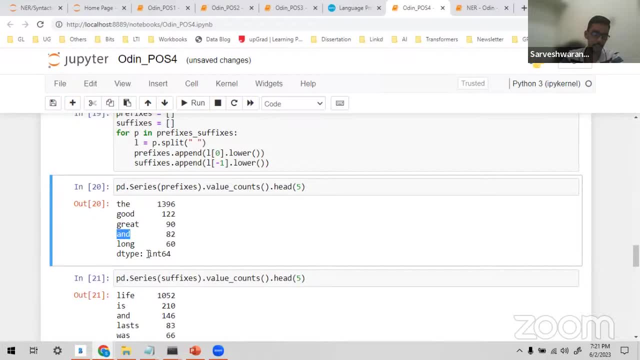 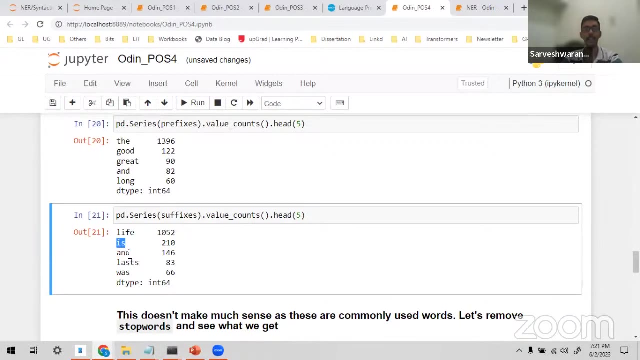 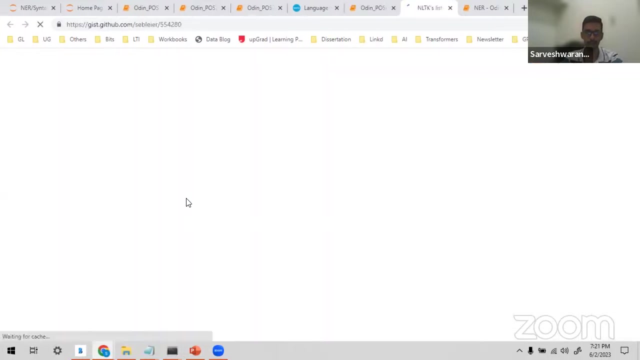 here. I am just taking few of it, just five of it. right Now you can see the and there are. yes, so these are all some verb, these are all connectors. These are some grammatical connectors, So these are often called as some stop words. I do not want to use the stop words, okay. 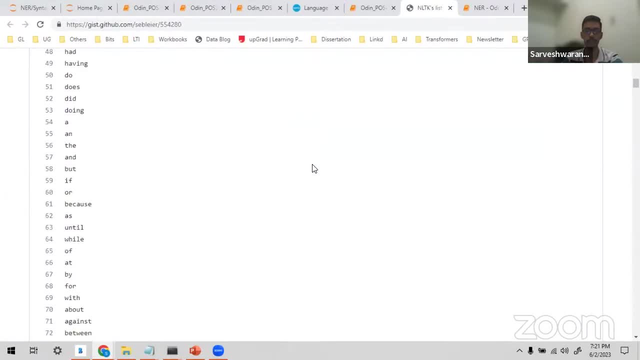 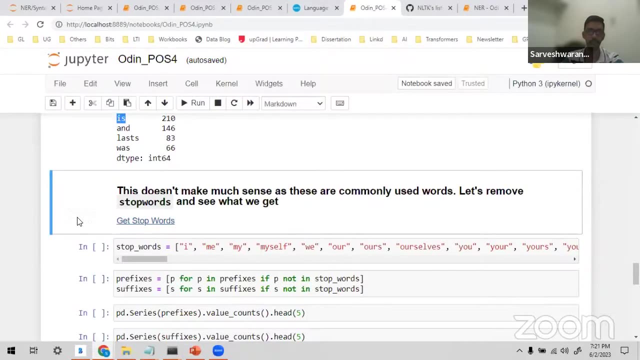 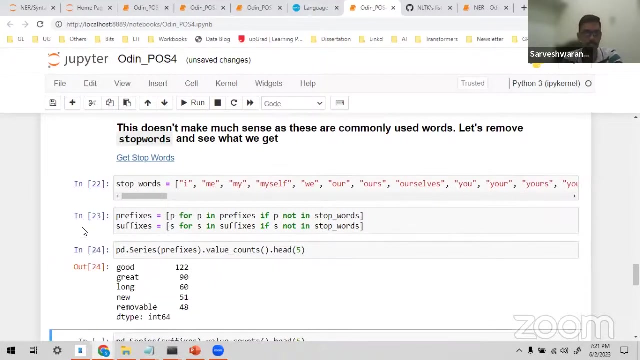 I can delete the stop words. I need to remove the stop words, right? so these are all the stop words. So there are stop words library. again, from the stop words library you can download the, you can use the stop words and you can remove the stop words, the prefix and suffix. I just 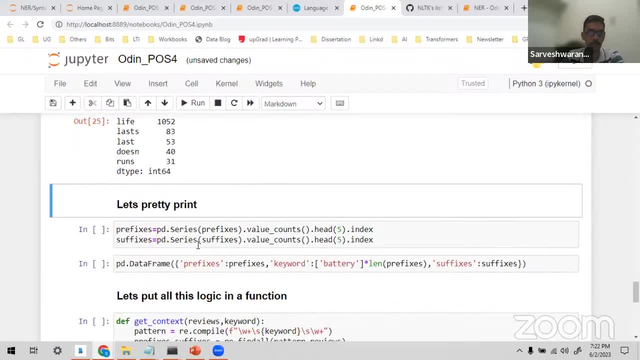 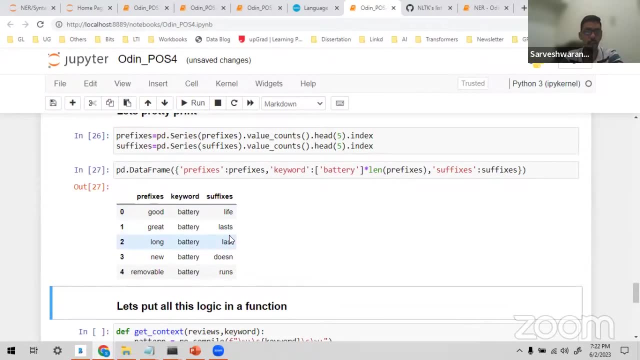 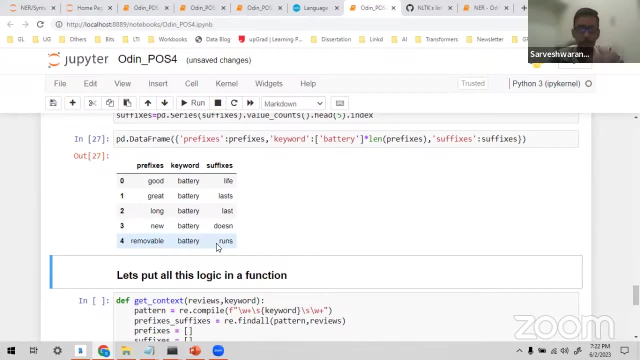 remove the stop words and you can see Now what does that the battery say? good battery life, great battery lasts longer battery lasts. new battery does not removable. battery runs. so we can extract some useful information. What are they speaking about? my key entity, my key entity here is the battery. what are 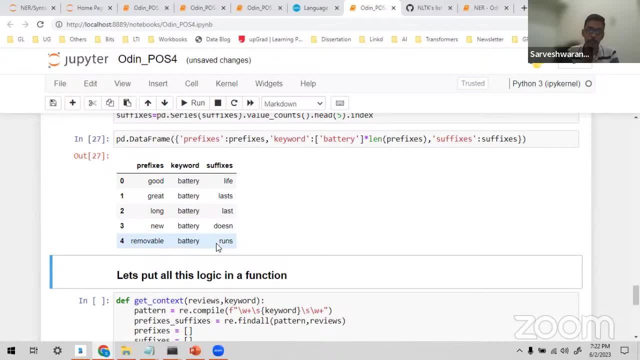 they speaking about my battery: good battery life, great battery lasts. so they are giving some positive words. they are giving something, some, some useful information out of all these feedbacks. first, I extracted the key word battery and I am giving in prefix and suffix. 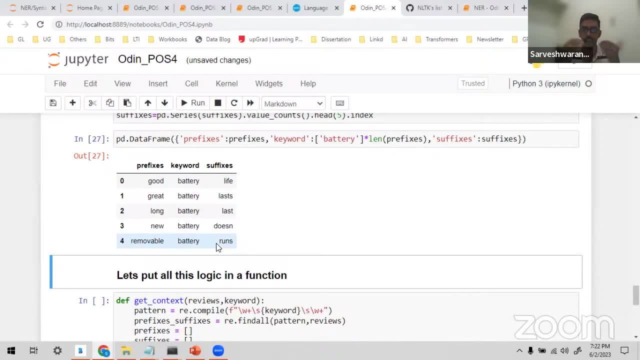 for that battery and as an user, as an analyst, it gives me a very good insight. what are they speaking about? my battery? I can make use of this regex and I can do this, So I am giving some positive words. they are giving some useful information out of 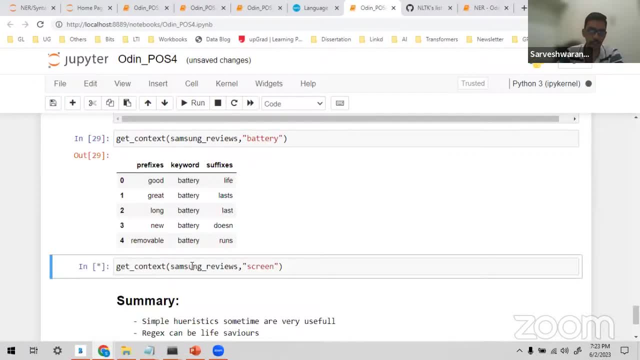 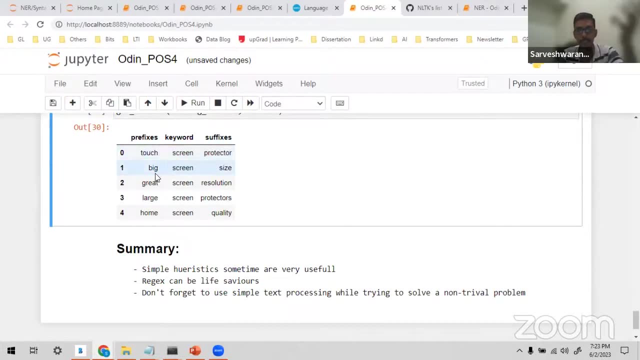 this. I can do the similar thing for your screen, right? so screen touch protector, big screen size, great screen resolution, something they are appreciating. larger screen protectors, home screen quality. So they are with I have just made. I have not got too detail, I mean too involved analysis. 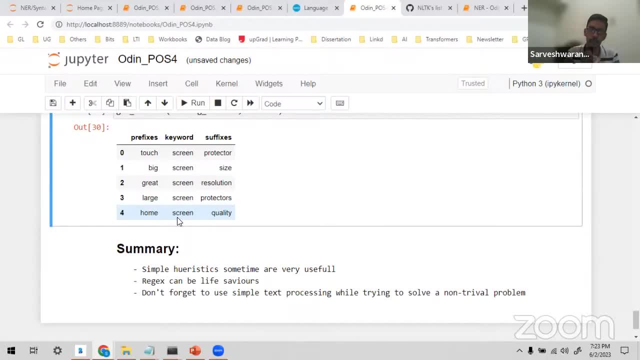 just in basic. I am just basing on the low hanging fruit. Just by taking the prefix and suffix of my key words, the key entities, the battery and screen, see how big you are getting some insights from the feedback As some take away, you download the tweets from the tweeter or you take your Amazon feed. 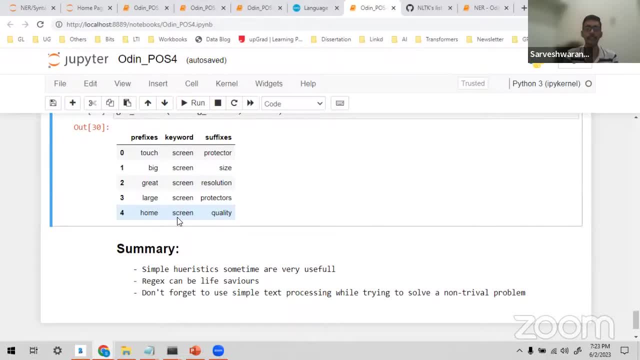 or the product feedbacks, and you do in similar analysis, just by taking few, two or three steps into the product feedback. Okay, So if you are using the regex and your spaCy, we have achieved something and one step towards your sentiment analysis right. 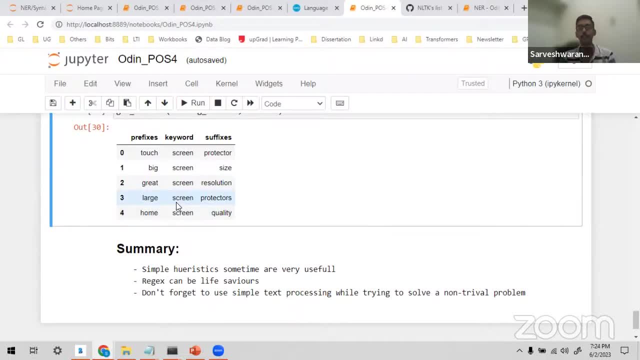 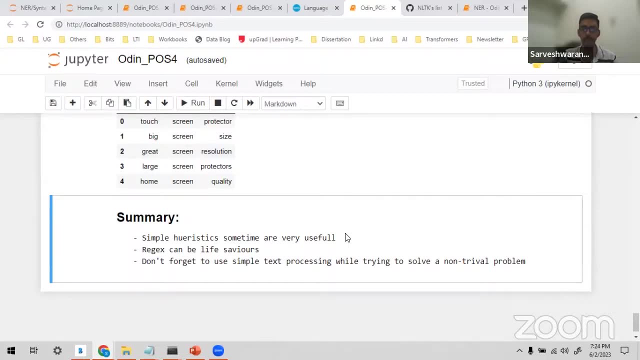 I am not saying this is all, but at least we have taken one step forward than the raw text that we were seeing right. So some very simple heuristics sometimes are very useful. I have done very simple. Regex can be life-saving. 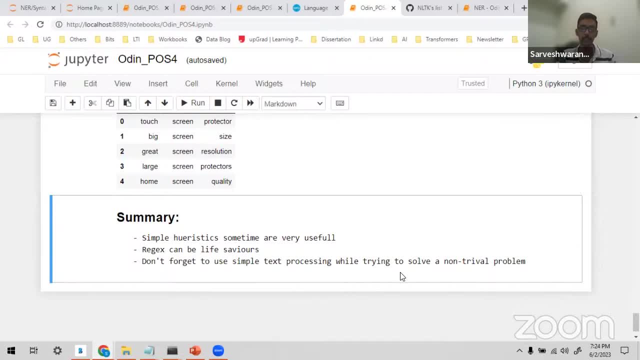 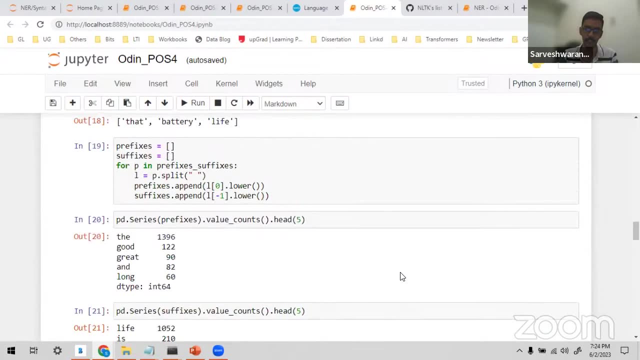 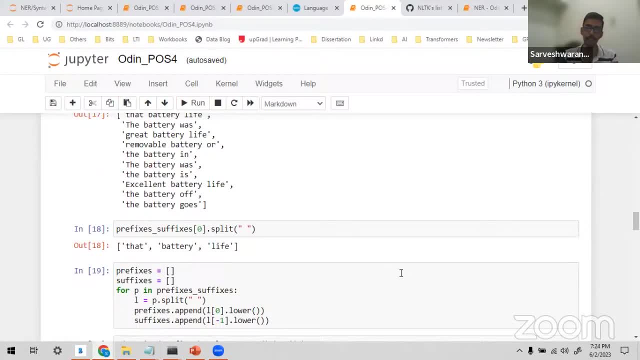 So, after the rise of all these GPT models, so this text has been the area of focus for all industry leaders. nowadays, Right, Basic text pre-processing- even in basic text pre-processing is not done in various different industries, Right? So if you could have taken stepping of a spoke in your organization, half text if. 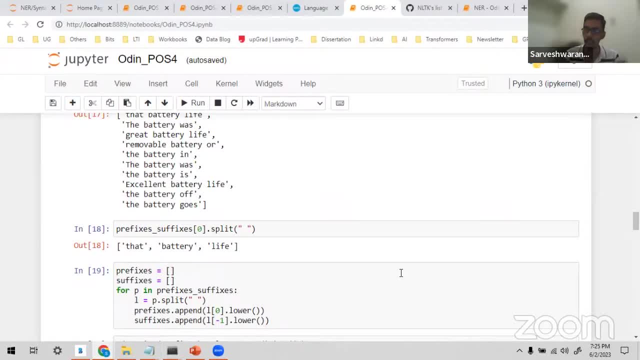 If you have log, let's say, for example, all the logs, all the programs, all the applications that we have in log files. take the log file, do basic the text processing, put it in a dashboard. Hardly takes, maybe for while you're learning it takes much time. 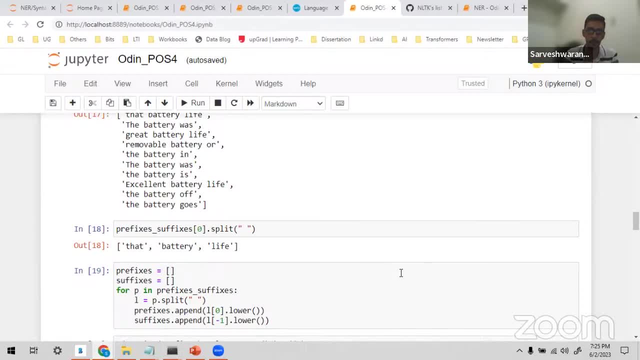 But once you have learned it's hardly one or two day job. it can amuse your clients. So that's the power of the MLP, the basic text. preprocessing The Gen A is a different thing altogether, the GPT stuff, But again, so the basic heuristic, the simple heuristics can do the magic. 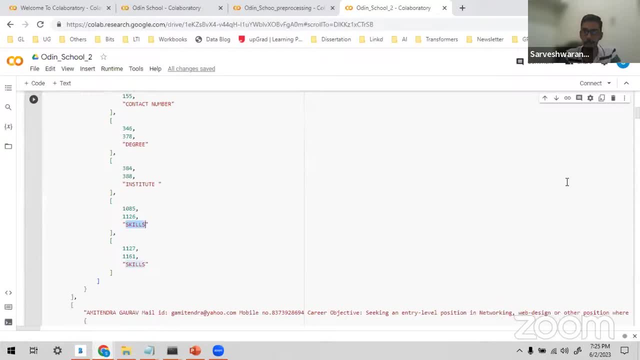 And let me simply go through the resume shortlisting what we have done. We have taken all the different entities and given the starting and end characters, So there are various different tools that's available and we have given the positions for each and every resume. what are the skills and the graduation year? 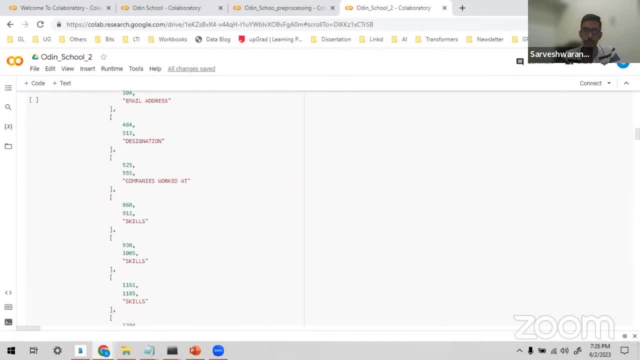 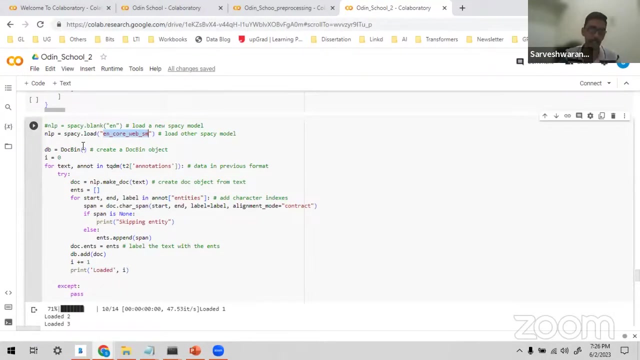 You know the collecting the training data is one of the most time consuming and the complex thing here. So once we have collected the data. so again I use the Encore Web, I use a custom based, custom NER, So I use some dogman format, empty dogman. 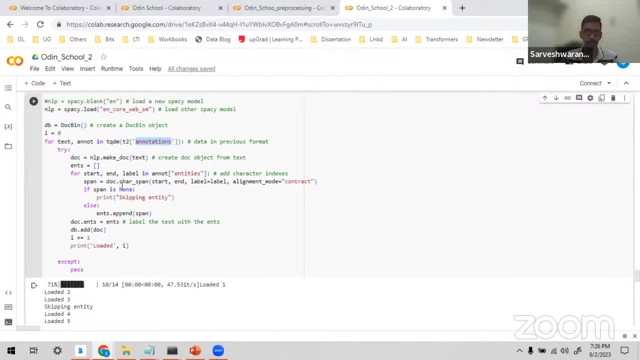 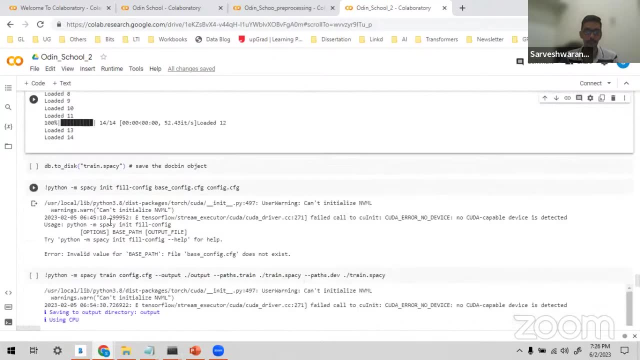 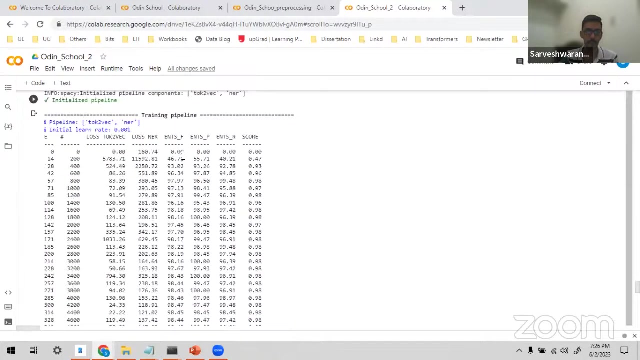 And I take the training data, I take all the annotations from the text And I do the entities. I extract the entities, okay, and you can see the pipeline builds. It takes some time. This has taken a lot of time here. 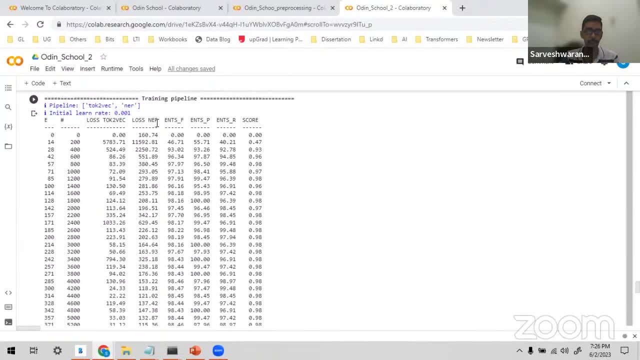 So, while you can see, in every epochs, these are all the epochs, each time for epochs, So for every epochs, and I've given the initial learning rate of 0.01.. So, what is the F1? What is the precision for each and every entity that is improving? 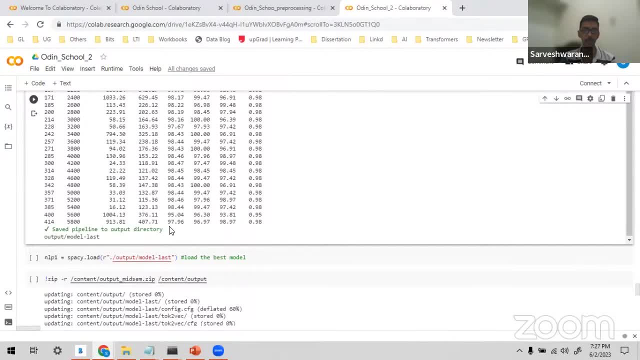 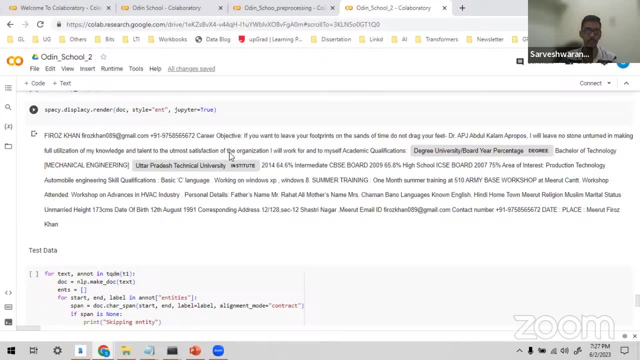 You can see the precision has improved, F1 score has improved and I have saved that model. Maybe instead of that, I can go here right, So this is resume. You can see that whatever I extracted, the degree, the institute name, all these are 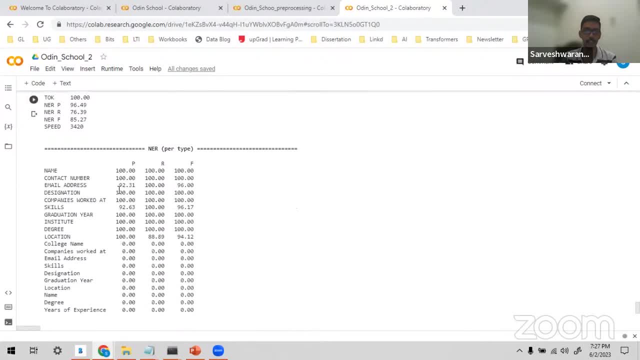 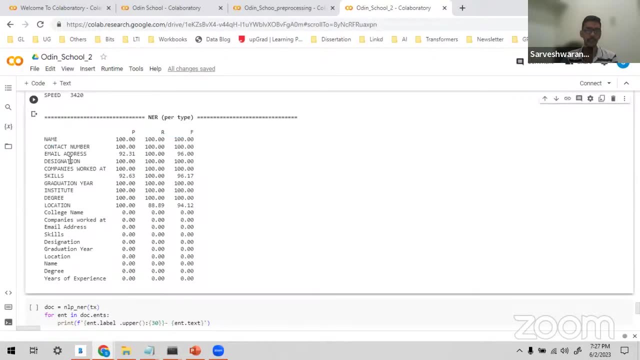 extracted right Again. I have the text data and you can see and I've evaluated the model right. So in that you can see that, You can see that, Okay. So what are the entities that I have extracted? the name, the contact number, what is the? 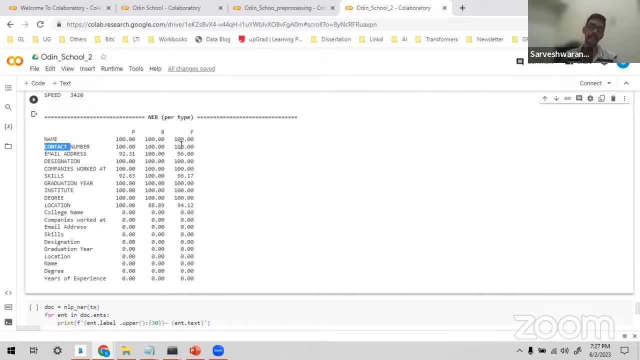 precision recall F1 score for the test data that I have passed. The one thing interesting, the challenges that I have faced was these were some entities that were in low case and it was in smaller case right. All this again to be pre-processed and I have a different working file. 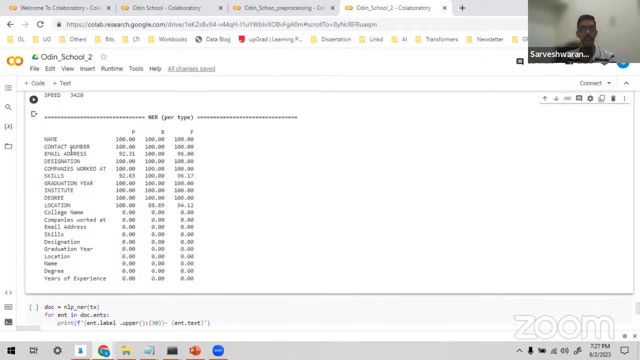 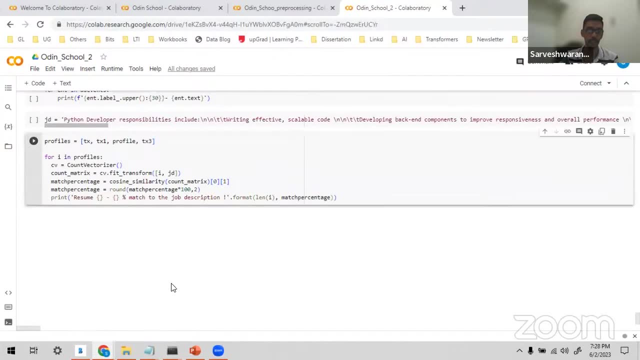 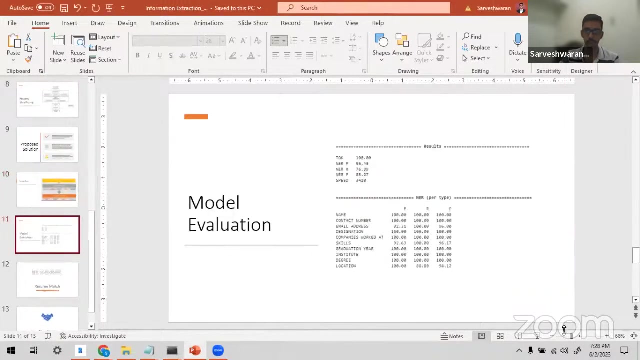 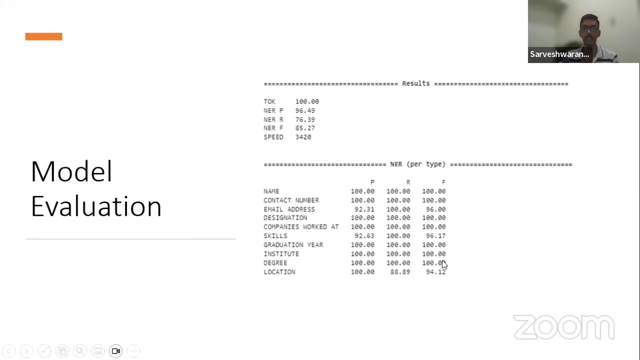 This is just for demo. The application in a lower case makes an impact, right. And then we have done a lot of processing and have used in count vectorizer. and coming here, Let me quickly, yeah, So what the model has, the final model has given us right. 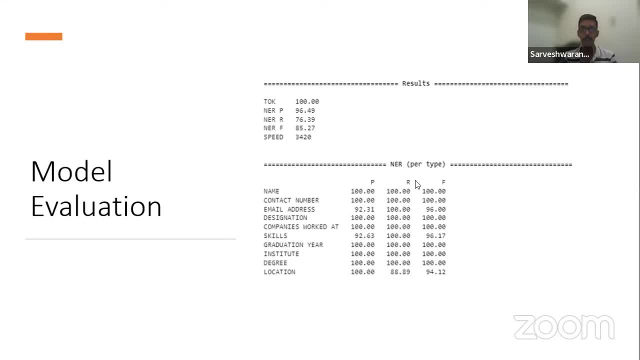 So what were? the F1 score? So the F1 score is the model that was evaluated right. So this was the first step And then later we have achieved that is again in different systems. We have achieved an with the, or a hundred and 150 resumes. 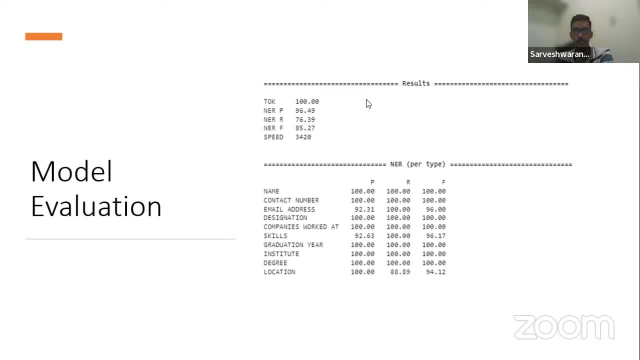 So we have achieved an F1 score of close to 95%, Right, So I was not able to get that, but by doing the same process here. in this example it was 85. So by retraining and doing some hyperparameters. 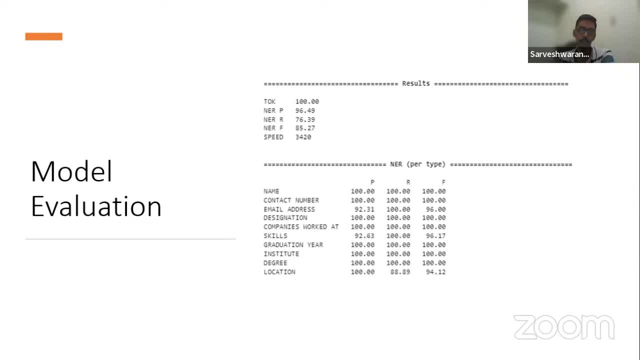 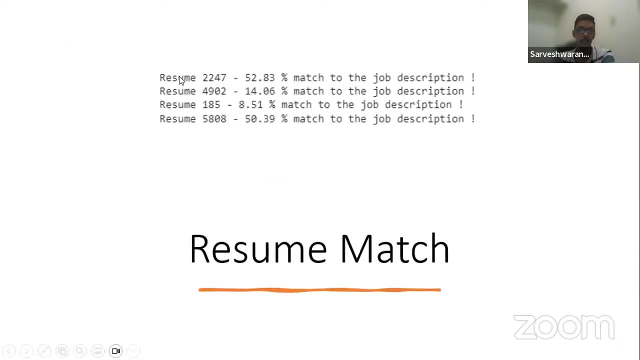 So let us go back to the table. Okay, hyper parameter during. so we were able to closely reach to 95 and this was- uh, this was how- my final. so for each and every resumes, i can see the percentage match and i can rank, order the. 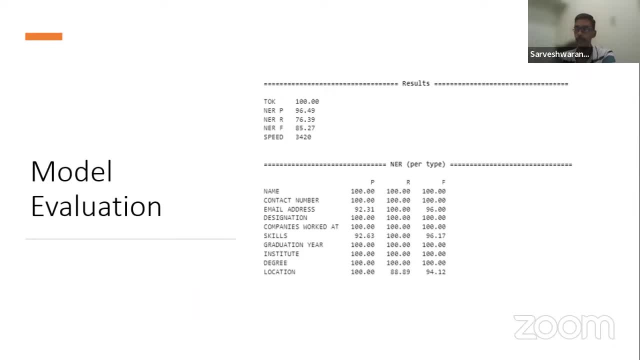 resumes right- rank one. surveys resume: rank one: right. so if i have hundred different resumes for one job position, i can uh rank order the resume. so at least it gives my manager to start with the screening process right, instead of taking something at random, he can have an informed. 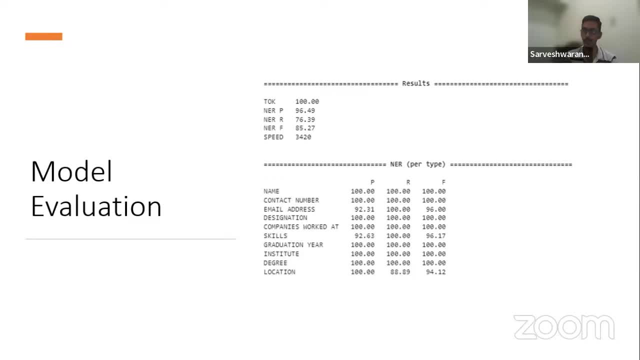 decision. instead of taking from the 100 different resumes going randomly, i'll go in this order which has the rank one to rank. if this is not uh found fit, then right, i'm giving a hierarchy, i'm giving a rank for my managers on the hr professionals to look. 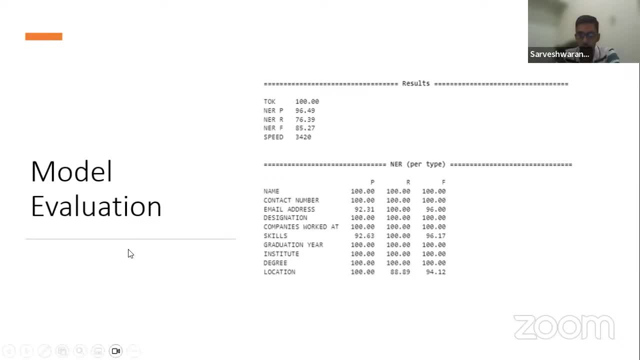 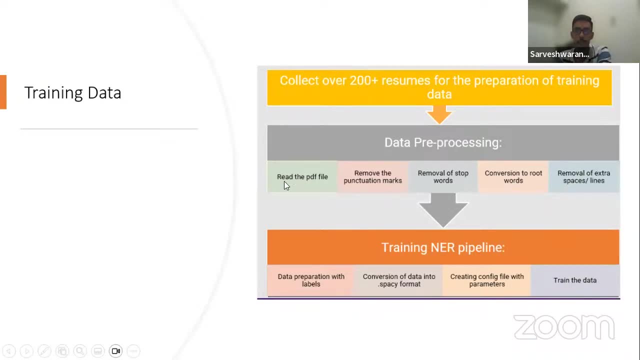 and make an informed decision. right? so, uh, this is one example where you can see that this is how the model is used. right? so this is again. we have collected over 200 resumes. right, some data. pre-processing: remove the punctuation. remove the stopwatch. conversion to the root works. the conversion of root works is called the lemmatization of stemming. 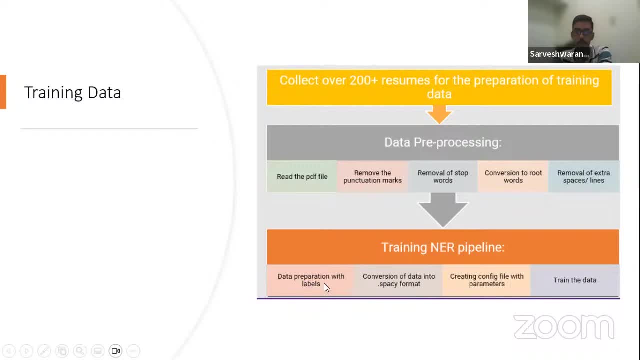 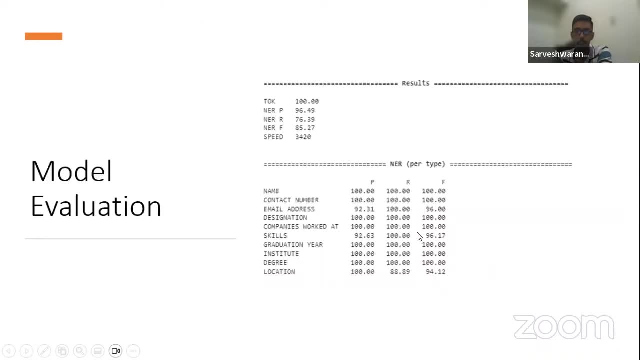 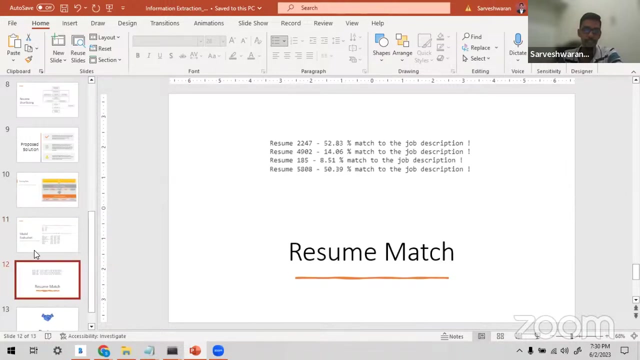 removing the extra space characters. so in the training in-ear pipeline, like it should be, the data preparation, conversion to the specie format, creating the concept file in the training, right so, uh, this is how the model is evaluated and this is for that we have achieved, right so, some real-time application. i'm trying to remember, right so? 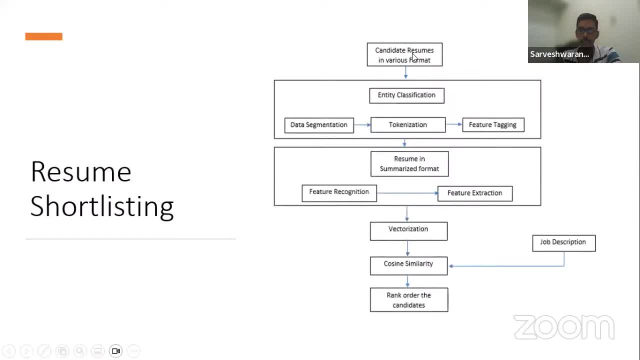 so at a high level. so so candidate resumes in various different formats. i do the entity classification, data segmentation, the tokenization and the feature tagging. i convert the resume in the summarized format, like i showed you in the json format, and i do the feature recognition, feature extraction and i vectorize it. 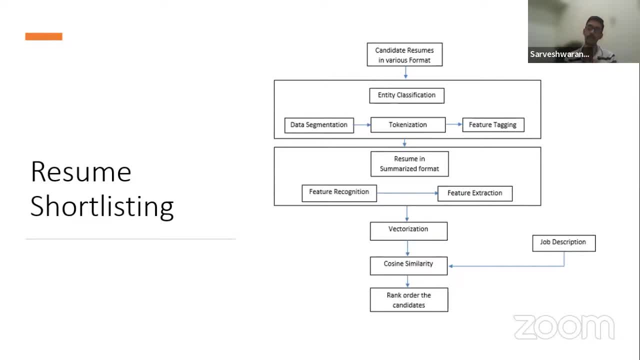 so you know what the vectorization, the pfi, the term frequency, will document vectorization and using cosine similarity, the job description is here and uh, the vectorized. uh, okay, the job description again should be vectorized. okay, this arabic should be here. uh, that's a mistake. 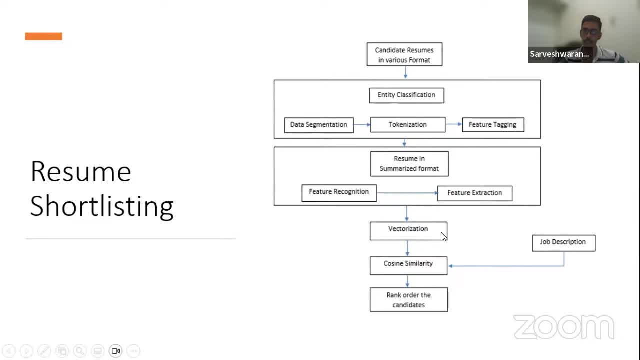 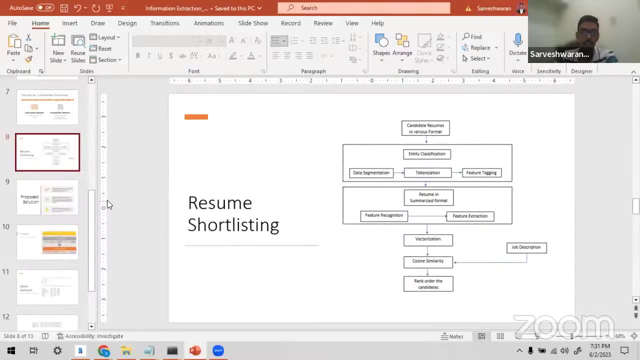 so this is one vectorized format and the job description is also vectorized. i use a cosine similarity match to find the match between these two and i rank order all the scanned days. This was a fantastic use case that we have achieved using this in the real-time use case. 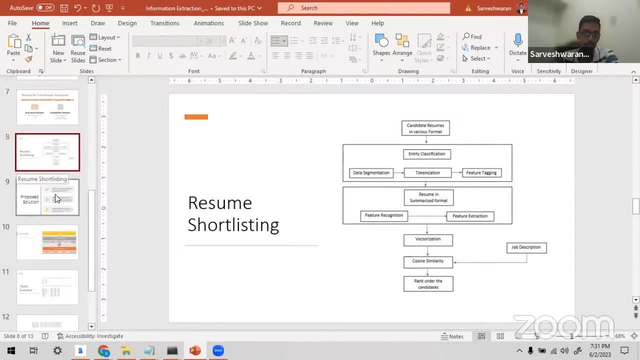 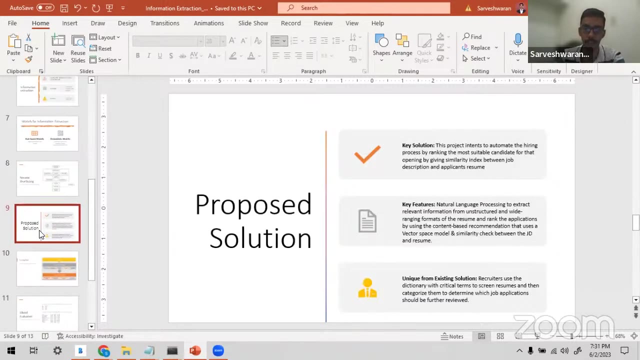 where we have achieved and we are using it in. so this is one area where we have achieved. So I'm just taking a pause or a break. do we have any questions? So this is what which I had planned for this session. so do we have any questions? 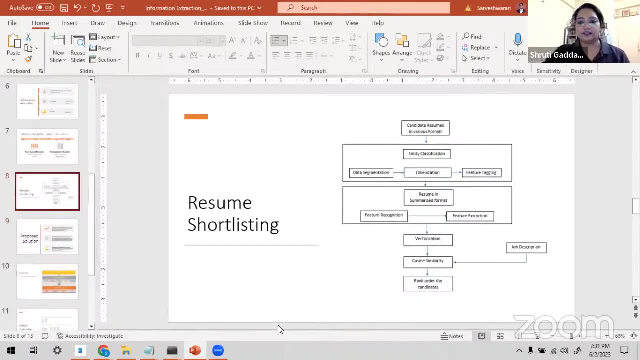 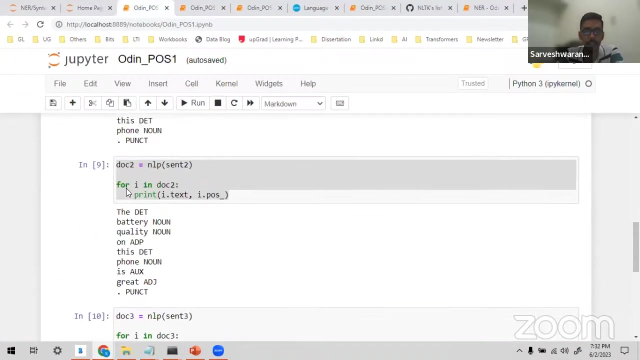 Yes, so we do have a few questions. probably give it 5-10 minutes. so first, one of the first questions is: could you talk a little about tokenization? what is tokenization? could you repeat that please? Okay, tokenization. let me quickly see if I haven't filed. so the tokenization is nothing but simple words. 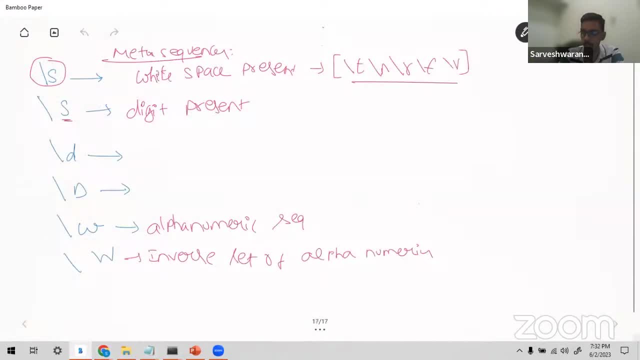 okay, what I'll do is I'll write it here. So today is a good day, today is a pleasant day, right? so this is the string. so this is the string saving it inside an object if it is in tokenized format. 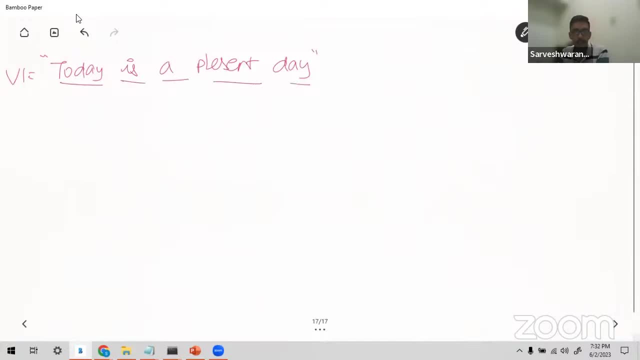 I break down in sentence into every single word. if I'm breaking it into every single word, it's called as a word tokenization. Today is a pleasant day, So every word in a sentence is being tokenized, right? So every word in a sentence is being tokenized, right. 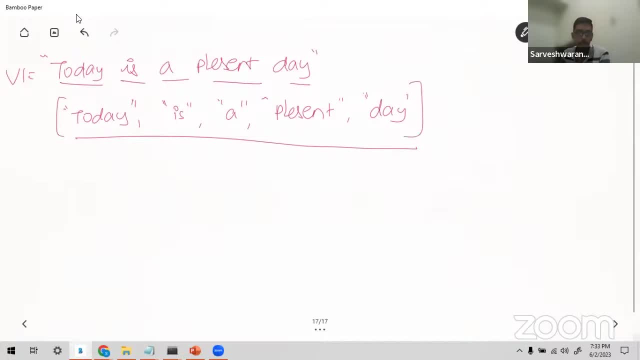 so it is again it is. it's separated, it's split into and separate words. that's what you call as a tokenization. tokenization can be a the sentence tokenization, the paragraph tokenization- right, so this is how sentence simple string is being tokenized. 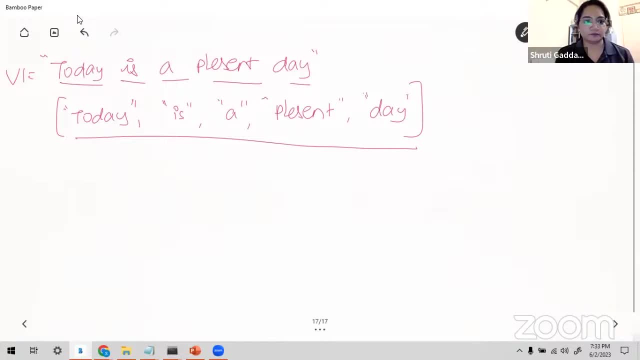 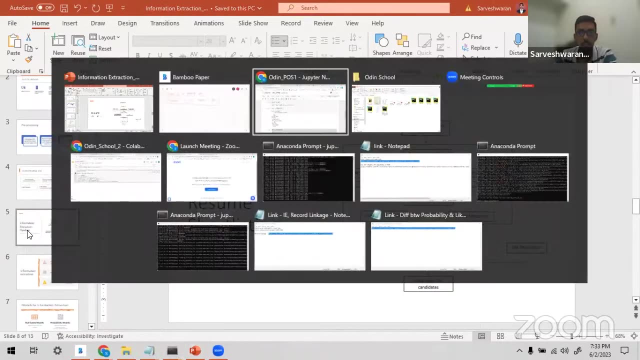 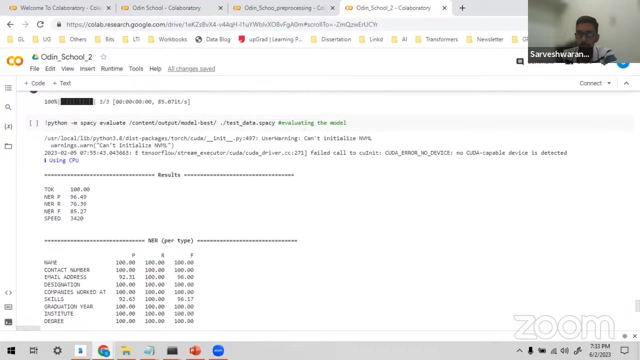 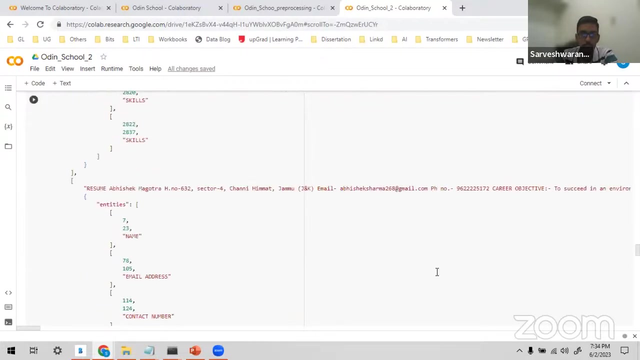 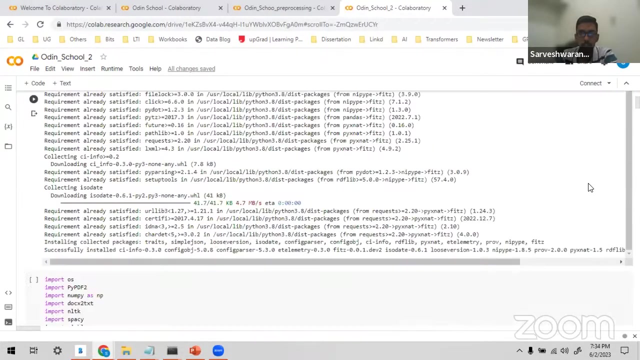 Great, what is JSON format? Okay, oh okay, the what is in JSON? JSON format is a semi-structured format. you can see here, let's go up. so it has an JSON, has a key value pairs. 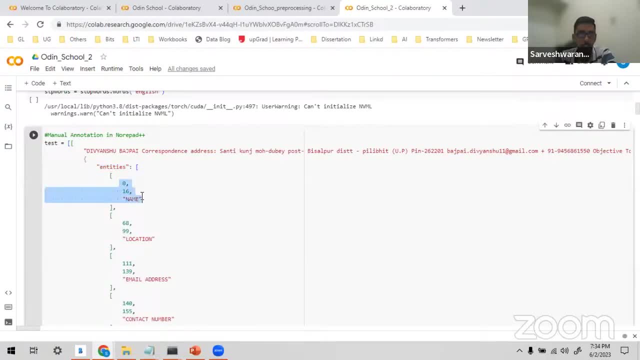 right for the word entity. right for the word entity. value is 0,, 16, and 0,. JSON is a key value pair. it's a semi-structured data. it's not a structured, it's a semi-structured data. 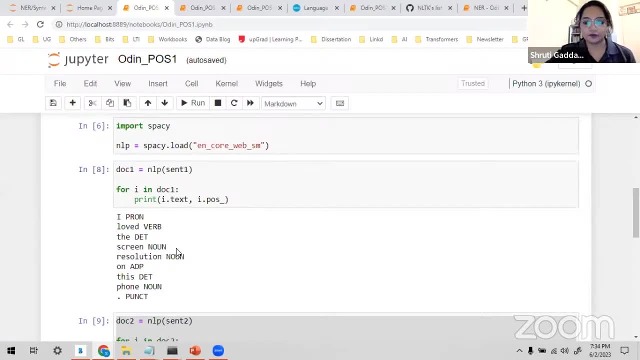 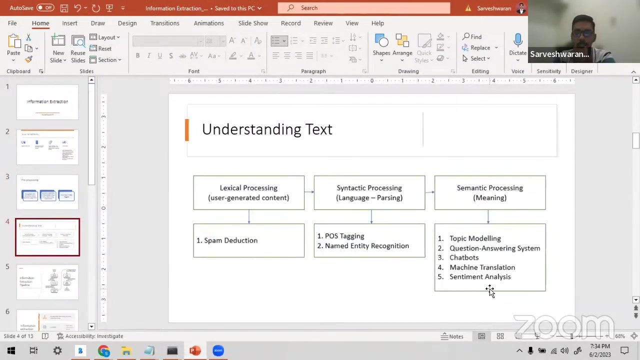 Right, there are a few more questions on a little more about speech tagging. I mean a lot of your talk was around it. could you like summarize it For the speech tagging? you mean POH tagging, Part of speech tagging, I think. 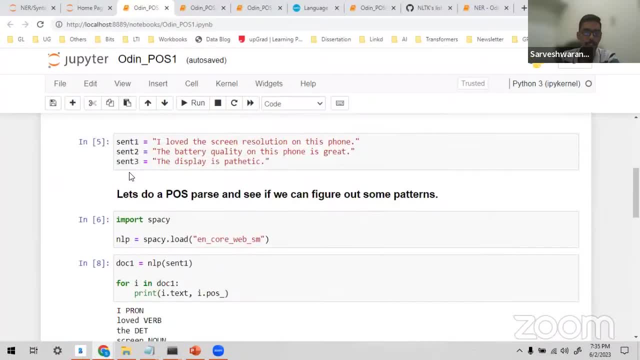 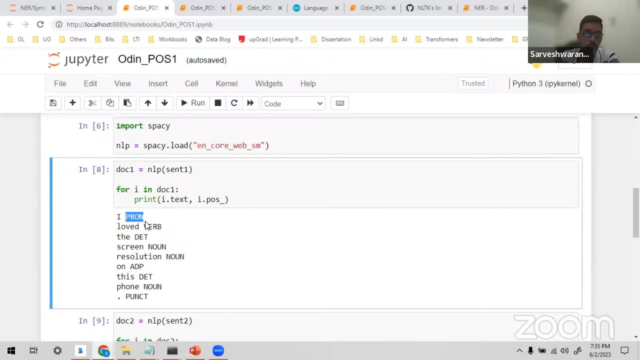 speech tagging- part of speech. yeah, yeah, so the part of speech. tagging is, again, this is what we were saying. so every word, the tokenized word, I'm tagging to what is the grammatical sense? part of speech. what is the part of speech? 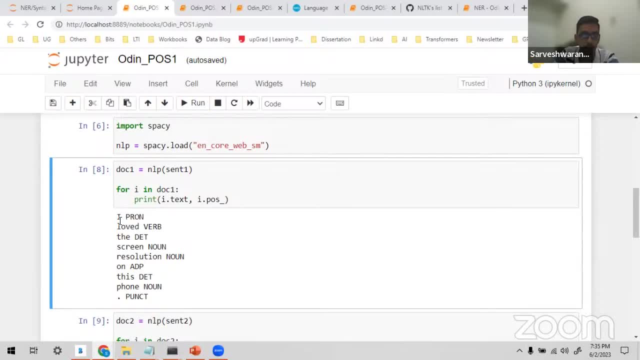 speech like we learnt in the high school. What is that? I mean It's a proper noun. Loud mean it's a verb In a sentence. what is that? each and every word represents? The is a determiner, Screen is a noun, Resolution is a noun. So what is that in a sentence? What is that part? 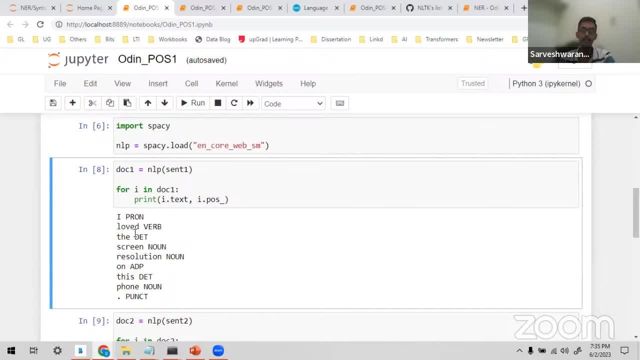 of speech tag. What is the grammatical sense of that word in that sentence? That is what the part of speech tag is Right. Another very interesting question: Is there all these capabilities that NLP has? Is there an alternative to this? Is there an alternate technology? 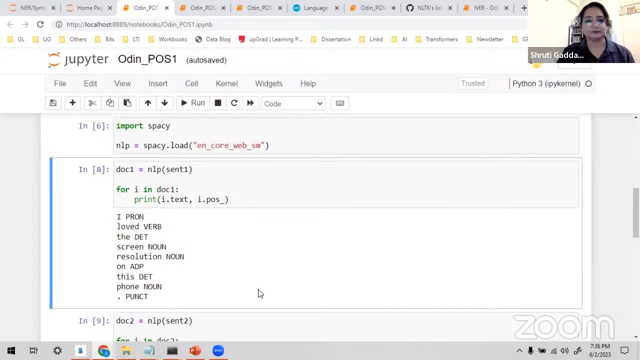 that gives this kind of results. That's why I used to critique: Okay, So alternative, see. so these are the basic fundamentals. How do you process this text If you do not want to process all this text? nowadays, there are a lot of open AIs from. 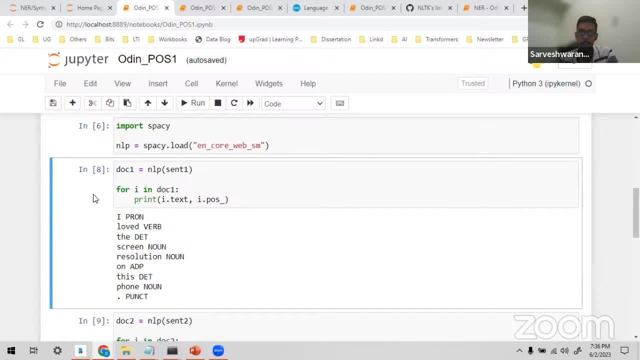 the hacking phases available. So the Gen A is making a revolution recently. So we can make use of the Gen A, You can upload a document and you can extract the entity right away Because, like an N-core web that I'm using here, they're using GPT models within the 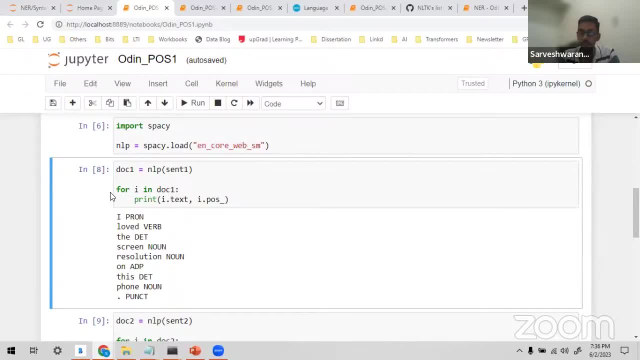 data that they are using. So if you're looking for an alternative for all this process, you can use maybe an pre-trained model. There are various different pre-trained models, So here what we have used is from spaCy and encoder. You can use an NGPT 3.5, GPT 4 models. 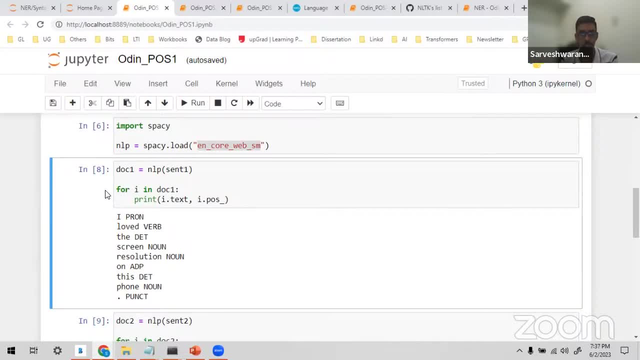 and you can look at, as an alternative for all this process, the pre-processing steps. Right, Okay, Another question. This will be the last question After this we will conclude. So all this NLP concepts that we're discussing, and I must tell you it is a very, very clear. 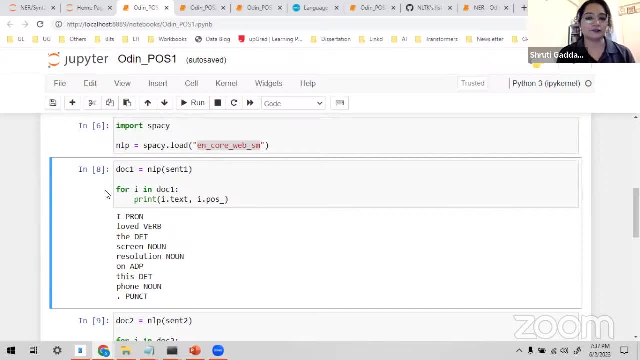 crisp kind of masterclass on the fundamentals of NLP. A non-technical person like me also could understand a great part of it. So the question is: where does data science come in all this process, come into in all this process? Okay, See, the word data science is a very 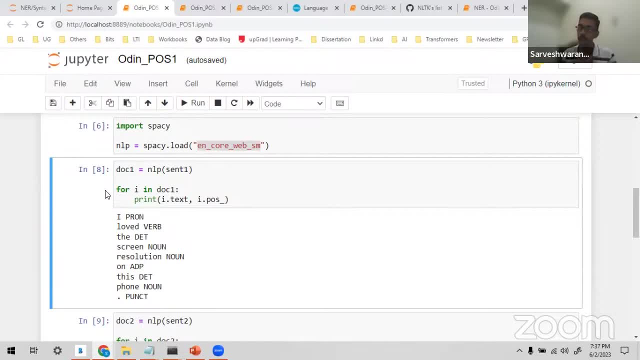 huge topic, right. So when you use in machine learning, deep learning, right, And text processing, the image processing, video processing. So when you do an analytics, when you do some analytics and when you do an algorithm, machine learning algorithm- or in deep learning neural. 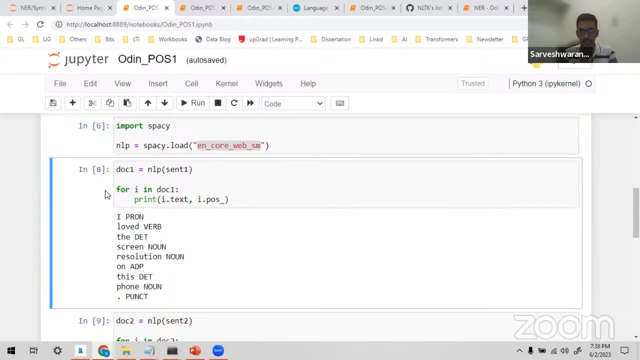 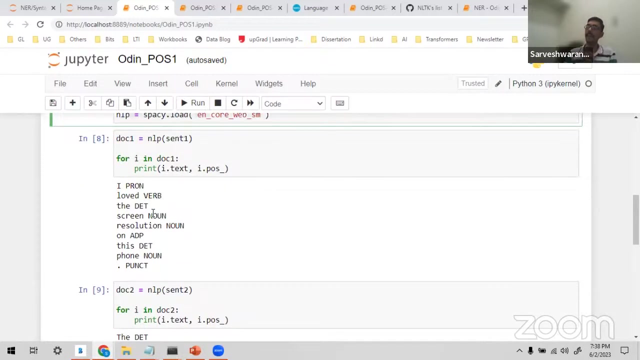 networks. it means that you're touch basing on in data science, right? So the N-core web is an pre-trained model. It's a pre-trained transformer based model. I'm making use of this model and I'm doing some processing, So the data science is again. 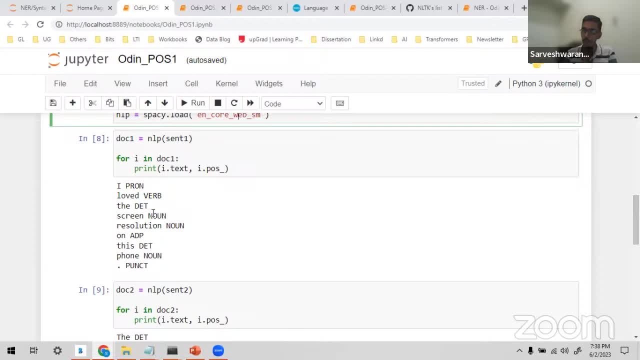 when you deal something with data, right. So when you want to look for an informed decision from the data, you call it as in data sensors, You would do basic data analytics, do an hypothesis testing, or you do an sentiment analysis or the chatbot. 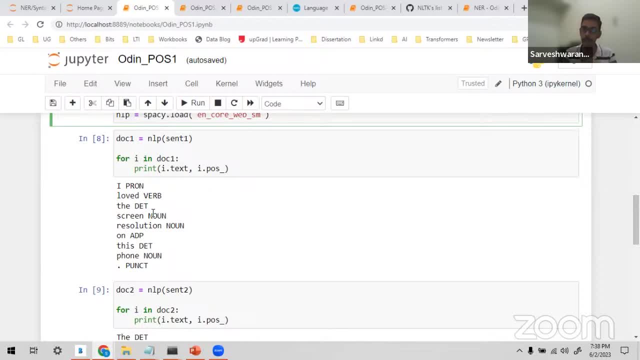 Okay, Right, Okay, and chatbot, or you do an image processing, or in video analytics, or image video processing- right? so all this comes under the scope of an data. you have some data and you're making some informed decisions from the data. that's where the data sensors fall into. that's where you call all. 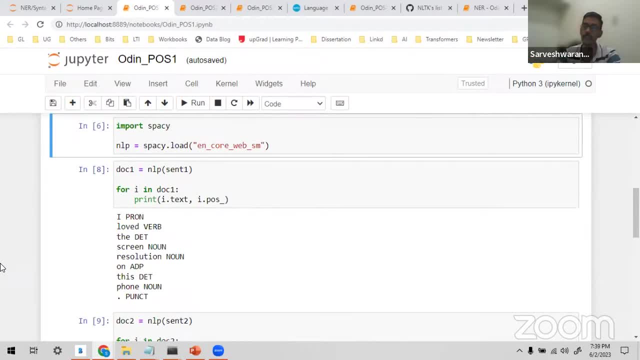 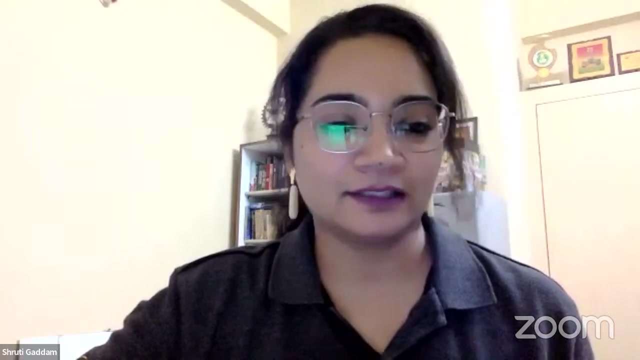 this as some data sensors. so under the data science, one of the branches is the natural image operations right. thank you, Zereshna, thank you so much for spending this one really, really exciting hour. i'm sure there was a lot of learnings for all our audience today. so, yes, this, this is being